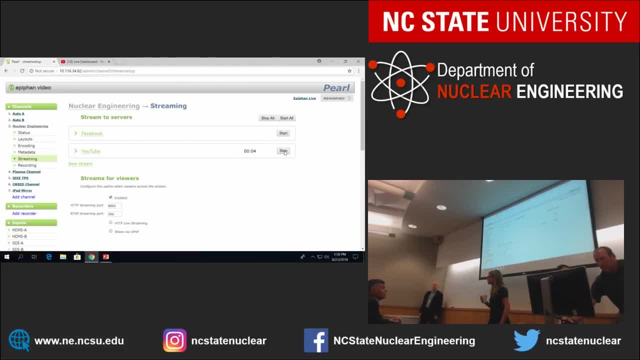 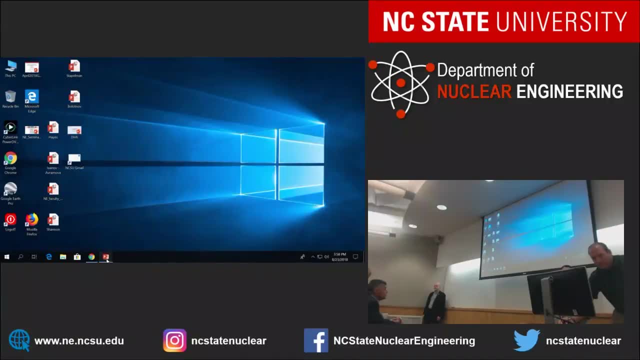 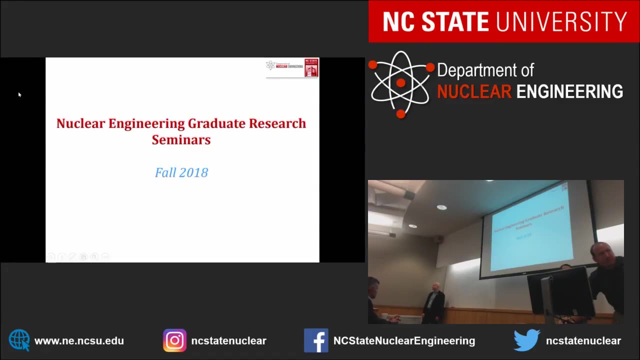 Thank you for watching, So we should be staying here, Okay. Okay, may I have your attention? Let's get started, because we have a lot of slides, So you may have to stay a little bit longer. So, with that said, first of all, I would like to welcome the new students. 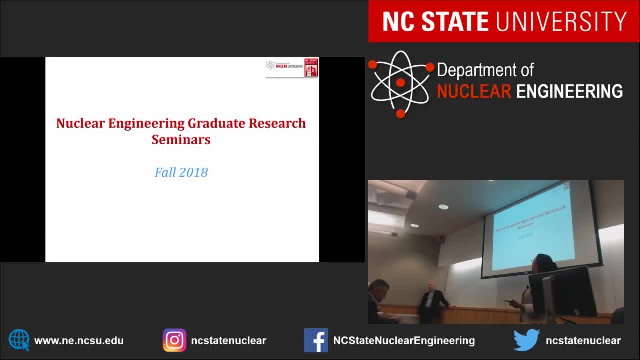 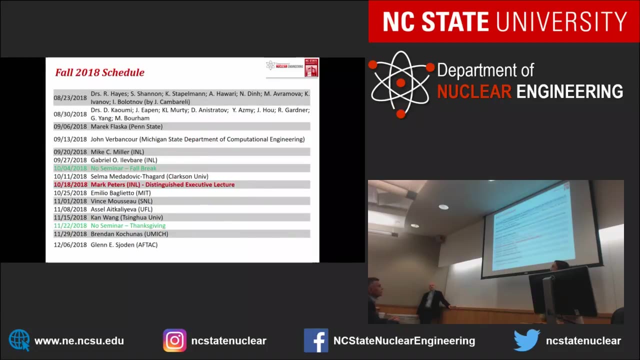 and welcome back the old students or the NC State students. I'm the faculty responsible for the seminar this year, So if you don't know me, my name is Maria Vramova. I'm associate professor here And before we start, I just want to show you the schedule for the seminar this semester. 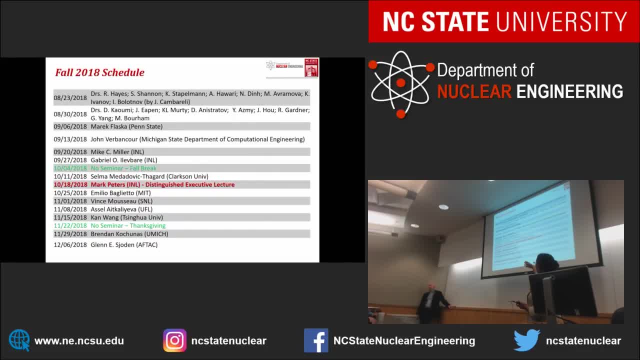 As you can see, it's full And we won't have one for the Thanksgiving and the fall break- Just to point your attention- and distinguish executive lectures which will be given by the director of Idaho National Lab. And you can see we have a variety of different areas. 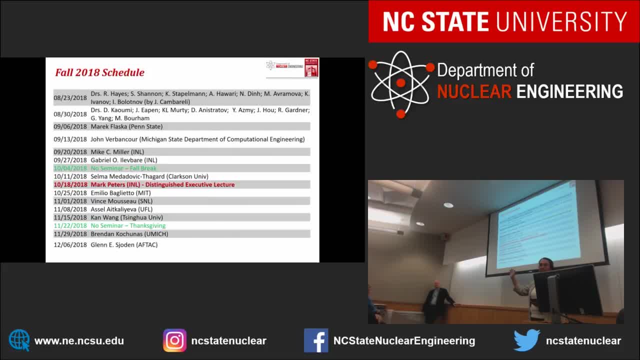 Probably you don't know the people, but I can tell you it's plasma, thermo, hydraulic reactor physics. good variety Now. the first two are for your professors here at NC State, So we'll have lecture. well, highlights of their research, or our research, today and next Thursday. 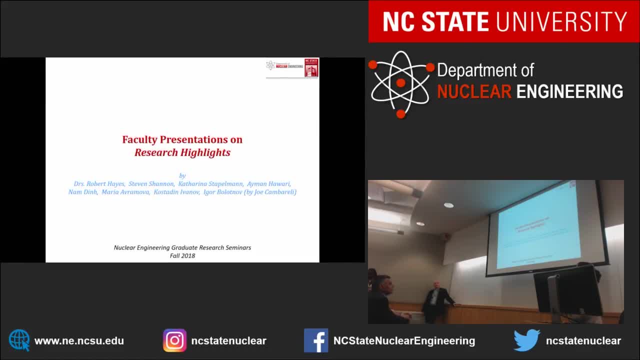 And we'll start in this order, starting with the first one. So we'll start with the first one, So we'll talk with Dr Heiss, All right, So I have a question for everybody When I talk about what I do. 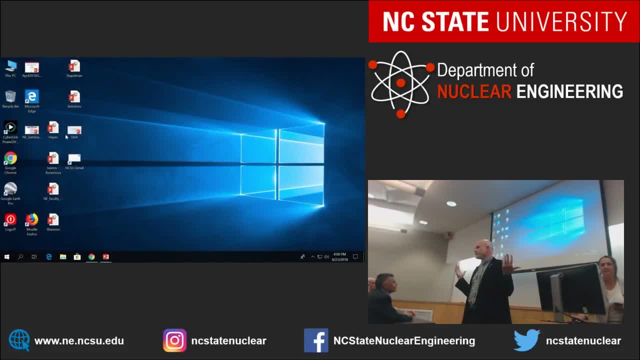 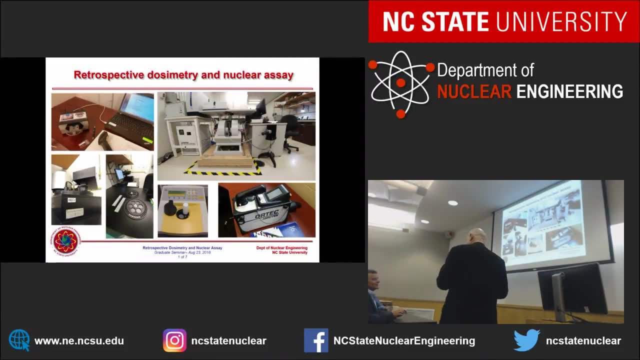 I'd like to start off. who does not know what a gamma-ray spectrometer is? Everybody knows what a gamma-ray spectrometer is, right. Hopefully You could do that one. Everybody knows what a gamma-ray spectrometer, okay. So it's. it's technology that's used to measure the spectrum from a radioactive source of some kinds. 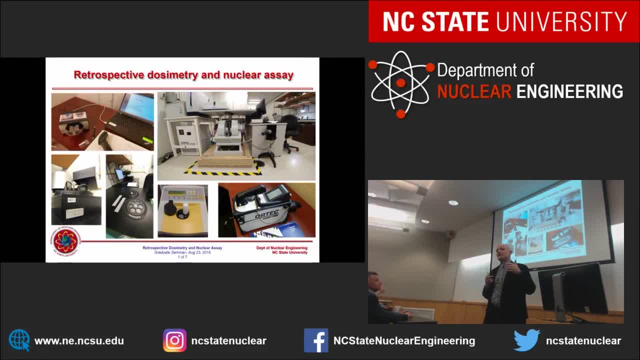 For ionizing radiation. we measure the energy distribution that's emitted. so the research that i do, uh, this is a that does something very special. i'm gonna- i'm gonna- introduce it by asking a question: how many of you would believe me if i told you that? 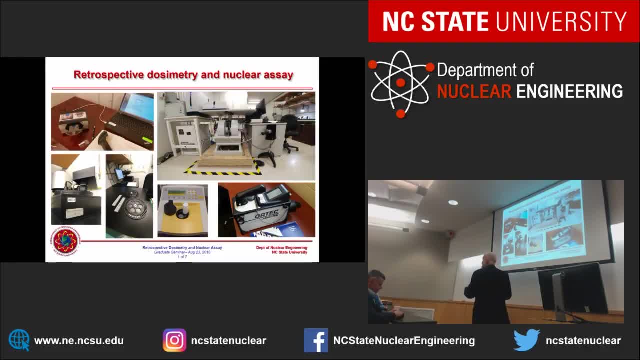 because of the research that i do in my lab. there is right now a gamma-ray spectrometer in your parents bathroom, in their very shower. oh, some of you. so some of you are familiar with what i do. okay, what if i upped the ante? what if i said that there's a an imaging gamma-rayлосьpectrometer? 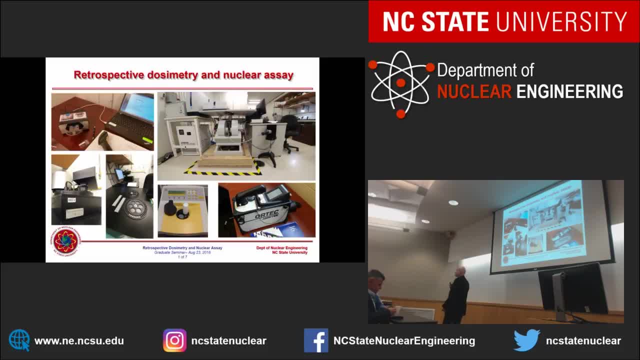 that's in every nuclear facility that the united states does has no idea exists. how many of you would believe that? none of you. oh, oh, then you're okay, you know me all right, so so that makes it fun. if nobody believes that, then i get to prove that and prove to you that what i do in my lab is impossible. 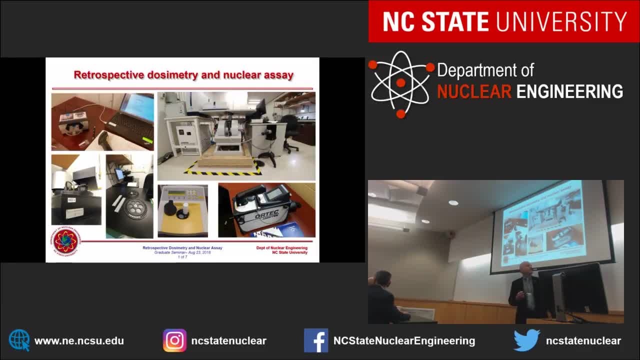 so that's what i like to do. i like to do the impossible. I like to do that for lunch. so here's some of the instrumentation that we have. what I do is up in this one, right up in here. this instrument right here. it does magnetic resonance. here's a traditional portable. 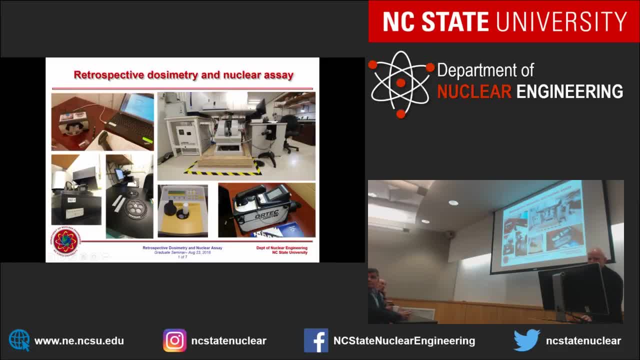 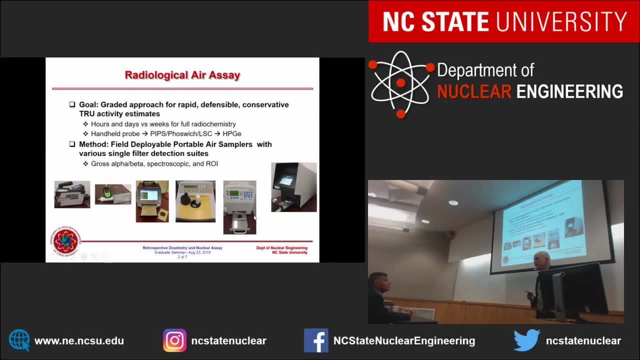 gamma-ray spectrometer, liquid scintillation. this instrument over here does thermal luminescence and optically stimulated luminescence and this system here is a medical physics dosimetry system for measuring entrance dose to patients for medical physics. I also do air monitoring. I do a lot of impossible. 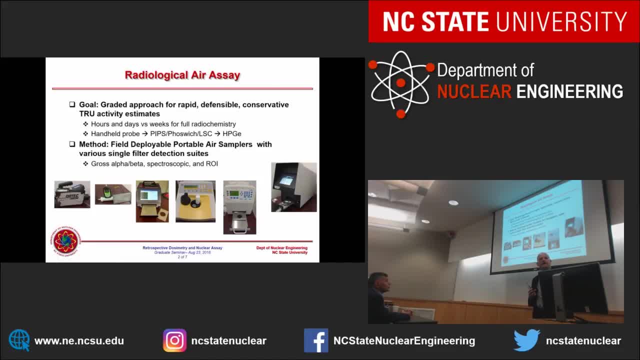 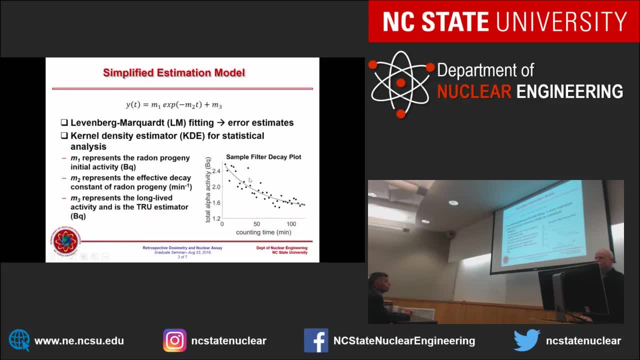 things with their monitoring. I love to tell you more about it, but there isn't time to go over the detail other than to instead- and that's, if you look here, this is an air filter and just measuring the radio, the radioactive decay on the filter, what I have up here in equations into the simple equation, a single. 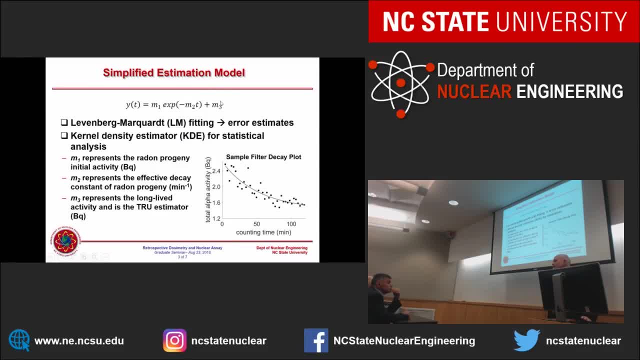 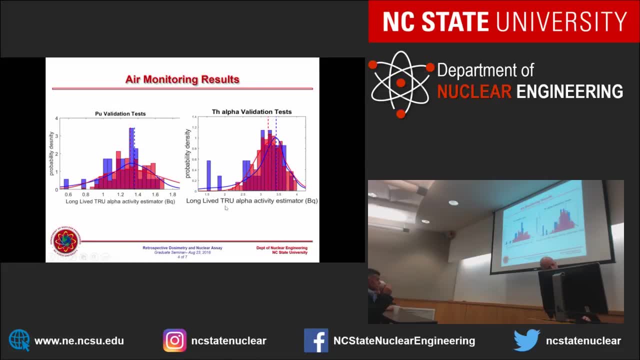 exponential decay so that asymptotically it approaches a constant. that constant is an estimate of the anthropogenic content in the filter. the student was able to do some really cool stuff showing that it works. it works great, it works amazing. one of the fun things that that came out of his research was using kernel density. 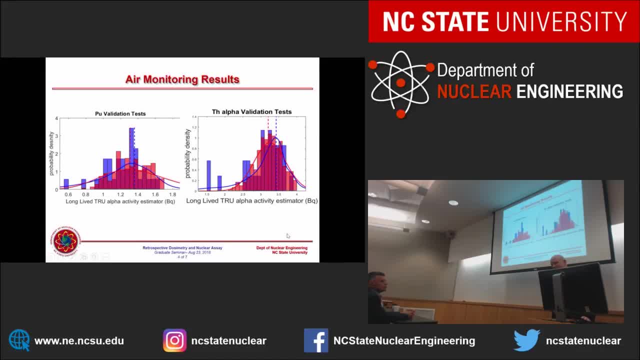 estimators. what that is is, when you histogram data, you're throwing away some of the information, and the reason why is because when you've histogram the data, you're assuming that the uncertainty in the data is folded into the distribution that you get from the histogram. but what ends up happening is that in any bin, the data that was in that bin 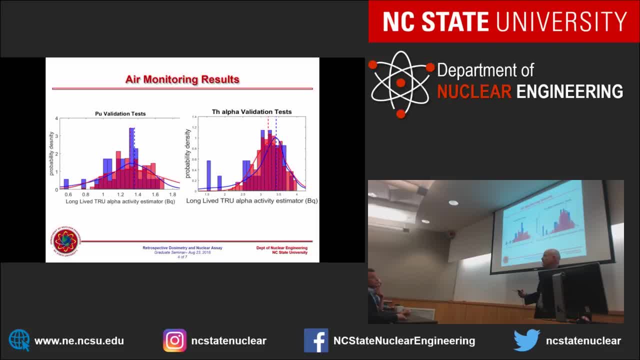 could be in a bin above or two bins below, depending on the uncertainty of that value that you histogram. you're basically throwing that away and you're assuming that that's getting folded in the distribution. by knowing the uncertainty of each of the measurements that the student did, who's able to? 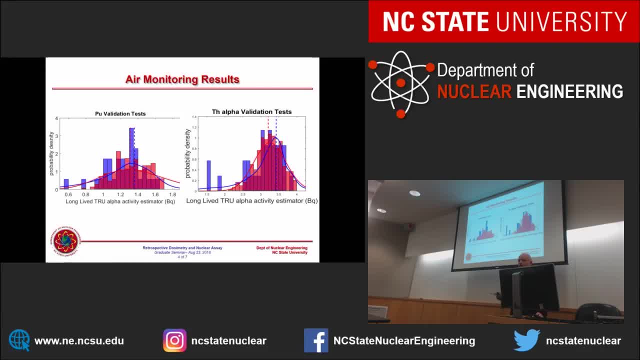 effectively model. each one of them is a Gaussian and then you just add up all the Gaussians and you get these cumulative distribution functions- cumulative distribution or these probability density functions over here, the blue and the red. The blue is when you actually had activity on the filter. 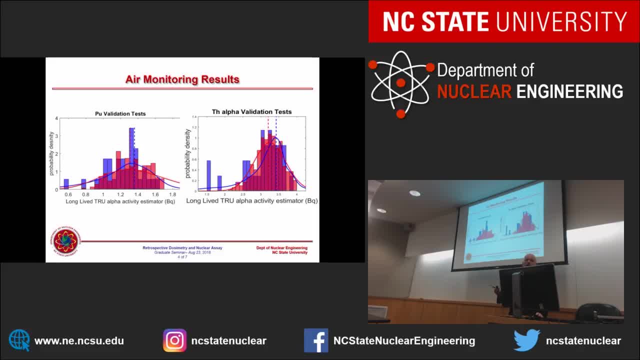 The red is when you had the no activity And you're comparing how well it was able to predict the actual values in Becquerel's And he was able to show that it's always conservative 95% confidence level. This method that I showed here does. 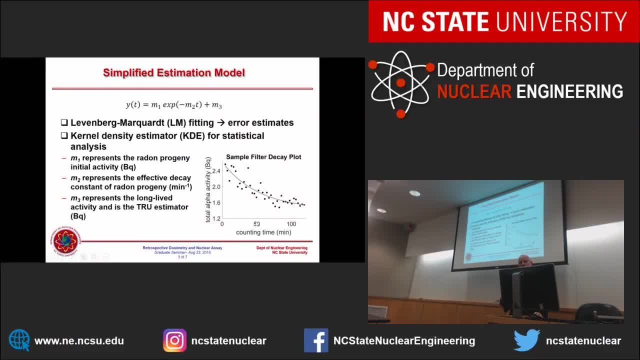 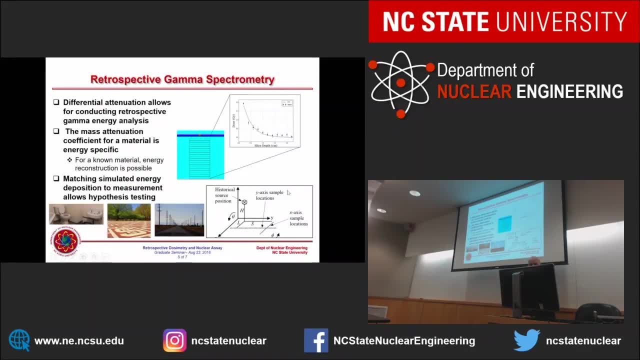 be conservative if you fold in the uncertainties. And that was done by fitting this data with 11 Bergmark Park, Not to my impossible claim that I get to prove to everybody in the last two minutes. So what I do is thermoluminescence. 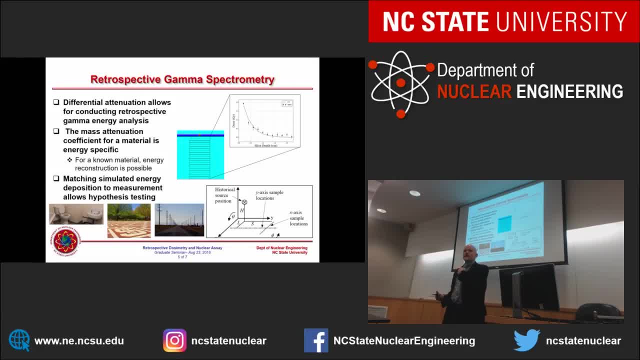 It's the same stuff we use for our radiation worker dosimetry badges. In a thermoluminescence badge we have crystals. You heat. It gives off light that's proportional to dose. If you're doing OSL like we do at our lab or here at State. 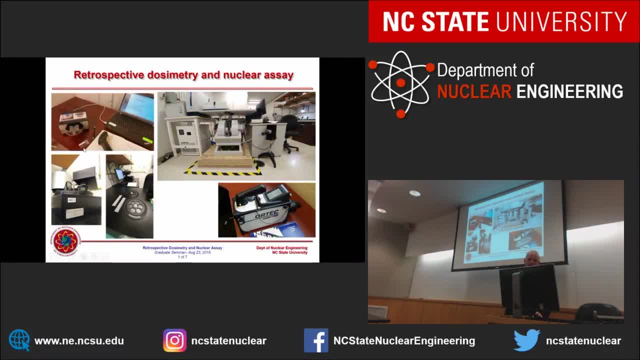 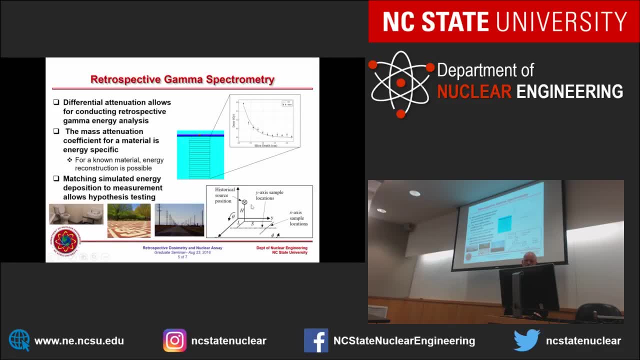 you're shining light on it And it gives off what this system does. This is an OSL. This one also does OSL and thermoluminescence, But if I were to do this, I would be able to take a grid if I had a source here. 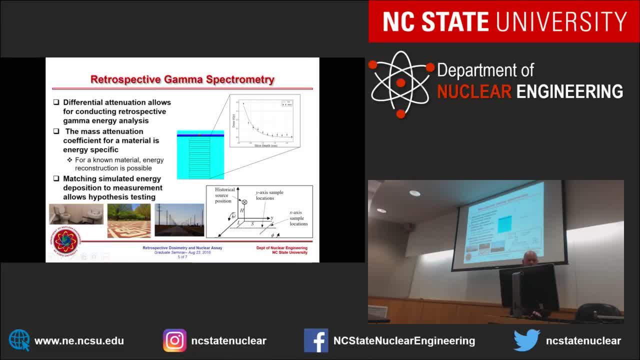 and I were able to take a grid of material. Oh, let me back up. So what I'm able to do is I'm able to take any kind of an inorganic insulator and turn it into a dosimeter. So if I take an array of bricks and I 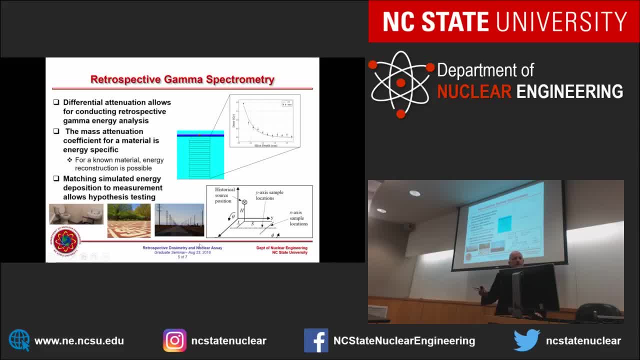 were to sample along these bricks and measure the thermoluminescence that's given off and it pours from that brick. based on inverse square from the array distribution, I can image the source So using any kind of a like this wall right here. 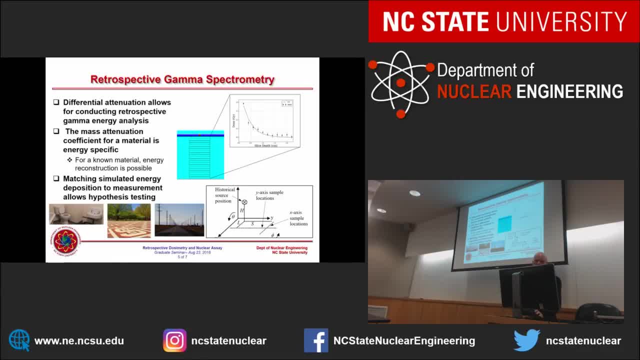 would work. Any kind of an inorganic insulator then becomes a gamma camera. So there are now gamma cameras everywhere because you have inorganic, basically building materials, everywhere. If you then do a core- my student was able to show- you do a core and then you do slices. 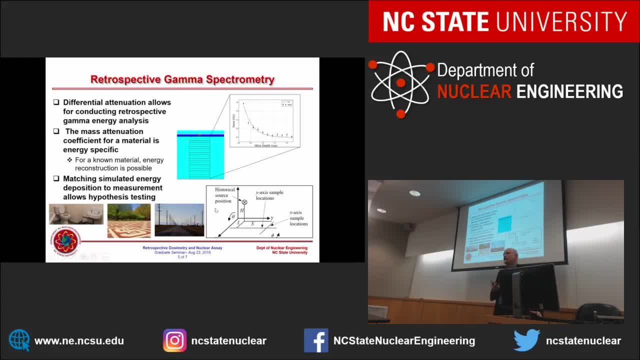 and then you measure the dose deposition profile. what that tells you is the mass energy absorption coefficient distribution of the radiation source that it was exposed to. And so by measuring that mass energy absorption coefficient you get the energy. So you can say: Is it a single decaying exponential? 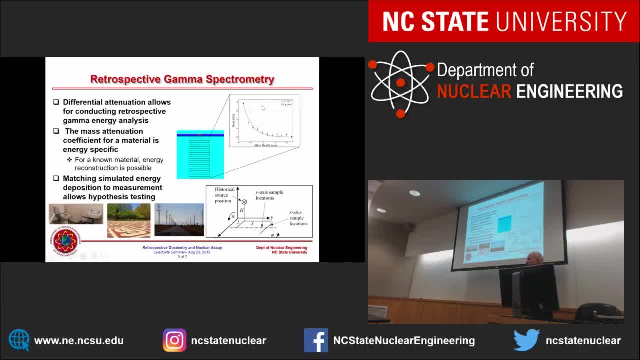 or is it a superposition of multiple, And so unfold what the energy was and therefore the isotopics of the source, And so it just became a gamma spectrometer. So there is as long as I can claim that these unknown nuclear facilities to the United States. 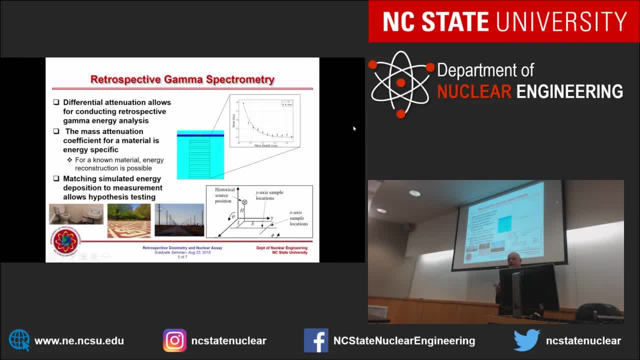 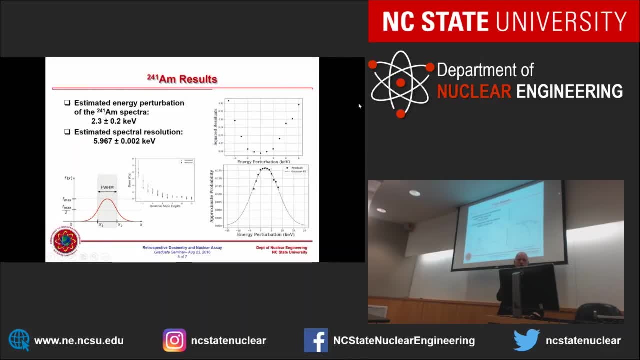 have insulating inorganic material in them. they have these imaging gamma ray spectrometers. So hopefully now you believe that the impossible is possible and we do it here at State On a regular basis. So welcome. And then he was able to show for americium using this technique. 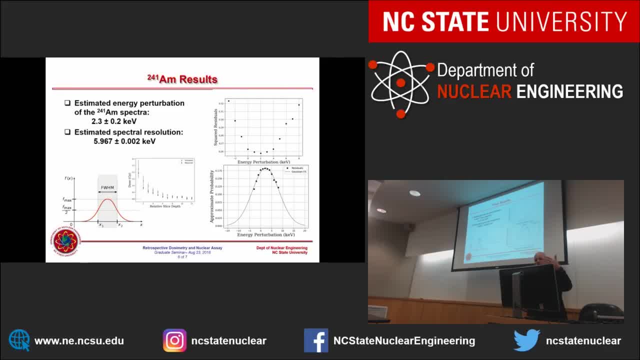 using a perturbation technique and then looking at the sum square of the residuals and how they're distributed, showing for americium that there was only a bias of a few keV with a half maximum of the distribution, showing an energy resolution of about 6 keV, meaning for americium. 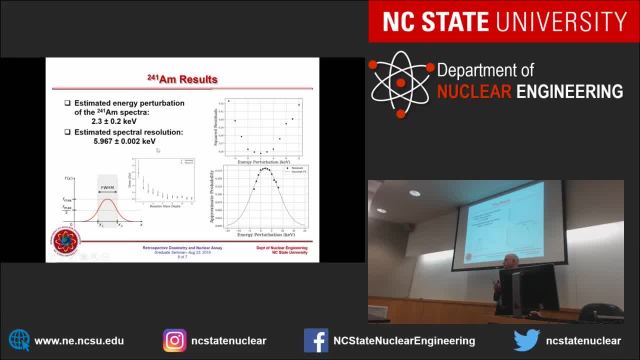 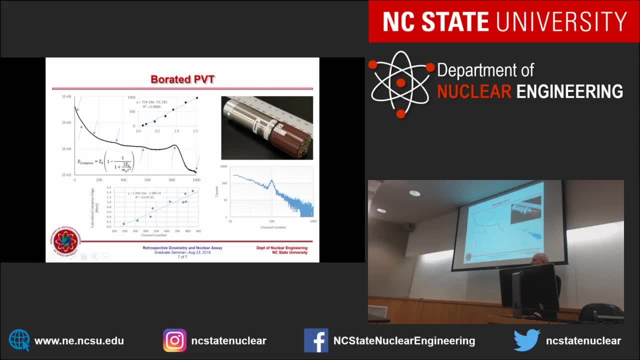 the energy resolution of the spectrometry system is about 10%. So with that I'm done And I've got to go. Oh, and then we're doing some other stuff with detectors. that's just really cool using the Compton Edge. 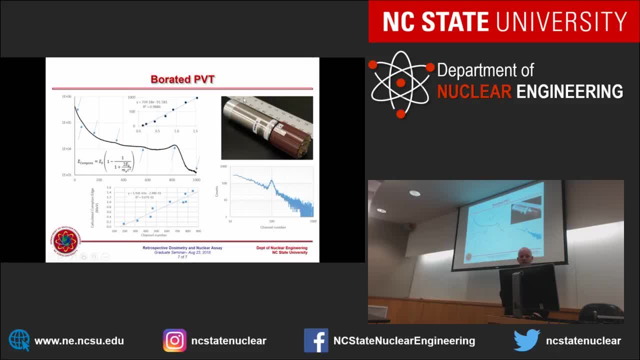 Doing a lot of other stuff. If you came to my lab it'd take a couple hours to go through all the fun stuff. But it's just crazy fun And, like I said yesterday, every one of us think we do the best research and I'm no exception. 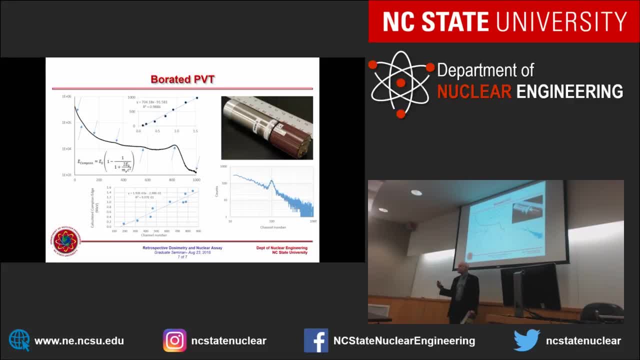 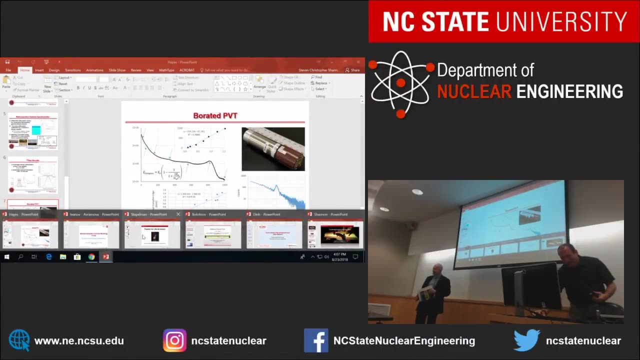 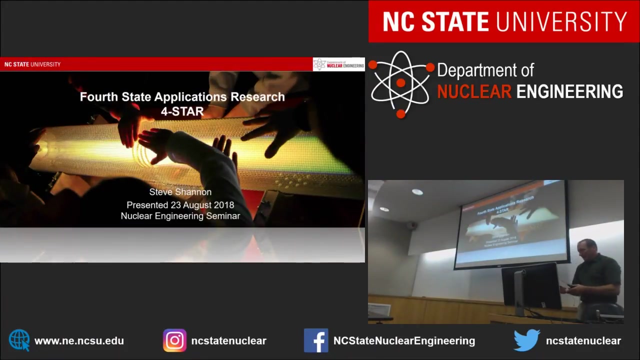 So who's next? Do you want to answer some questions? Oh sure, Any questions? Any questions? No, All right, All right, Let's see again where you picked up. Come to my lab, I'll show you. Hang on. 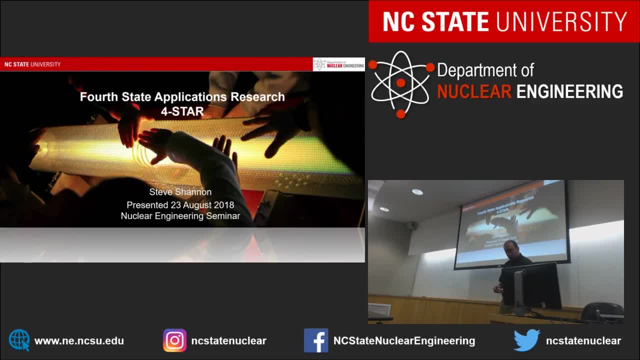 I've got to pretty myself up here. Here we go. All right, My name's Steve Shannon. I'm going to talk a little bit about my awesome research. depending on who you ask, It's the name of our group. It is the Fourth State Applications Research Lab. 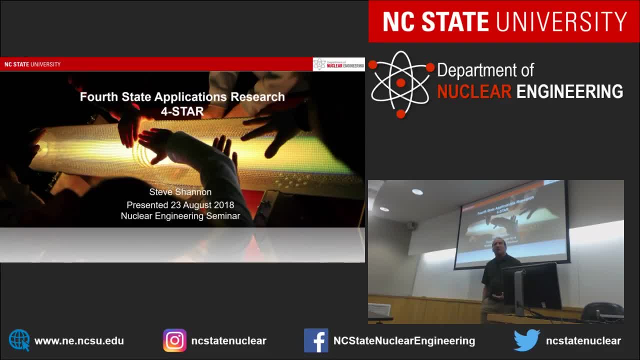 or we call it, we nickname it Four Star. We specialize in plasma science for an array of applications, everywhere from fusion technology to industrial and biological applications. I'm going to talk a little bit about my focus area, And Professor Stapleton is going to talk shortly. 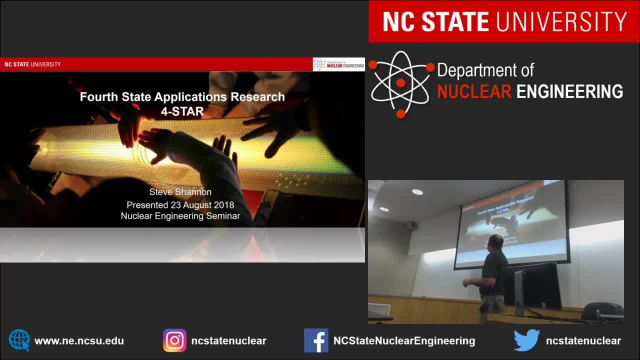 after about her focus area in plasmas for life sciences. This is actually a plasma reactor that was designed by some undergraduates a few years ago as part of the senior design team. It was a portable plasma source that you could take to elementary schools. 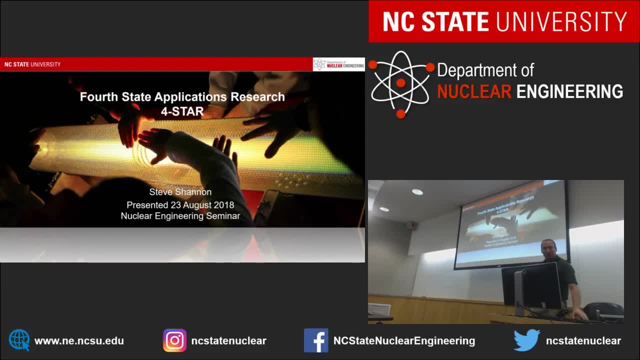 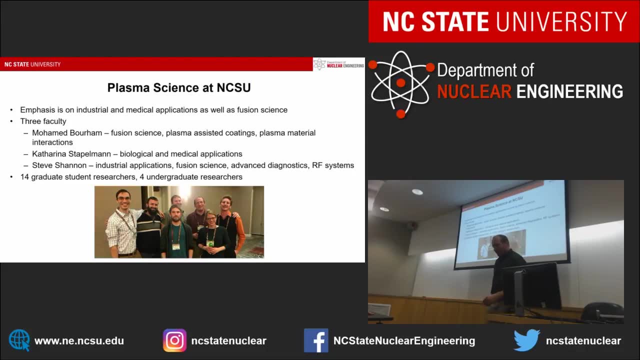 For science days so we could teach kids plasma physics. So those are actual little eight-year-old hands playing with a high-power RF device. So a quick overview of the plasma work we have going on over here. We have three primary faculty: Dr Borum, Dr Stapleton. 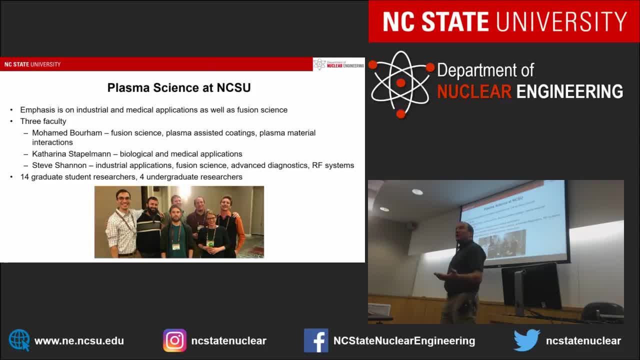 and myself kind of crossing over into a lot of different plasma areas, spanning from fusion energy technology, which is the traditional nuclear engineering plasma application, and also working And industrial applications, biological applications, et cetera. Right now we've got a pretty good group: 14 grad students. 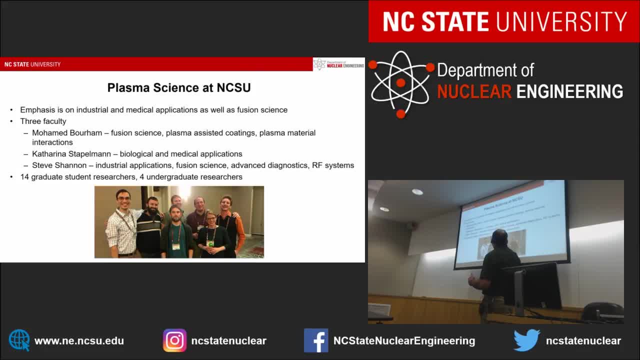 four undergraduate researchers and looking to grow. We couldn't crop all the beer bottles out, but we were able to get rid of the ones the students were holding. But this is a picture of some of us at an international conference last fall out in Pittsburgh. 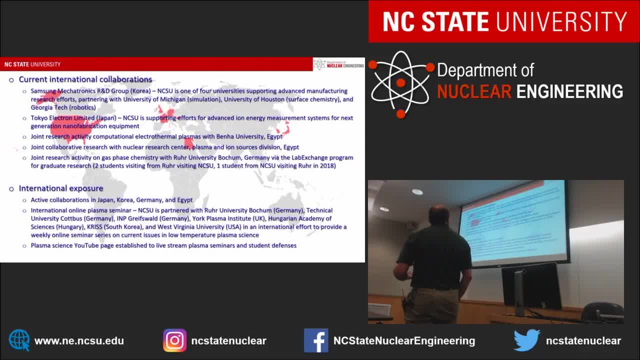 So we have a few. Our efforts are actually pretty international And we have collaborations with groups in the UK and France and Germany, Egypt, Korea, Japan, as well as the United States. We have an active biweekly plasma research seminar. 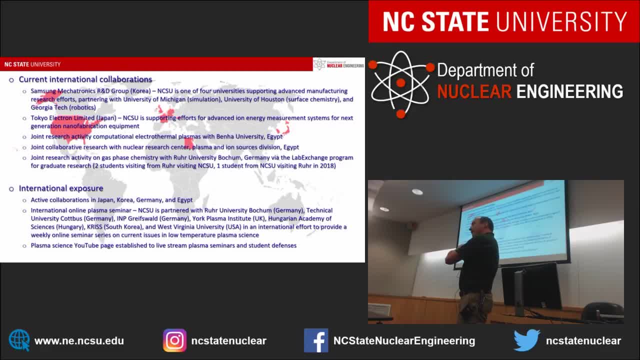 that we actually have it over in the conference room every other Thursday morning. So any of you who are interested in some of the current research going on in plasmas you're definitely invited to attend. We can send information out to the grad students later on that. 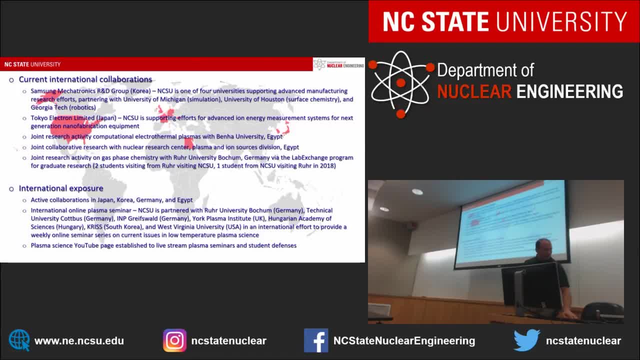 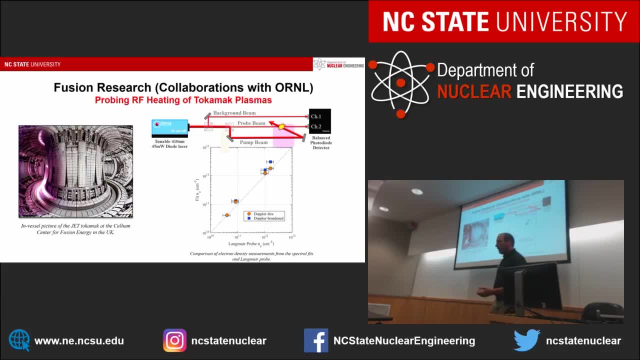 But definitely there's an opportunity. It's definitely a global research effort. We have a lot of collaborators all over the world- Some of the applications we work with. I'm just going to go through these really quickly. We do some fusion research in collaboration with Oak Ridge. 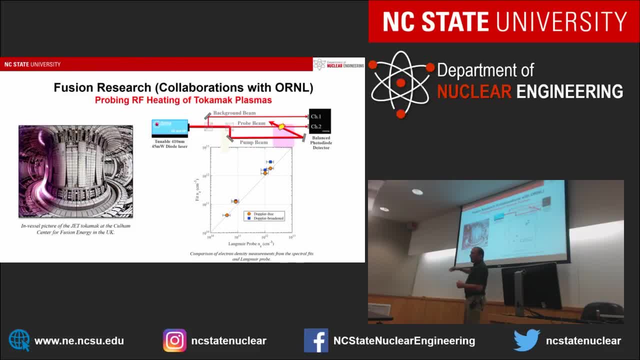 And what we really focus on with our work at Oak Ridge is working on auxiliary heating systems for tokamak reactors, in particular ion cyclotron range of frequency heating, And we are developing diagnostics to probe the plasmas in front of these antennas. 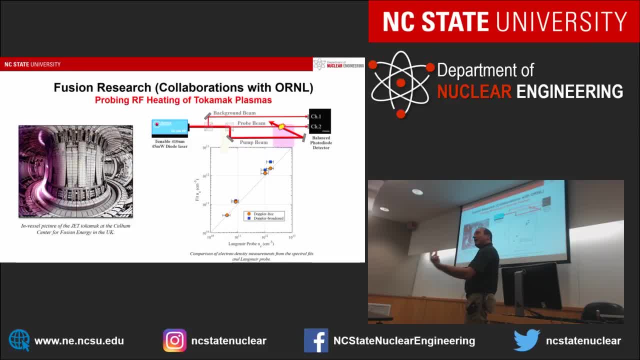 because these antennas will dump a tremendous amount of power into the plasma and can actually damage the fusion reactor if not properly modeled or optimized. In fact, the plasma fusion device over at Princeton NSTX blew a hole in its center stock because some of the RF energy that 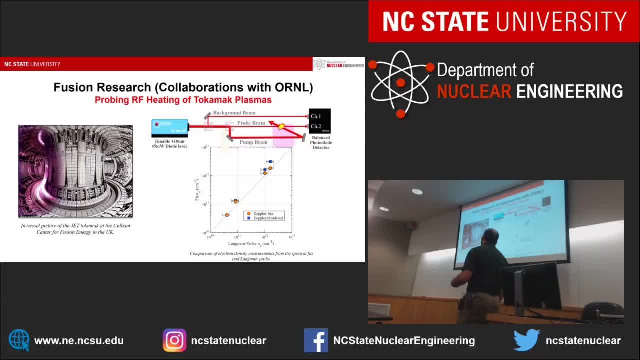 was going through the plasma diverted into the center stock and melted a hole in it. So having a better idea how these operate is definitely a more economic way to run your lab. So one of the diagnostics we've been developing is a pump probe laser diagnostic system. 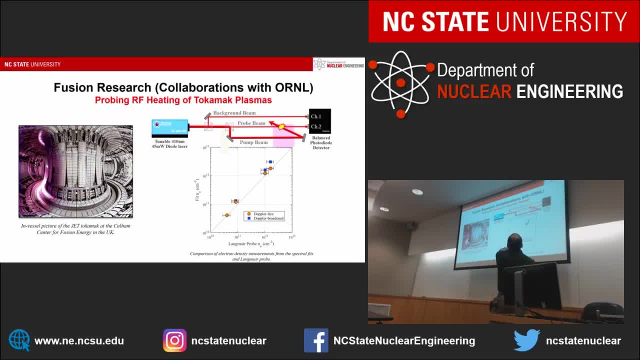 to estimate the density of the plasma in front of these antennas, And this is just highlighting some of the results in comparison to other diagnostics that one of our current graduate students, Abdullah Zafar, has come up with in his collaboration with Oak Ridge. 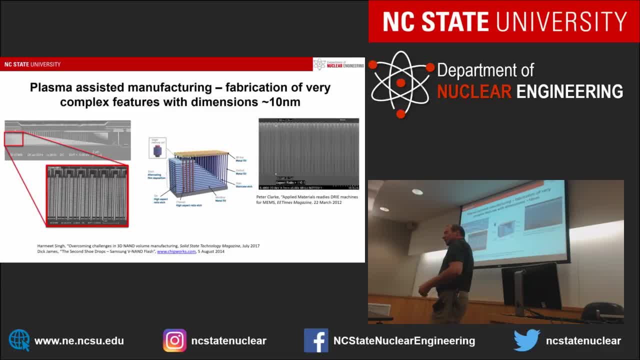 A big chunk of our research, though, focuses on plasma applications in industry, And what I highlight here are some very, very high resolution pictures of things you all have in your pocket right now. This is a NAND memory device that's being developed and is probably sitting in your phone or your iPad. 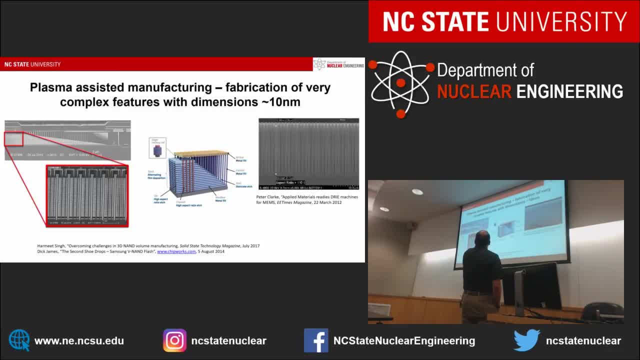 or your computer or whatever else. These are single memory cells that are being developed where you have to etch 10 nanometer diameter holes with 100 to 1 aspect ratio into complex film stacks. This is a cross-section scanning electron microscope picture of some 110 to 1 aspect ratio holes etched into silicon. 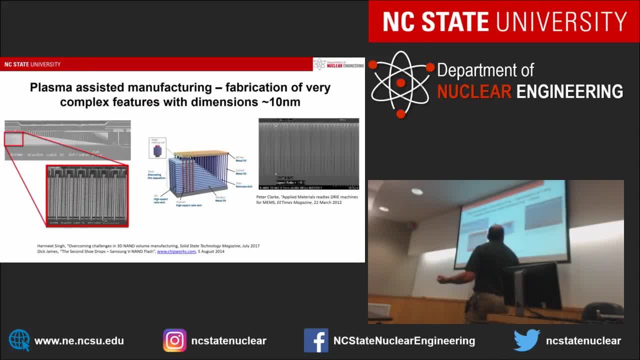 for memory devices. The smaller you can make these holes and the closer you can get them together, the more memory you can have in your computer. And you need plasma processing in order to do this. The nuts and bolts of it I'm not going to cover in a few minutes. 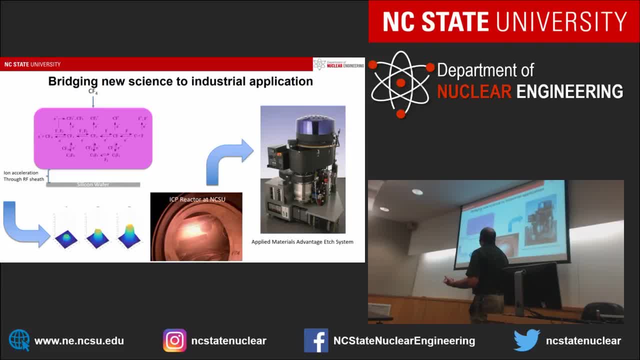 but I will say that we do play a role in this. The main thing that plasmas provide in these industrial applications is a combination of unique room temperature chemistries that you can't achieve through anything other than electron impact processes that you have in plasmas. 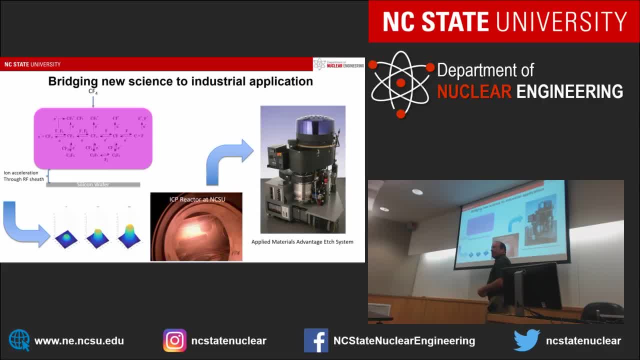 and ion acceleration at the periphery of the plasma, generated through something that's called a plasma sheath. Basically, the combination of these reactive species and the ions give you literally a plasma drill that allows you to cut these high aspect ratio holes into different devices or different materials. 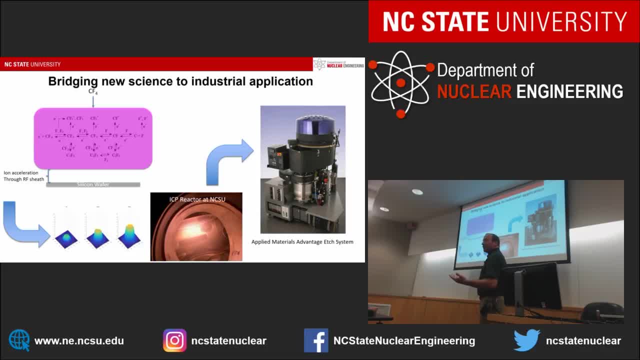 that you use for computer chip manufacturing. Now, our lab's role in all this is that we take these basic concepts of chemistry control, ion energy control and plasmid formation. We develop diagnostics and methodologies for extending this technology so that we can keep. 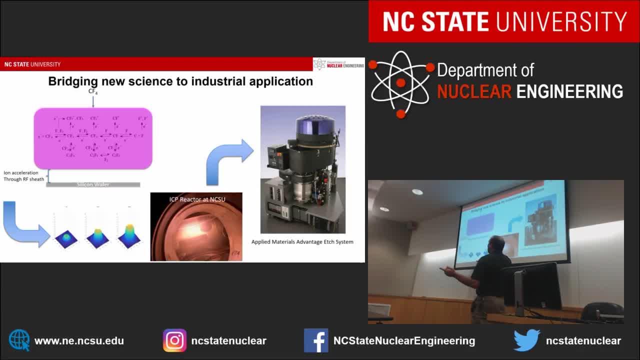 making better computer devices. We test them out in our reactors, just that way, about 50 yards in our lab. And so we test them out on research-friendly reactors And eventually our technology winds up on industrial reactors like this applied materials advantage etch system, which is a shameless plug. 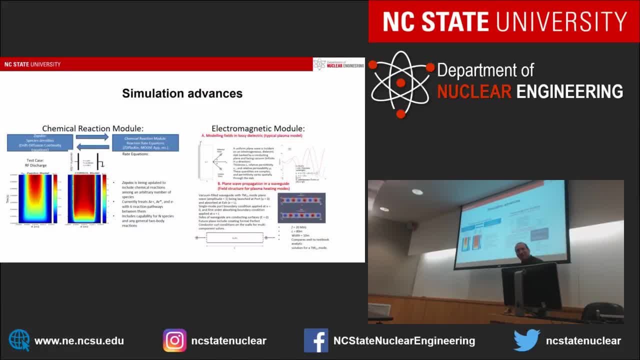 for my former employer. That's where I was before I came here. Now we not only do experiments, we also do a lot of simulation work. This is actually some work. for those of you who aren't interested in plasmas, We actually started using a simulation platform. 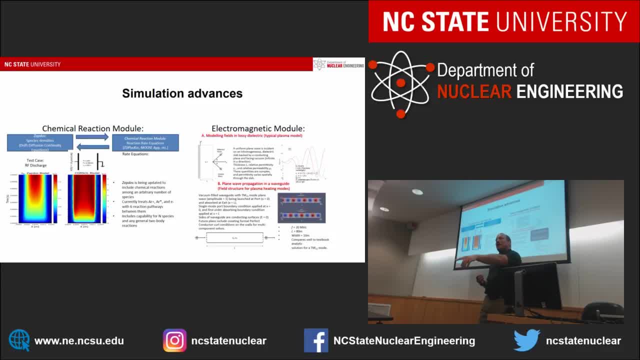 So Corey over here in the middle- hey, Corey is one of the students who's working on this- And we're actually taking the MOOS framework, which was developed for modeling nuclear reactor systems, And we're actually starting to use it for plasma simulations. 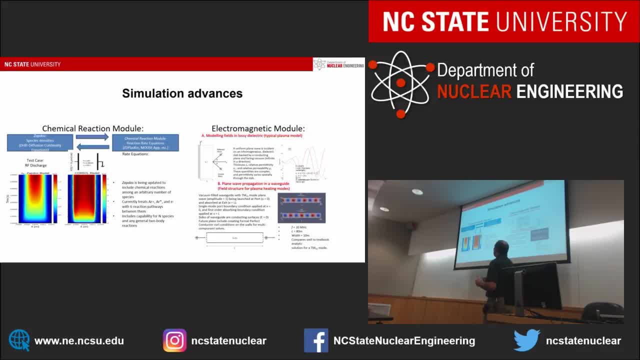 We got a collaboration with the National Science Foundation and University of Illinois where we've actually demonstrated been some success doing plasma simulation work in the MOOS framework. So taking something that was developed in CASEL and now using it for plasmas is kind of fun. 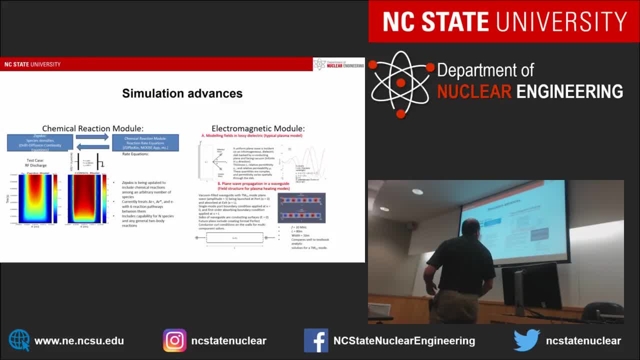 It allows us to talk to all the other people who don't do plasma stuff in our department. So we've got two students who are currently working on this in the collaboration with University of Illinois. I didn't know the noise was going to come on. 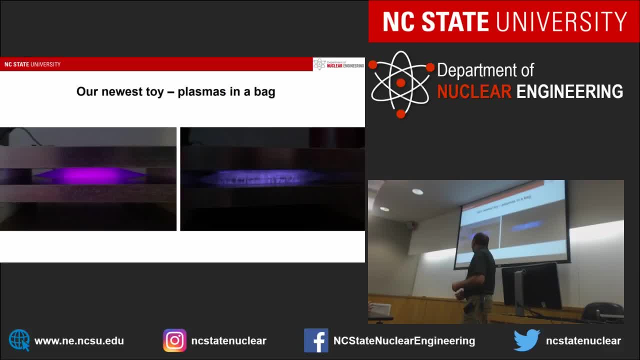 This is our newest toy and this is the one I'm going to wrap up with. This is a plasma in a bag. This is two, Two high voltage plates. This is a Ziploc bag And we fill the Ziploc bag with some combination of gases. 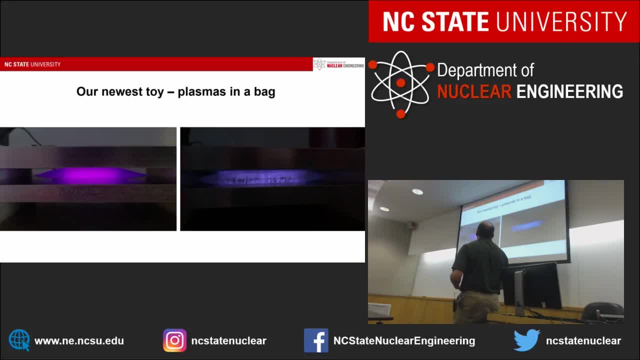 that we can use for sterilization or treatment of whatever we want to put in the bag. We then expose this to a high frequency, high voltage waveform between the electrodes And we can generate this nice uniform glow discharge inside the bag between these plates. 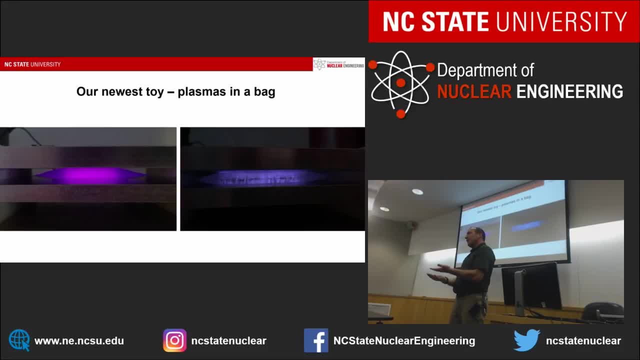 So think about if you had something that you needed to keep sterilized or you needed to treat, that you then had to transport. By being able to put on the process within the bag, we reduce the likelihood of cross-contamination And we've actually gotten a grant in collaboration. 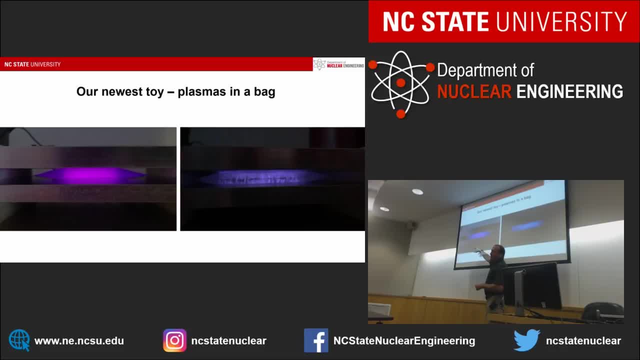 with a local company through National Institute of Health in order to develop this technology for the sterilization of material for internal medicine. This is actually a video of the same process running, but with powder in the bag that we're trying to treat, And you can see that the plasma actually gets the powder. 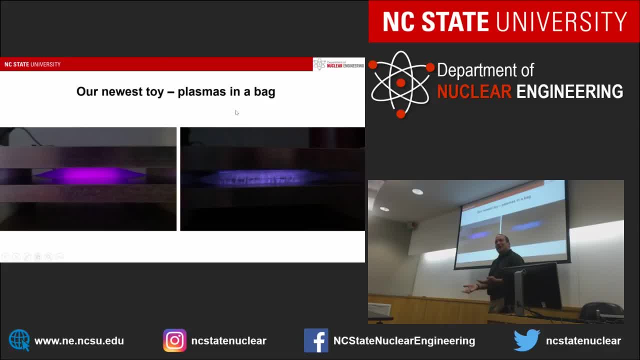 You can't see it, Never mind, I'm going to skip that. But the powder dances around and it actually agitates the powder. so we can conformally treat all of it, Treat all the surfaces. So this is one of our current projects. 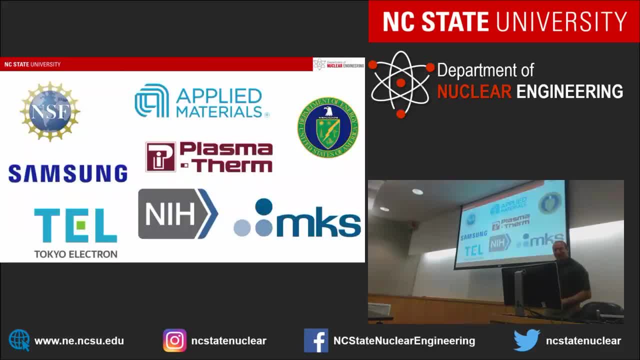 So I know I'm talking fast. We've got a lot of people we want to get through today. I guess the last thing I want to acknowledge- we all should acknowledge- is who's helping to pay the bills, And one of the things I want to emphasize here. 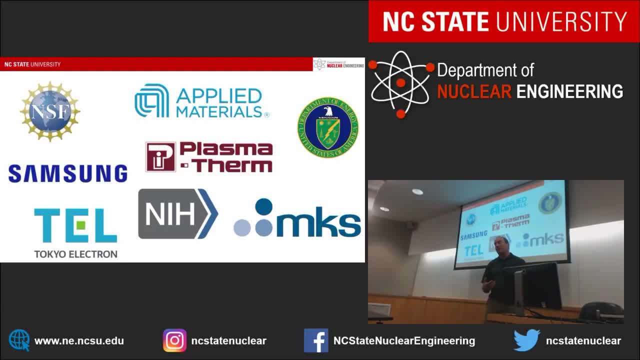 is that? actually, we've got some pretty diverse funding in our group. We have everything from industry, Samsung, Tokyo Electron, Applied Materials, Plasmather, MKS, And we also get federal funding from National Science Foundation, Department of Energy and NIH. 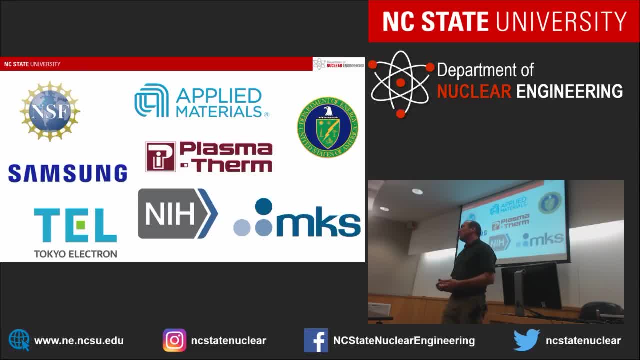 So we're kind of playing around Pretty much. anyone who wants to write a check, we're willing to do work for them, I suppose. So with that I think I finished up kind of quick, But while we get ready for the next presentation, 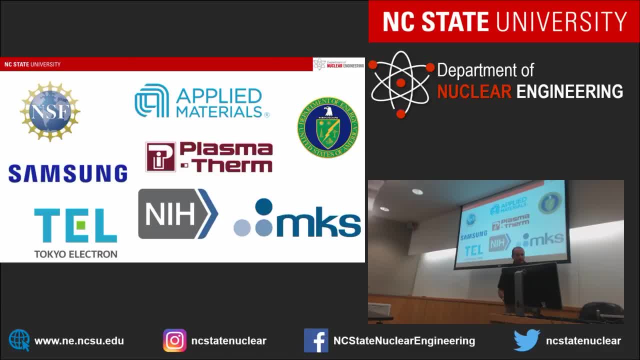 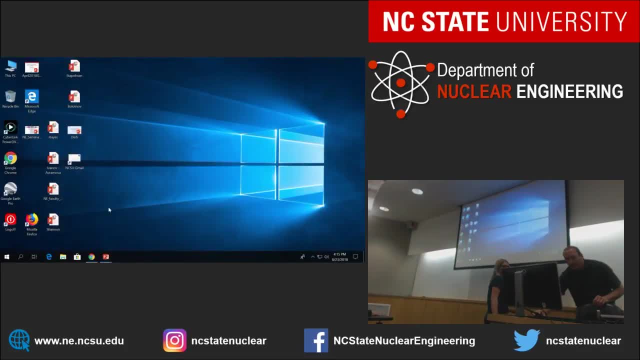 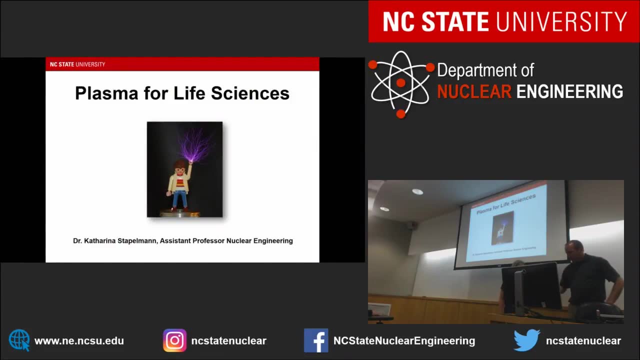 are there any questions? Thanks, You are Just going to hold it. Last time I used it, you could hear my hair scratching over the microphone all the time. Awesome, OK. So yeah, My name is Katharina Stapelman. 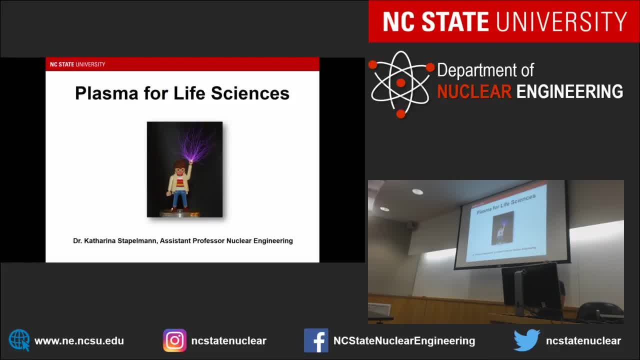 I joined NC State last year as assistant professor And I'm working on plasma for life sciences. What you can see here, I like it. It's a corona discharge actually, And yeah, So I'm working on atmospheric pressure plasmas solely. 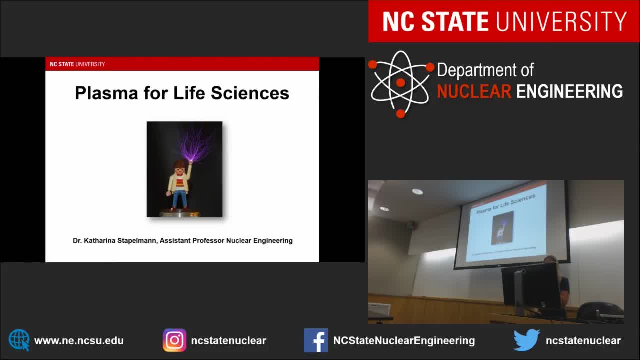 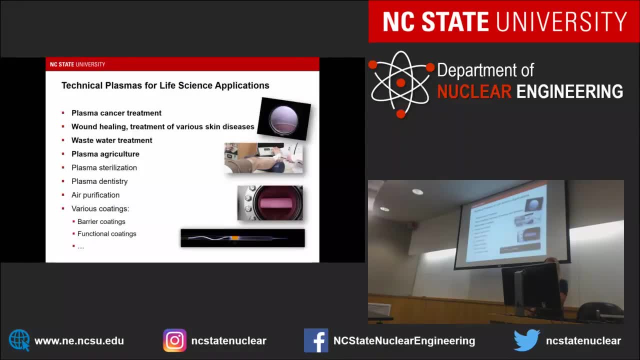 So Dr Shannon just showed some applications that were low pressure plasma. a little bit bigger Plasma in back is atmospheric pressure. I think, Yeah, I'm solely working with low pressure plasmas. The reason is with atmospheric pressure plasmas. 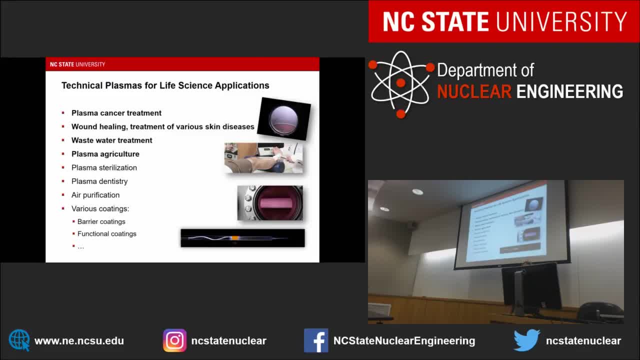 the reason is because I want to treat humans. You can't do that in vacuum. I mean you can, but only once. And the areas of application. I'm doing the research for life science applications. There are so many topics you can cover with plasma. 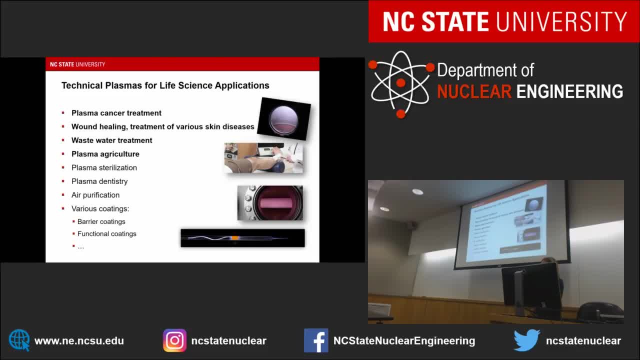 for life science applications, For example, plasma cancer, And I'm working on plasma treatment. This is really right at the beginning of research. We have some workshops already on the topic And in 2020, the next one will be organized in Raleigh. 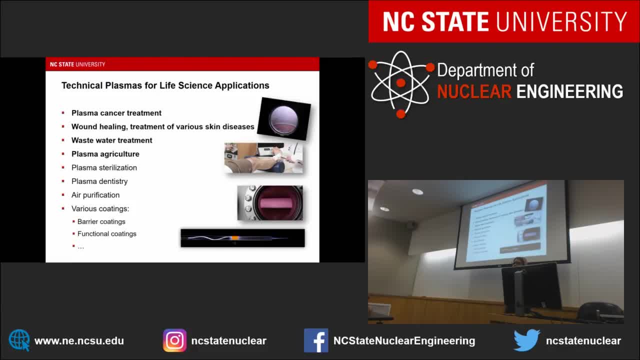 here at NC State. So this is really a strongly growing field with a lot of promising results, but still at a very early stage. Wound healing is one of the topics. There are some clinical trials Um In Germany. mostly In the United States it's kind of stuck at the FDA right now. 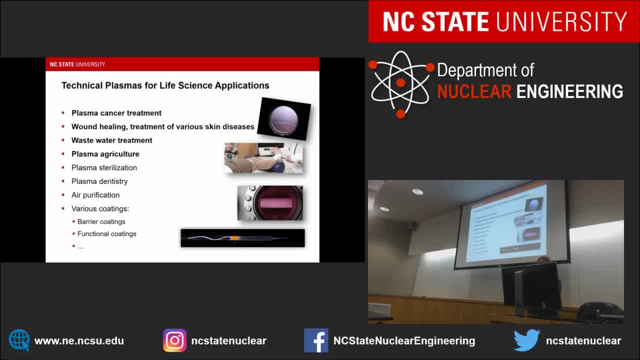 But I think the United States are getting there soon as well to get the first plasma devices really on the market for wound healing. You can also treat various skin diseases. You can treat wastewater. There's plasma agriculture as one of the topics, And those are the topics I'm dealing with. 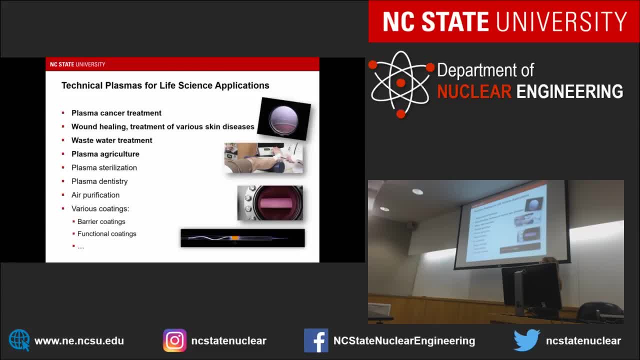 I'm doing research on, But also just to give you an overview: what's what's possible, what is within this range? plasma for life science application. There's also plasma sterilization, plasma dentistry- I imagine you go to the dentist and he's not using a drill. 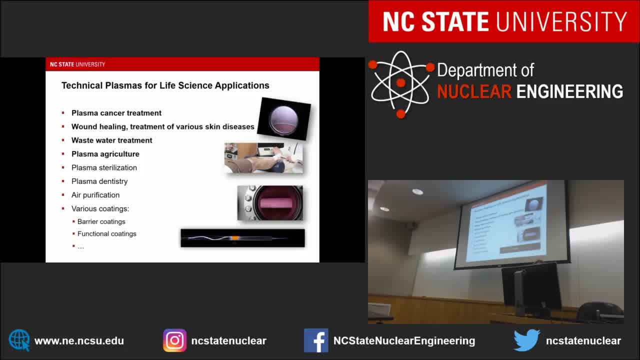 but a plasma Painless. That would be great. Purification is one big topic, especially for industries, And you can do various coatings: barrier coatings, functional coatings, For example the PET bottles where you get some bubble water or Coke. They're usually coated with a very, very thin glass layer, Because otherwise it would just lose the bubbles pretty fast. So they coat the plastic with a very thin layer of glass to enhance or prolong the shelf life of the product, And you still have the benefits of using a plastic bottle. 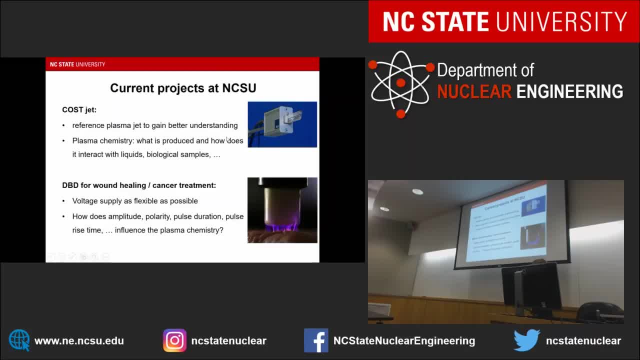 Those are some of the applications and the current projects I'm working on here at NC State- is the cost jet? this one, It's a reference plasma jet that was developed by a group in Germany and is used, I think, at five or six different places all over the world now. 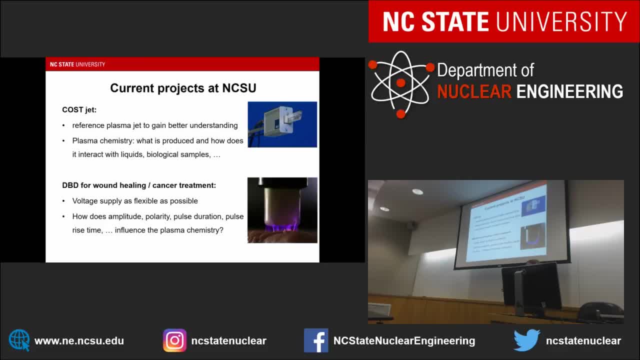 Everyone has different expertise, Everyone has different diagnostic techniques. So the idea of this cost jet is to have one source at different locations to gain just a better understanding of the plasma physics and what's going on, The plasma chemistry. So everyone has his own diagnostic devices. 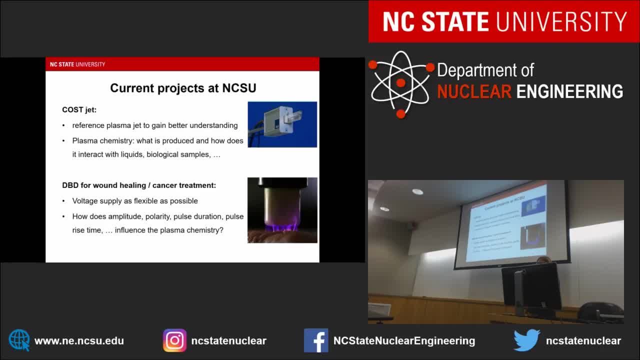 and his own ideas. So we are collecting a lot of data with this jet. I'm trying to understand the plasma chemistry. So what is produced and how does this interact with liquids and with biological samples and with biological samples covered with liquids? So there are a lot of complex systems. 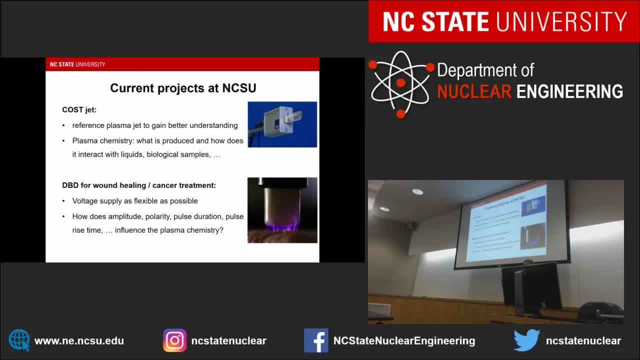 Plasma is a complex system consisting of different molecules. There are molecules and atoms and charged particles, And the radiation of the plasma plays a role. And then you have the liquid where you can produce some species. And then this whole thing is interacting with biological samples or, for example, 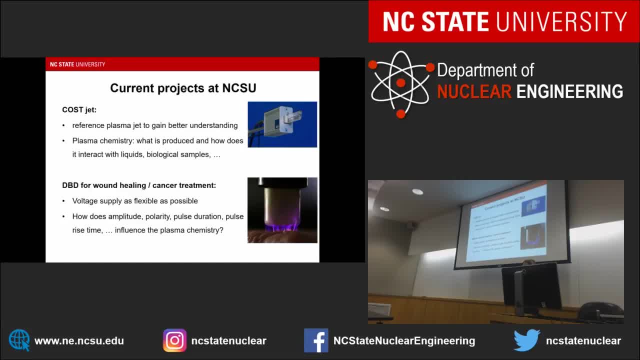 with skin, which is again complex. So a lot of complex systems interacting with each other. The next project I'm starting to work on now is the DBD for wound healing or for cancer treatment. The DBD is- yeah, the plan is there. 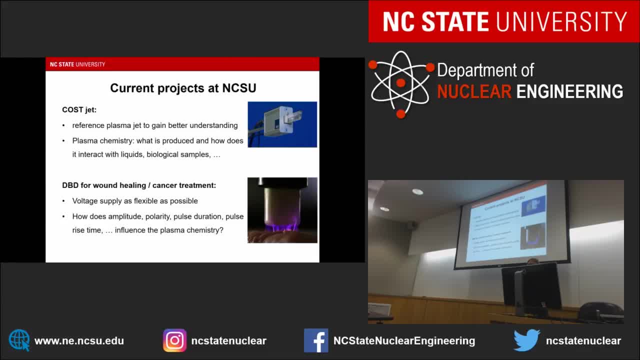 The parts are there but needs to be built. My idea is to have a voltage supply that is as flexible as possible. I want to adjust everything: The amplitude, the pulse rise time, the pulse duration, the polarity, just everything. And I want to investigate: how does the amplitude 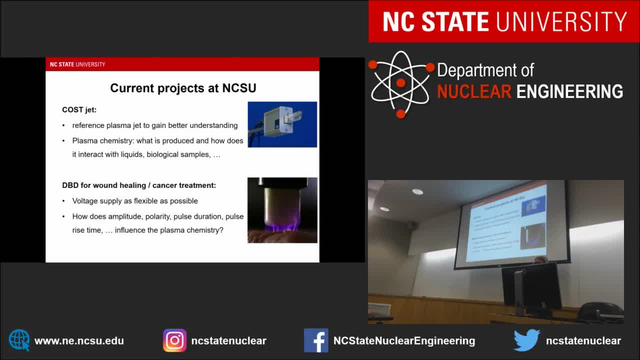 and the polarity and all this stuff influence the plasma chemistry, And is there a way to tune, by adjusting the voltage, the discharge, in a way that it just produces exactly what I want, in the amount that I want, for example, for wound healing or for cancer treatment? 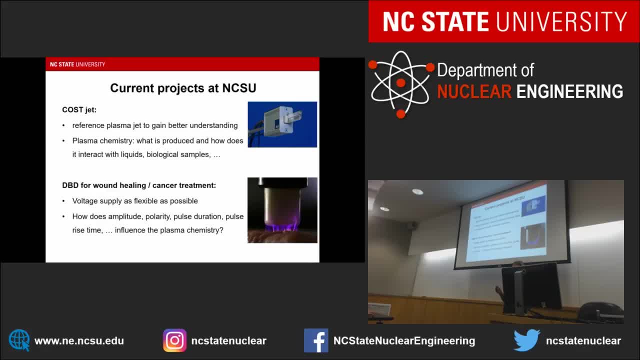 You can imagine, with one source, doing both wound healing and cancer treatment. Wound healing: you want to have growth. You want to have cells that migrate and that proliferate. You don't want that with cancer. You want the cancer cells to die. 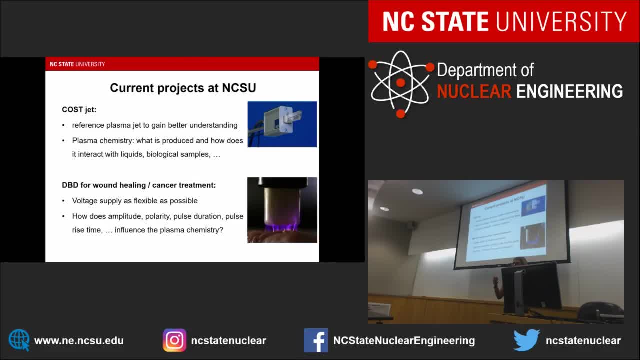 So it's just a question of the dose. You need to get The right dose at the right time, the right amount to the patient, And then this decides if you have a cell growth, an enhanced cell growth, or if you can kill the cells. 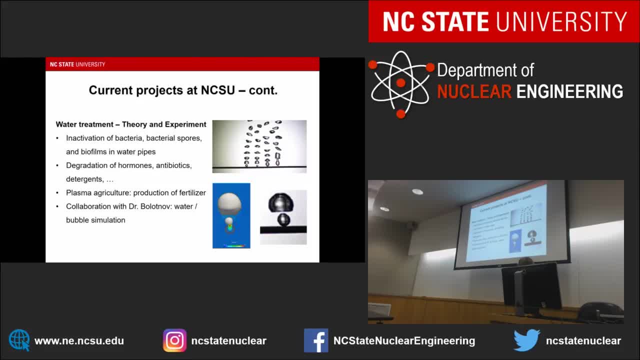 And the last slide for me is the water treatment for different applications. One application is the inactivation of bacteria and bacterial spores and biofilms and water pipes. Another application is the degradation of hormones, antibiotics, detergents, whatever is in our water system that we don't want. 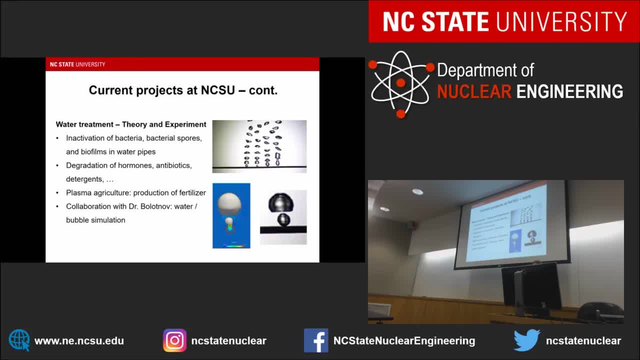 to have in our drinking water. And plasma agriculture is the next application where you can produce fertilizer on demand by igniting the plasma just in the water that you want to use to irrigate the plants. For this topic, I'm collaborating with Dr Bolotnov. 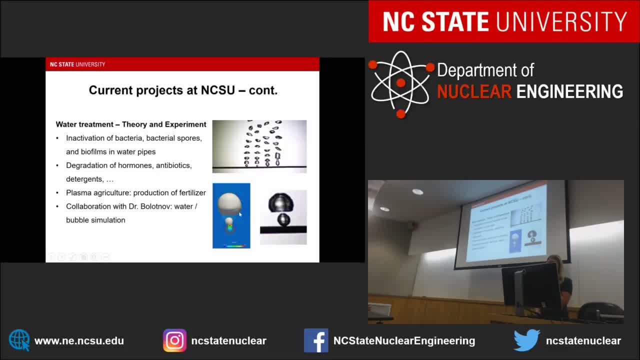 Naveen is doing some very nice simulations and sent me these two pictures. This is one from the experiment And this is a simulation picture, So I'm really glad that we have this almost same looking pictures. So we're making good progress in this collaboration. 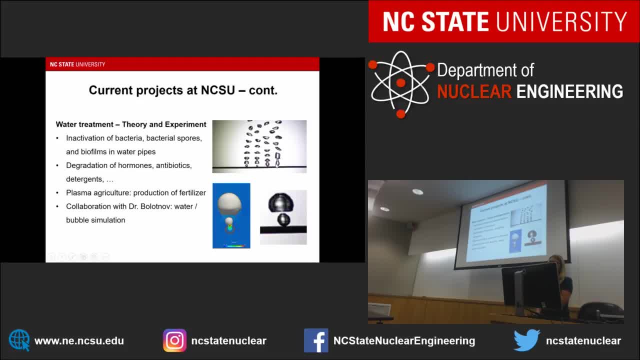 And this is a picture of the experiment. Just let some gas flowing inside the liquid, get these gas bubbles And I want to ignite the plasma inside the gas bubbles or along the gas bubbles. And for that, of course, it's important to understand. 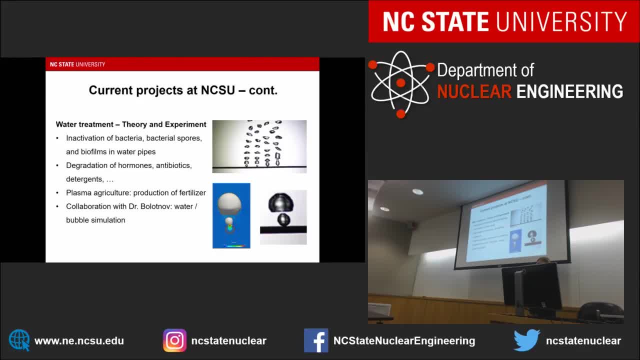 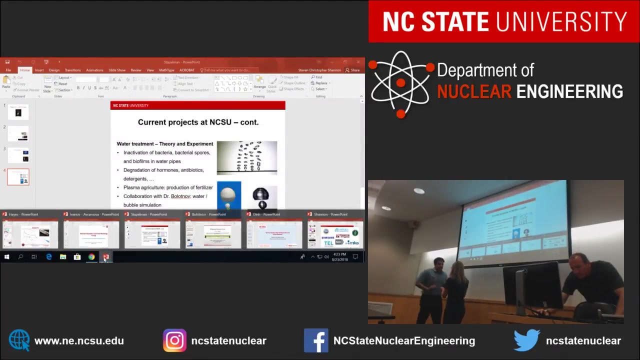 how do the bubbles form? How does the bubble shape influence the plasma? And that's what we are working on. Thank you, I don't need it. I use this room for to teach any two or two. Oh, we're live streaming. 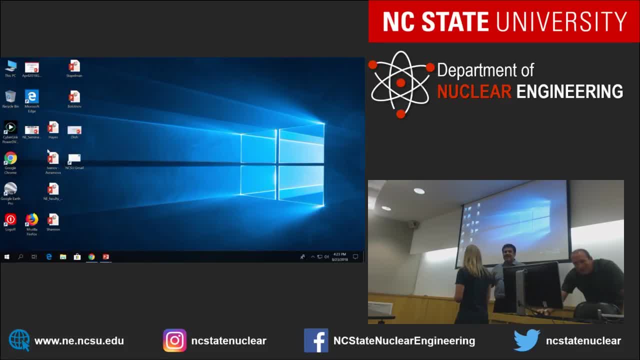 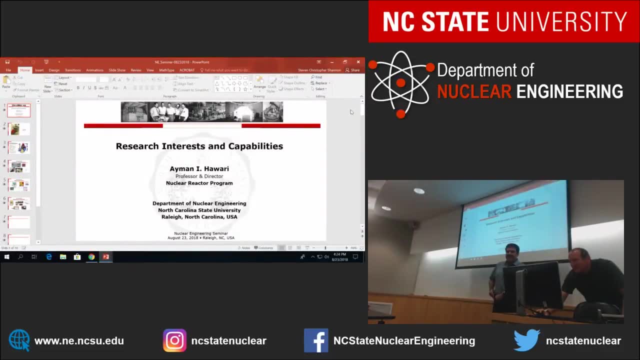 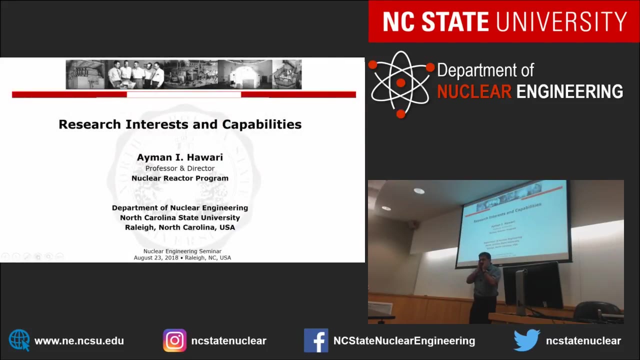 To who. Who's watching? The world is watching. OK, because I'm loud, usually Ask my students. But OK, you got me All right, thank you. So after hearing all this, I'm thinking: oh my god. 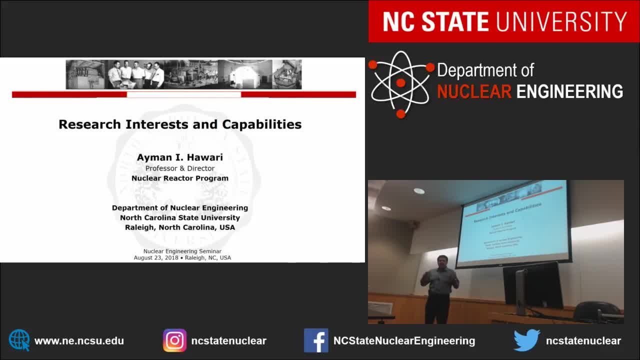 I'm so traditional because I'm actually a nuclear engineer that works on reactors, So I'm a little bit too traditional, I think, in the way I work And I like nuclear reactors. I like them in many different ways And I work with them from both looking. 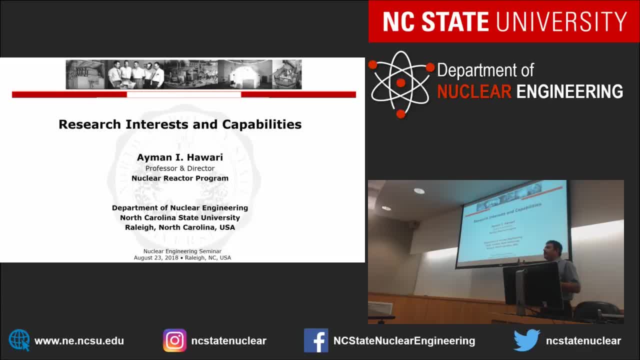 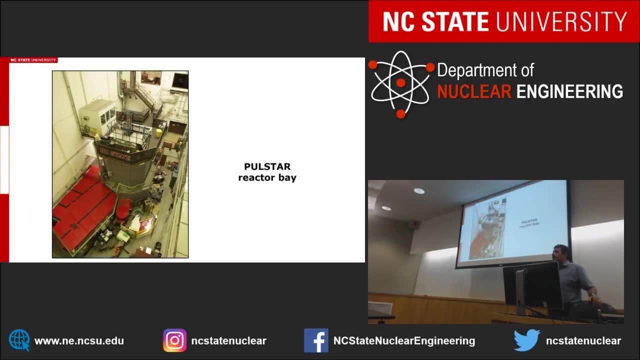 at the fundamental phenomenon of radiation and interactions that happen in a nuclear reactor, and also the applied nature of the interaction process itself. One disclaimer is That I need to make over here is that none of the pictures and images and plots and graphs were made by me. 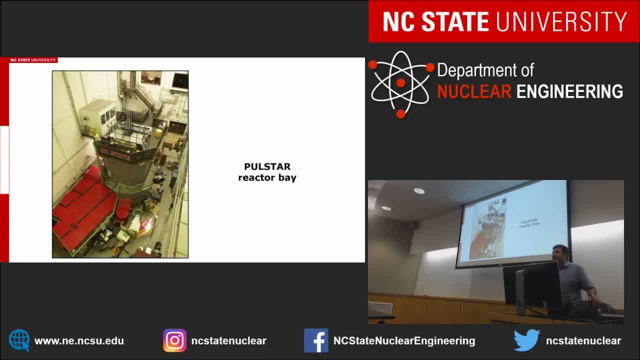 in this presentation And students and researchers in my group that are sitting here will recognize stuff that they did. So just don't consider me that I plagiarized your presentations. Polestar reactor is the first reactor and the main reactor I'm working with on a daily basis. 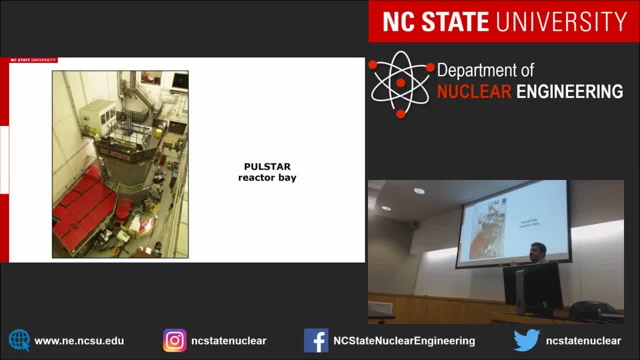 This is our Bay Area And if you haven't visited, this is something that you might want to do. Take a tour and look at everything that we do. We have a very busy activity level in this reactor, with all of the facilities that we have developed. 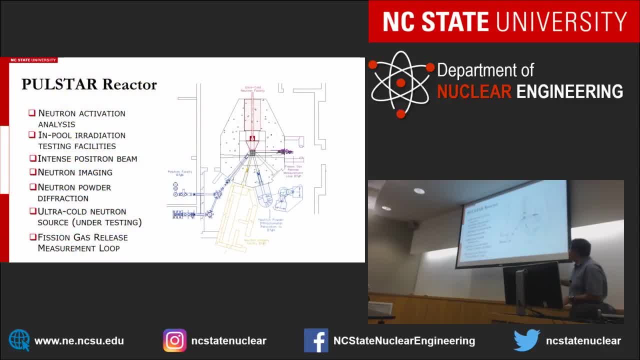 and all of the nature of activities that we have. Just to give you an idea in a schematic fashion, we really viewed this reactor as a major radiation source And we're using the radiation emanating from the core of this reactor And we're using it. 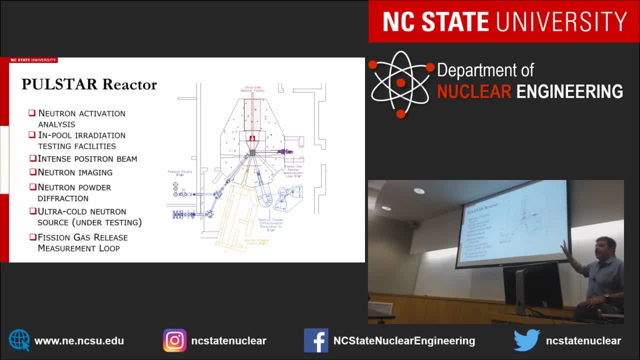 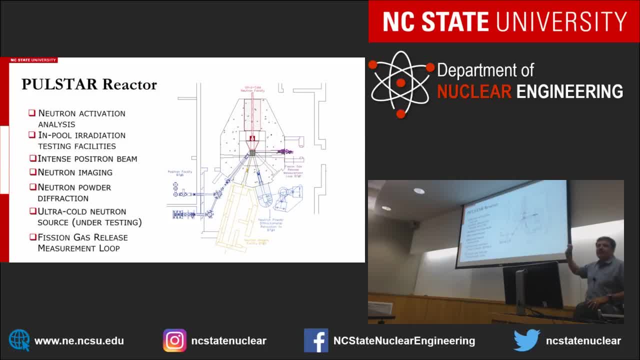 We're using it also to generate positrons and using them as radiation probes. We have fundamental experiments going on with neutron physics and the use of ultra-cold neutrons. We have nuclear energy-oriented experiments where we are testing, building, and soon to be operating, a fuel testing loop here in the reactor. as you. 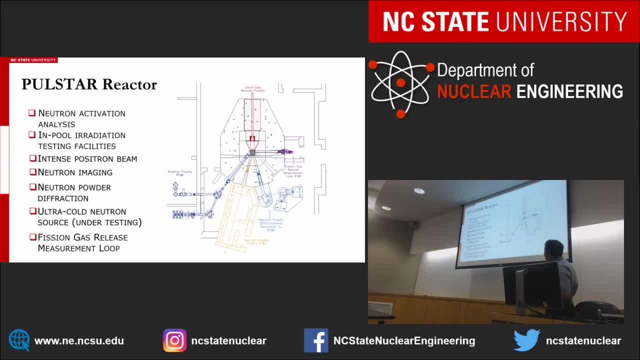 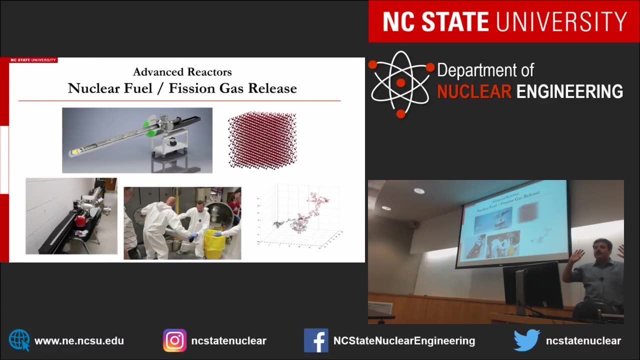 see, and this is one going to be one of our main and newest facilities going online in the very near future. but in addition to doing all this and all of the work that we do, that I thought of the theme that our group is is really moving into and we really move in a theme that you could consider as a 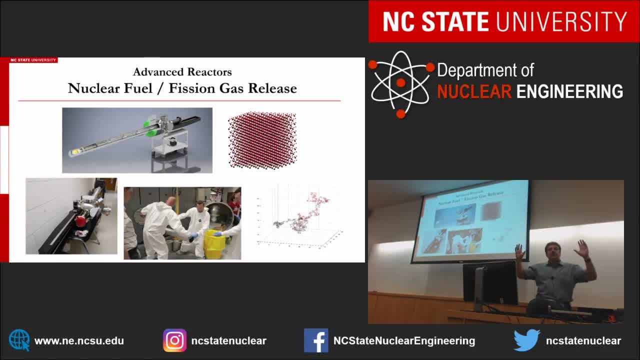 general umbrella for it, the title of advanced reactors. because everything that we do in terms of the fuel research, in terms of the fundamental physics analysis that we do in terms of the development of instrumentation and detection techniques, all really falls, whether programmatically, from a funding point of view, or even scientifically and engineering wise, under the advanced. 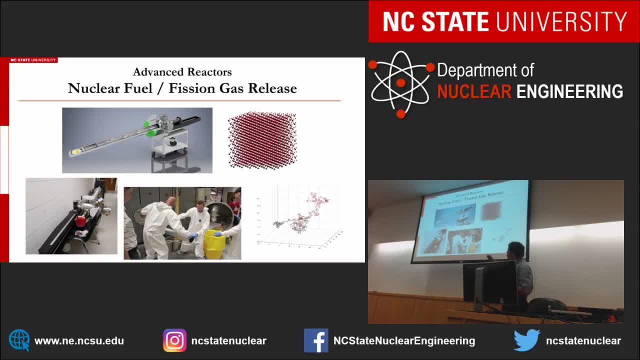 reactor umbrella. and this is the loop- and I put it here on purpose. this is the loop that we're going to be using in the future and this is the loop that we're designing, and some people may recognize these figures. I think is it you, Cole, that? 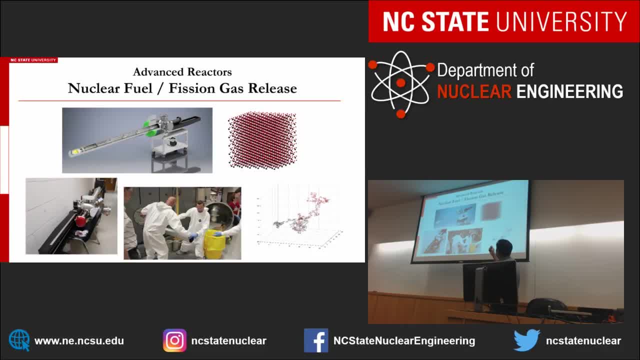 made this okay, so I'm guessing right, because I was wondering where these figures came from. and- and this is a schematic of the loop that we're building and we're actually testing its insertion. you could see, here we're also looking at fundamentally what this loop is going to generate for us. it's going 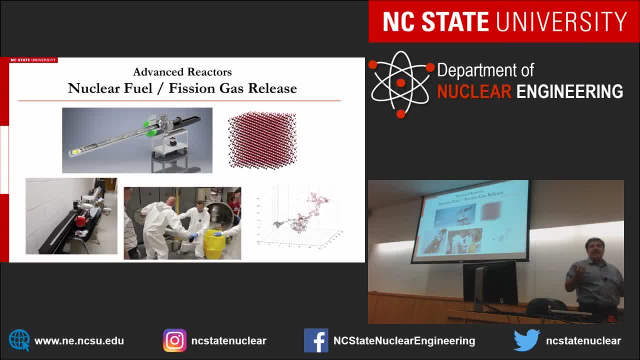 to generate information about the release of fission gases from advanced nuclear fuels and we're trying to understand how this release happens on an atomistic scale. so we're resorting to atomistic simulation techniques to not actually model the atoms, but we're actually modeling the vacancies, almost like modeling the inverse of matter, the lack. 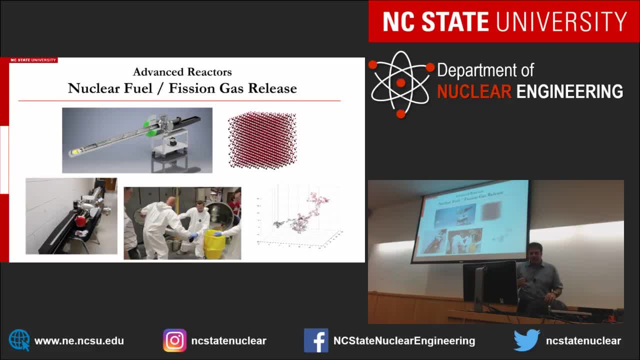 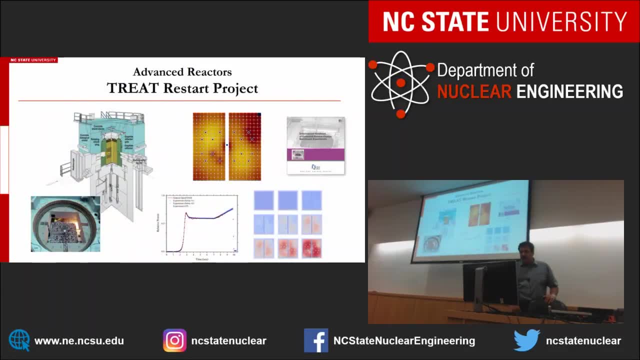 of matter and trying to track how these vacancies move around, because they are actually the main mechanism by which fission gases move in nuclear fuel. another project related to this is a. we are also help restart the treat reactor at Idaho National Lab and the testing of nuclear fuel, and Colby Sorrell here is working on that heavily and I think 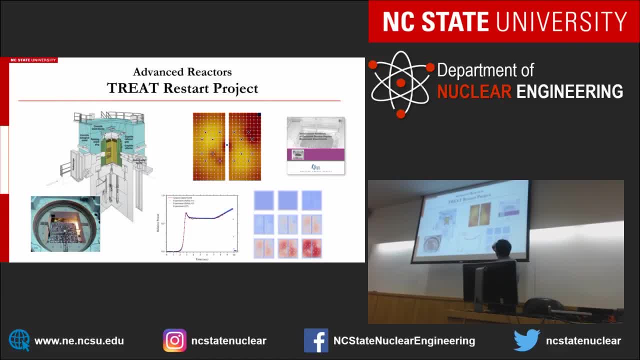 these are pictures from you right and what you could see here. this is treat. treat is a pulsed reactor that has just gotten restarted after about 25 years of hiatus. we are actually modeling the transient operating phenomena, and I show here a transient that were with experimental and computational 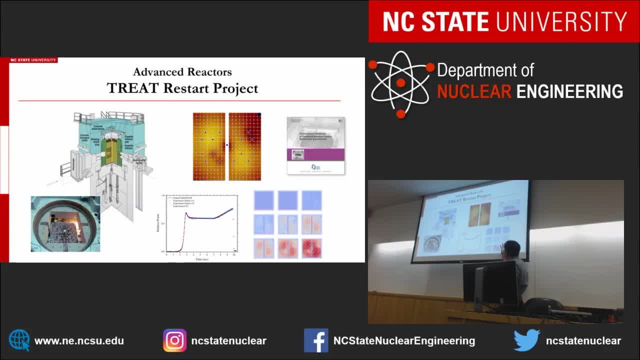 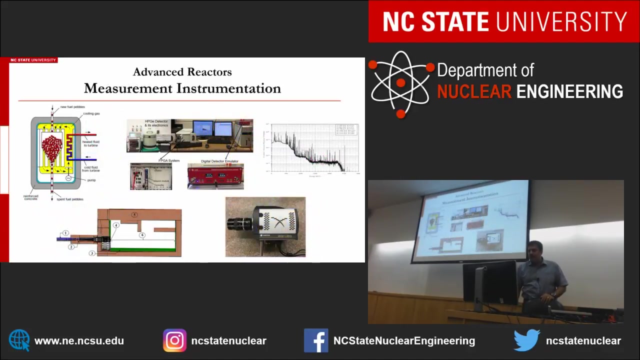 predictions of the transient and the evolution of energy distribution and temperature distribution in the core, and we're hoping to be able to contribute our transient simulations, coupled to the experimental data, to the international reactor physics handbook, which is which puts together all of the international effort in benchmarking in a place that users can. 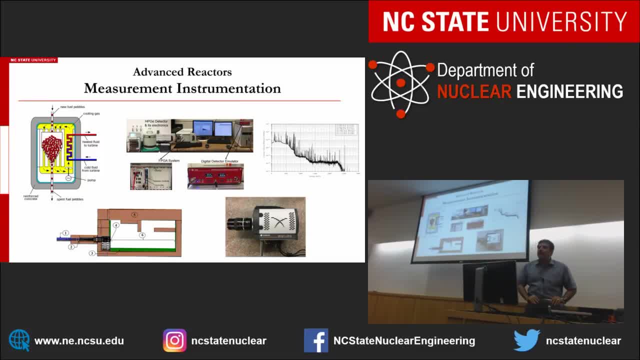 resort to, again to support understanding fuel phenomena. we're developing very advanced instrumentation. by the way, this is a gamma spectrum and, just because there were questions about it, we're developing very advanced gamma spectrometry instrumentation. why is it advanced? because traditionally, right now, when you go and you buy off-the-shelf gamma spectroscopy or spectrometry, 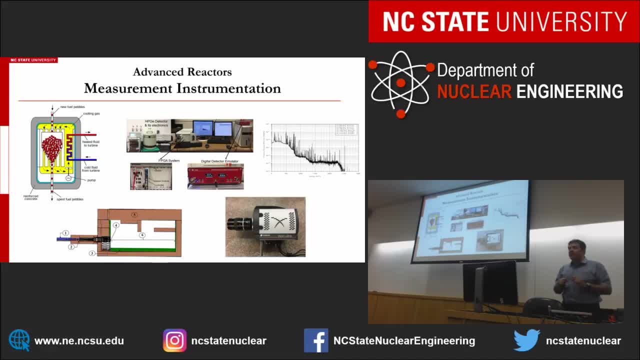 instrumentation. it's almost a one-size-fits-all, so you set it up and you leave it and it does the detection for you. here our gamma spectrometry instruments actually look at the radiation environment and decide how they want to operate in that radiation environment, if the radiation 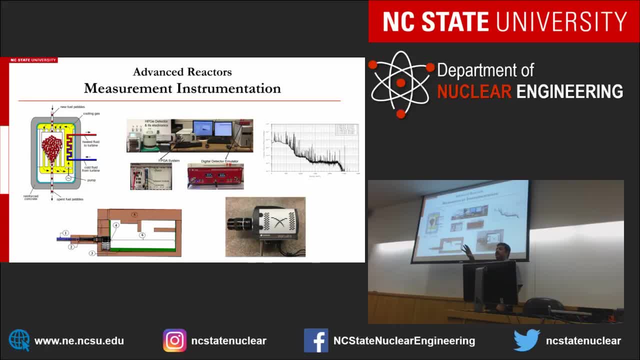 environment is very hot and intense, the spectrometer will start adjusting itself to match that radiation environment and to collect the information in the most optimum fashion. that results in the best resolution, that results in the best throughput and count rate, without any risk of failure. We're using FPGA technology to do that. 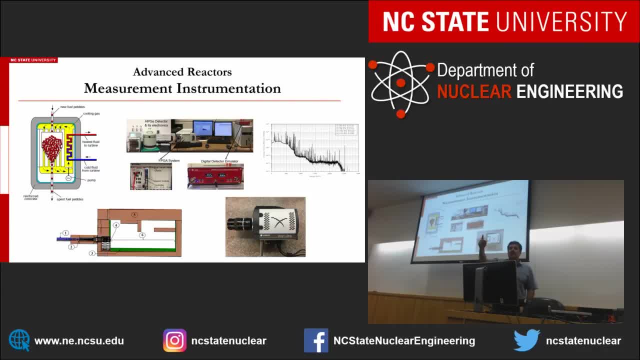 Some folks I think might be here who are dabbling with FPGA. you guys are dabbling with FPGAs. Shapali Saxon has been working on this for a few years now and she's near graduation with her PhD on this. We're also working on the visualization process, so we do a lot of imaging and 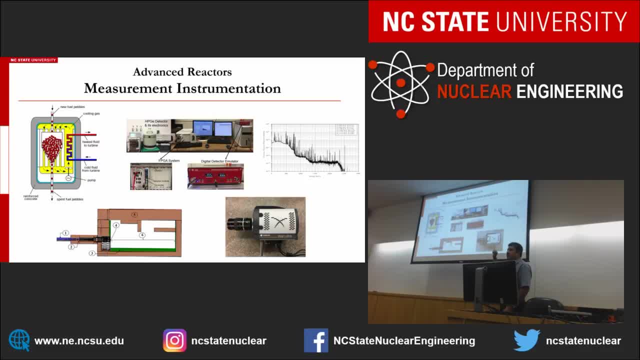 we've just started installing our dynamic imaging systems in the reactor. Again, one of our interests is to be able to image fuel structures and look at the damage in these fuel structures, and also do it in a flow environment. So these dynamic cameras that we have been installing and using can capture a flow environment, for example. 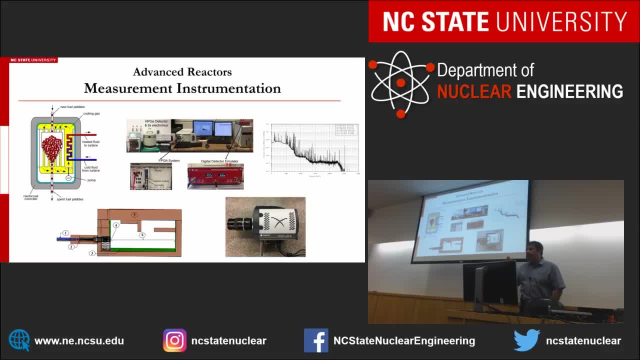 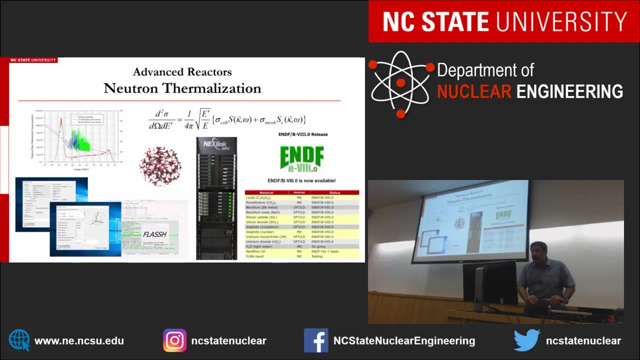 And again, our thinking is that this would be quite applicable to advanced reactors Like, for example- what would this be? Pebble bed reactors- Again advanced reactors- and neutron thermalization. This has been a staple of our operation and probably one of the biggest bill payers over here. 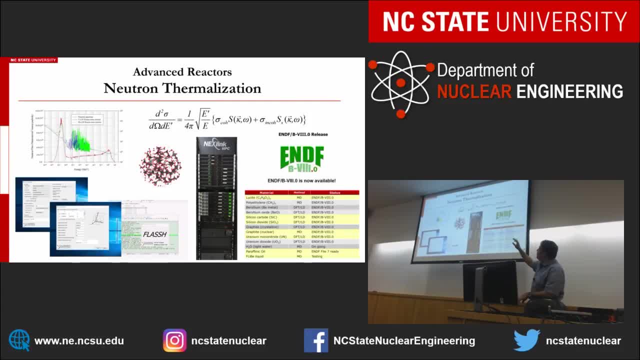 And there are too many bill payers. But this has been really a major piece of work that we started many, many years ago in this group. And again, the motivation is to understand the operations of these reactors. You really need to understand the reaction rates. 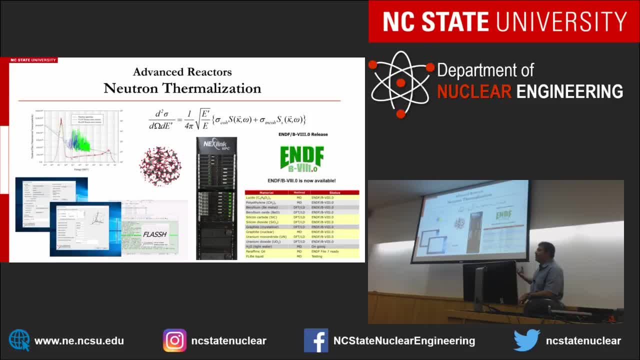 Inside the reactor and the reaction rates depend on the neutron spectrum in the reactor. And if you don't know the neutron spectrum accurately, everything gets thrown off, from basic operations to safety, And one of the largest sources of uncertainty were the cross-sections, especially at low energies. 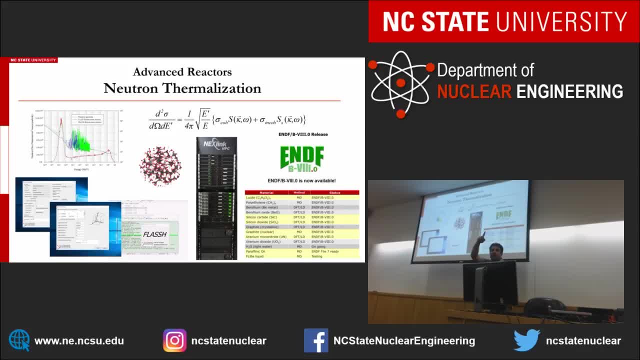 This is really the workhorse equation. My students over here have seen this too much. You can close your eyes if you don't want to look at it anymore, And many of our group members right now are still working. We're a big contributor to the NDEF-8.. 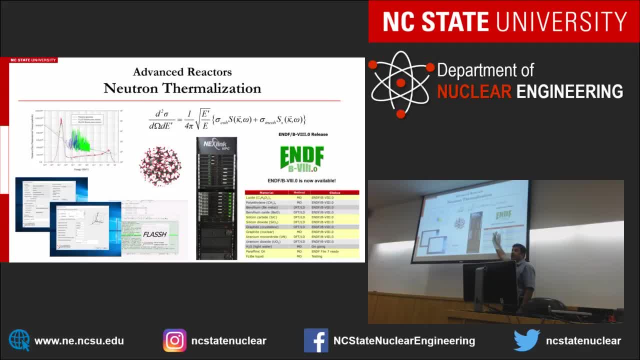 So if you use NDEF data libraries and cross-sections, probably you are, even if you don't know it, if you're doing any kind of neutronics calculations. And these are all the libraries that we have contributed in the last two years. 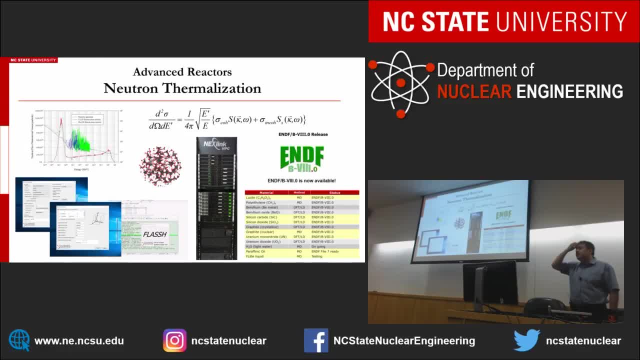 So we have 11 libraries. I think there were 15 contributed to NDEF-8.. 11 came from us at NC State, And so we are probably the largest in the world. We developed a new platform We're aspiring to. 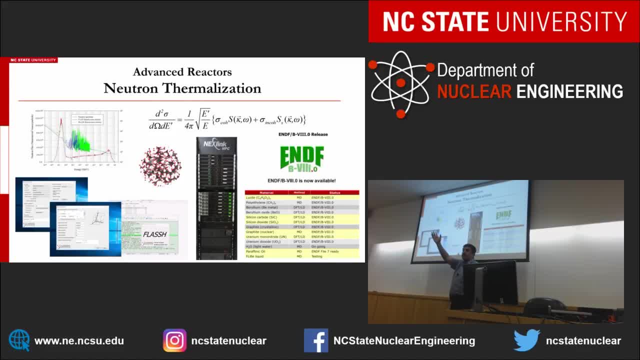 Who knows the ENJOY data code? Anybody used it, Everybody knows it. We think we can replace it. We have FLASH And FLASH is a new system that now certainly replaces everything in ENJOY that deals with thermal scattering. We think that we can take it a step further and couple it to even higher energy treatments of the cross-section. 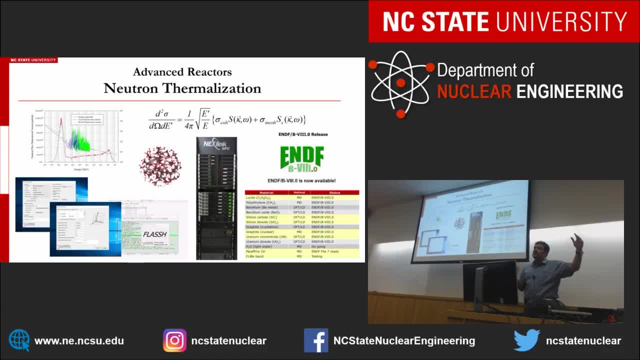 And if we do a little bit of work on that, we're starting to think that we can take out the whole ENJOY thing. But I'm not telling Los Alamos. I'm not telling Los Alamos that yet, Because you know I'm scared. 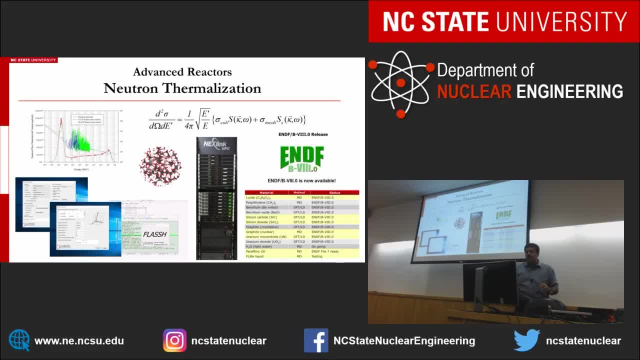 I'm scared to say that. So we do a lot of atomistic simulations that support this, Because really at the heart and soul, thermal scattering is sort of an area between materials and neutronics. It's a very special area, An interface area. 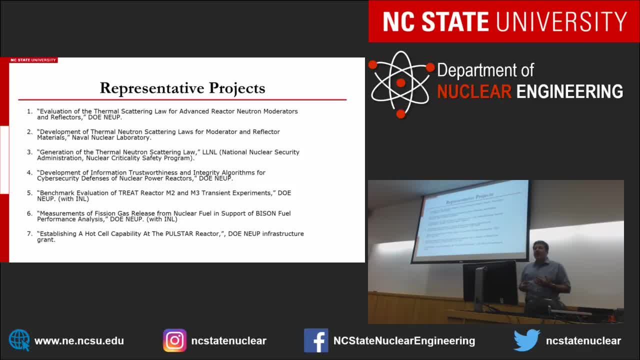 These are representative projects that we have. We collaborate a lot with national labs And, of course, we're sponsored by government agencies Like the Department of Energy Naval Reactors, NNSA, And so we have a lot of that going on. 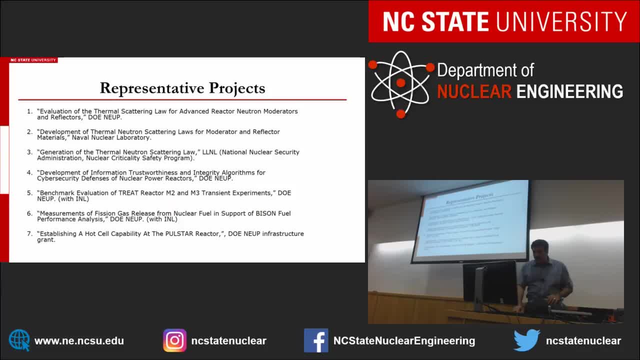 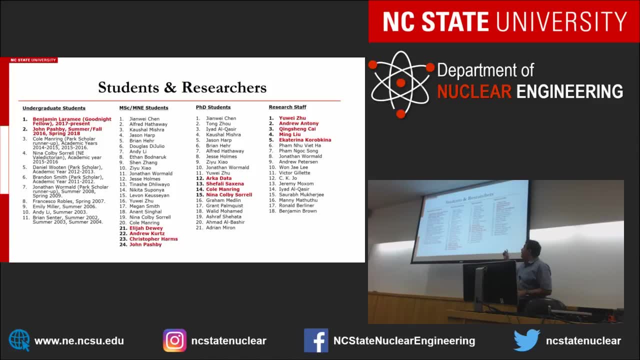 These are active projects. Some of them are just brand new and starting, And we aspire to have more in the near future. This is the family tree. This is the family for the past 20 years, So we have a lot of members in our family. 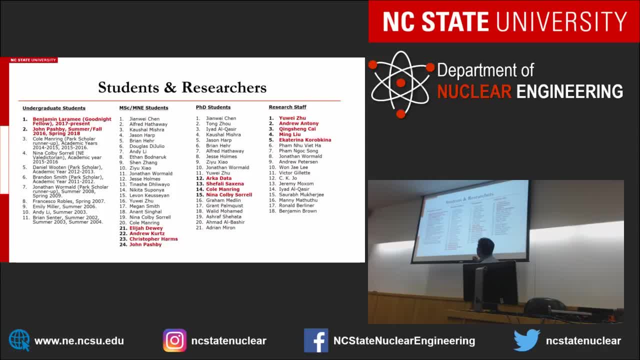 And the red ones are still at home And one day they will leave home. I know it's sad, But that will happen. And Yuezhu is the latest addition- They move this way, by the way, So this is the youngest. 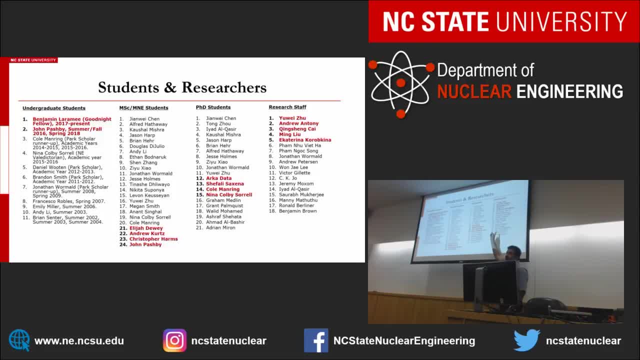 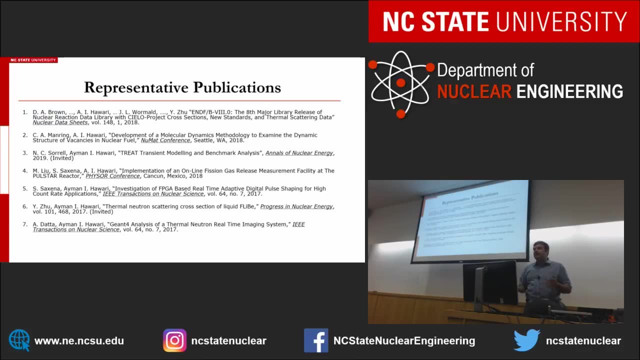 And they get older, older, And then Yuezhu just went here over here And so it happens. But we're very proud of the family tree over here And representative publications We publish in journals like Annals of Nuclear Energy, Progress of Nuclear Energy. 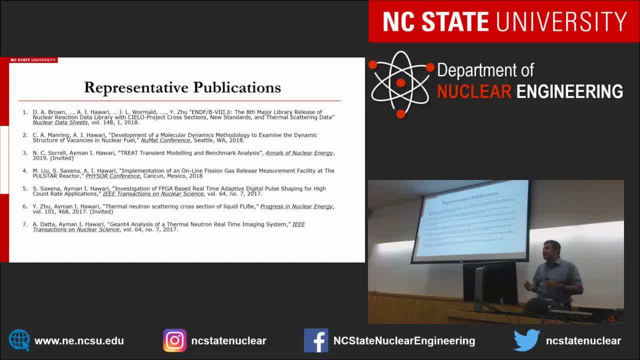 IEEE Transactions on Nuclear Science, Nuclear Instruments and Methods Conferences. We go to FISO, We go to NUMAT Nuclear Materials Conferences. A lot of what we do overlaps many areas of research And we have been populating many of these conferences. 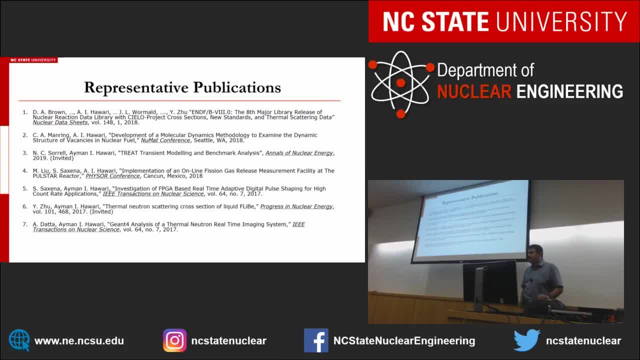 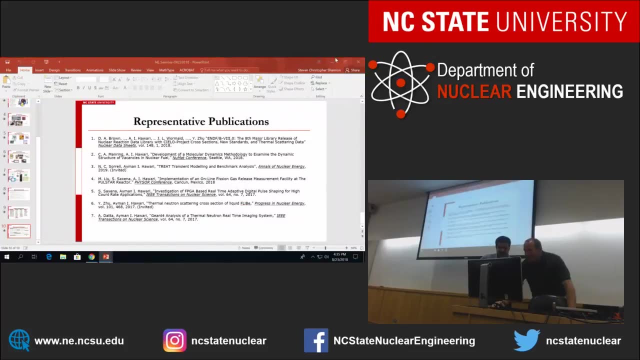 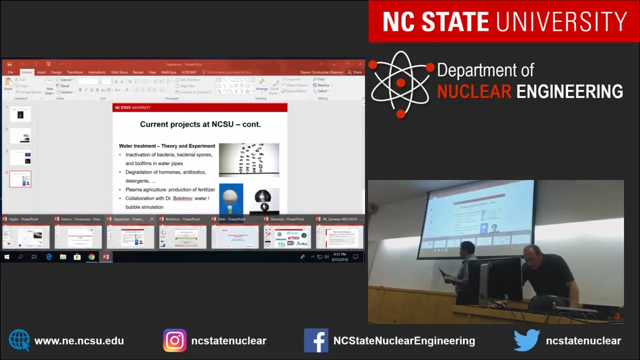 Okay, That's it, Thank you. Questions: No: Oh, Okay, No, we're not used to this live text, Sorry, Thanks, Thank you. Can you hear me? Yes, Yes, You have to talk. It's not on the speaker. 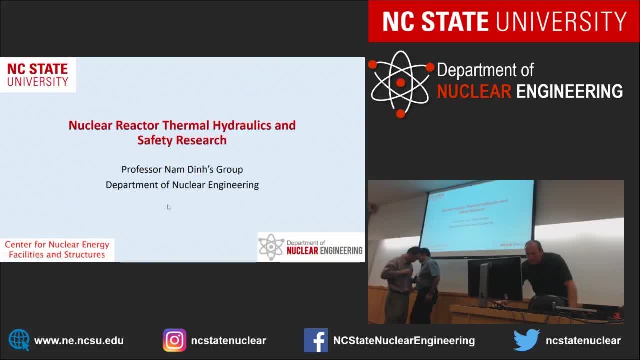 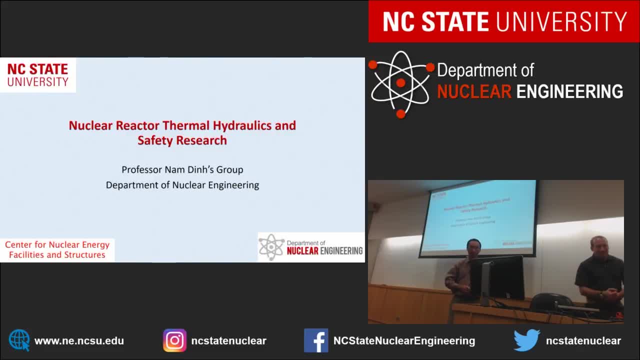 Thank you, Thank you, Thank you. I talk low voice, so my topic here my group is doing nuclear, thermoelectric and safety. So safety is my area and safety is not observable. We study safety, but safety is not observable. 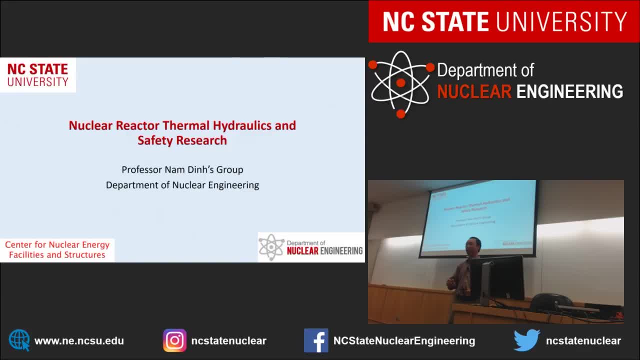 What's observable is unsafety, Sometimes until we have accident. then we realize that we have something unsafe, So that safety is illusion. So chasing after illusion is something very tough, And so this is two areas of my research: thermoelectric and safety research. 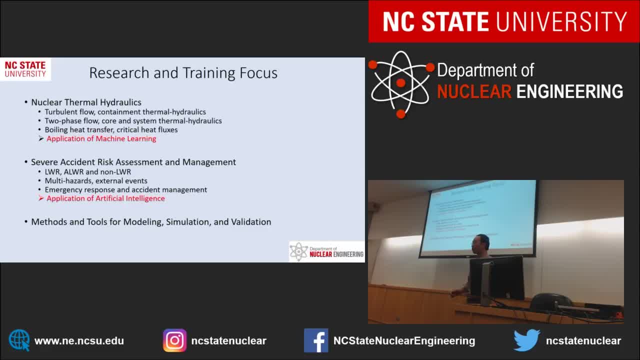 I'm doing stuff, very classical stuff, Nuclear thermoelectric. we're talking about turbulent flow, containment, thermoelectric two-phase flow in a core and in a system, boiling, heat transfer. You learn a lot about thermoelectric. You know that this is basic thing in thermoelectric. 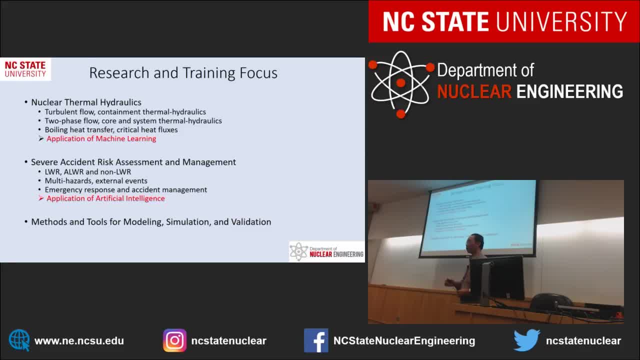 It's very interesting, It's preventing boiling crisis happening in nuclear reactor, So it becomes safe to become unsafe. And my area- the one I've been working for 20 years- the severe accident risk assessment and management. we do assessing the risk of accident. 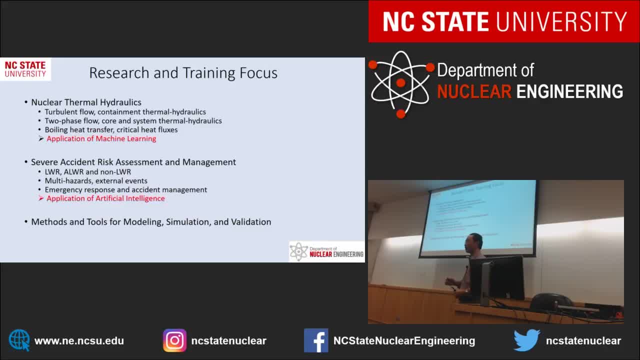 Because when we care about safety, it's risk of accident. How do we assess the risk and then managing the risk? And what happened in nuclear reactor? we deal with a very high consequential hazard And we have very low probability risk, Although it's too hard for multiple people to cause severe accidents. 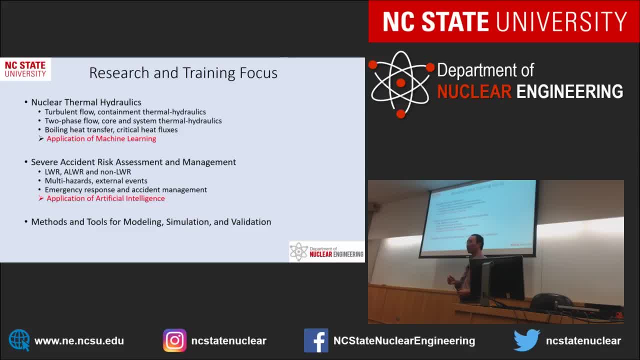 But that's very low. probability And risk is something, and consequences. We deal with probability in small number and consequence in very large number and take multiplication of the most small number and large number And then we have to deal with the risk. 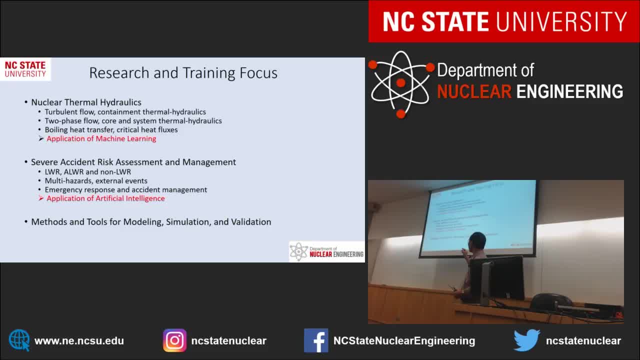 So uncertainty become very important part assessing that. So I'm dealing with for non-light motor reactor and介 factory. It's them who PLAY LETTER TURN 06対 여기에해�, vida pointers and accidents management. So those are very traditional thing. 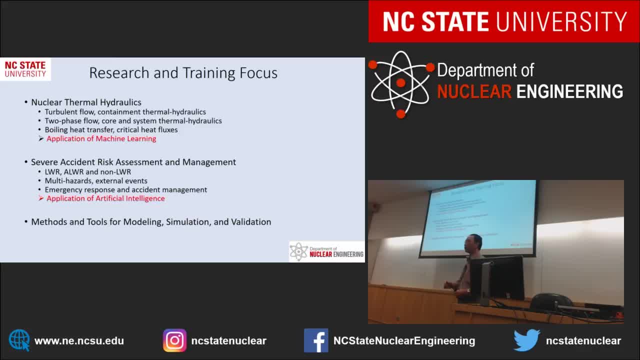 Basically my research is very traditional thing but we try to do that in a non-traditional way So those are classical thing. but in red you try to. my students are working on application machine learning to really looking at the from machine learning point of view. 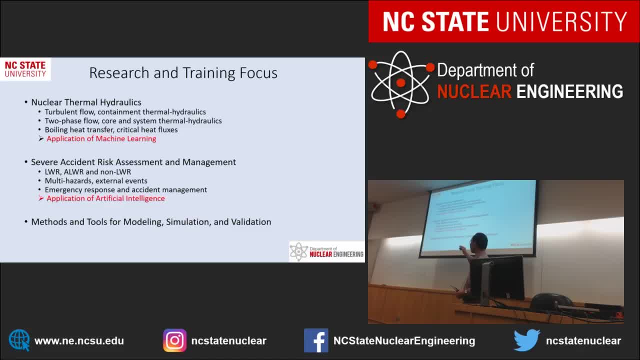 And machine response. we talk about operator and we talk about how to use artificial intelligence to enhance operator function to deal with emergency response. So basically traditional thing, but I've tried approaching that in a different way. And, of course, everybody talking about modeling, simulation and validation. 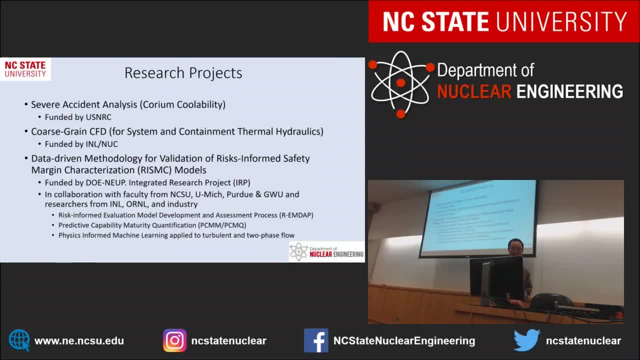 That's something I'm working on. This is a typical project that we currently current project. we have severe accident analysis funded by USNRC, funded by INL, We have an integrated research project on validation funded by DOE And we're working with faculty from NC State for our MOVA, for the Bullard NOPE, with the. 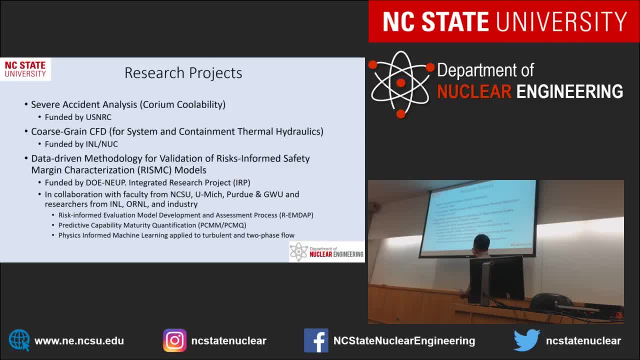 Michigan, Purdue and researchers from National Lab and INDUX-C. Really, the question here is that how do we know that your code is mature for the purpose? Because many times you do safety analysis, safety analysis. you need a prediction. 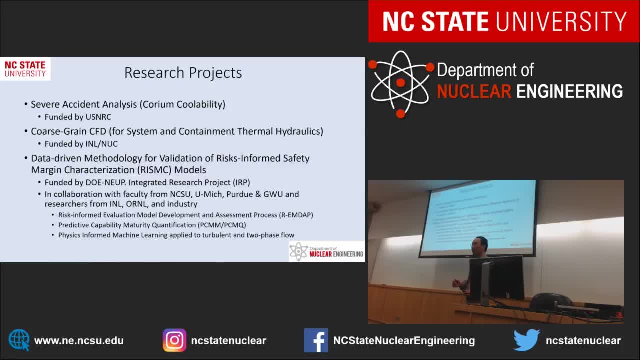 You need a prediction, meaning that you need to use a computer code to do that. And how do you know that the computer code actually is valid? You can have validation for laminar flow for 20 cases, but you apply that for two-blend. 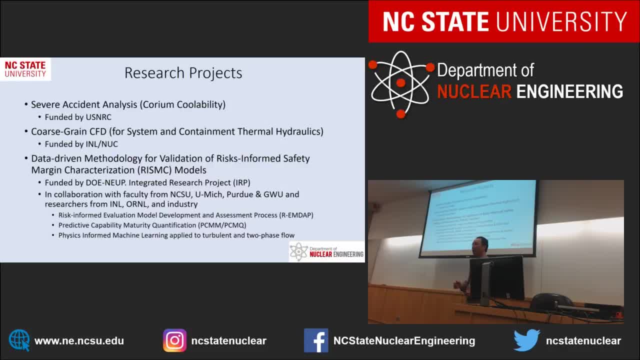 flow, then you are not having any luck to make convincing. It's very difficult. Thank you, Yes, and I see that you are having a valid code. So the question is how to really make sure that the code that you are using is mature. 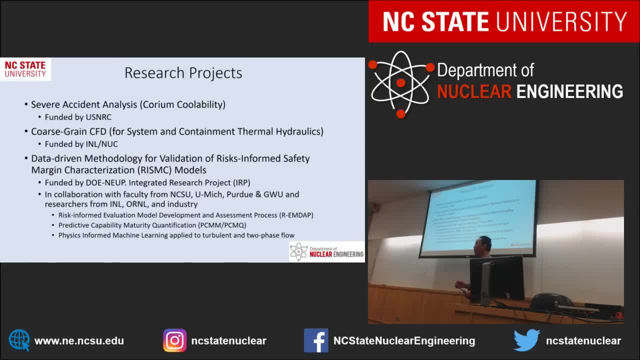 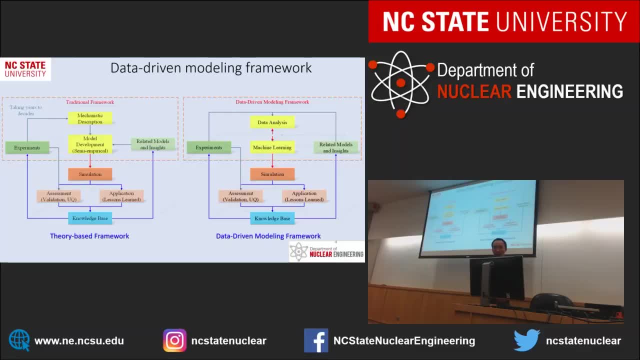 for the intended application. So basically it's related to decision-making. So that is something, This thing we are moving. we are in line by the classical way, like this classical way that you do experiment: take four or five years to design an experiment. four or five. 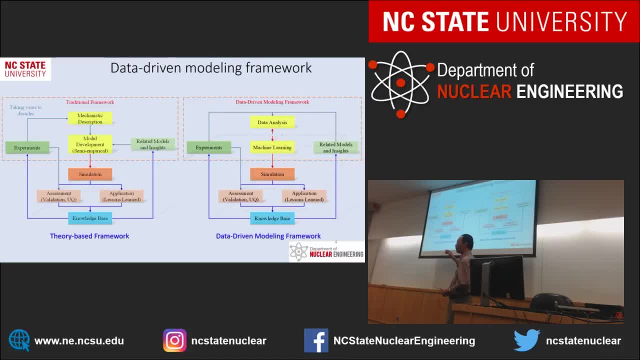 years to really execute an experiment, Get a student to work on that, through three generation of students to really work on getting a model. So basically we go from taking years to decades to really make a mechanism, understanding mechanism, develop a model, and then we apply that for simulation and assessing that and 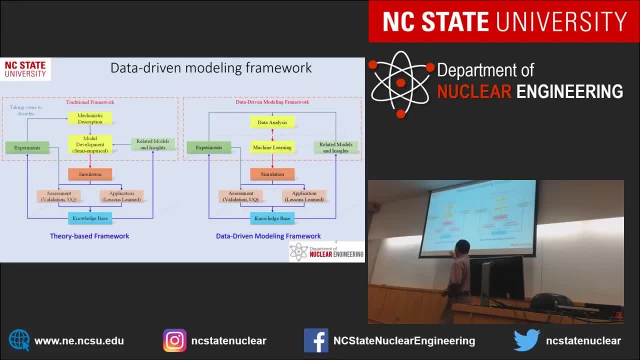 application and improve the knowledge base. That's something we think very dearly for the theory base. Theory base is modern-based framework And it likes to say that if researcher, a graduate student, play a very important role in experiment execution, Designing experiment- and then do processing data and develop model. 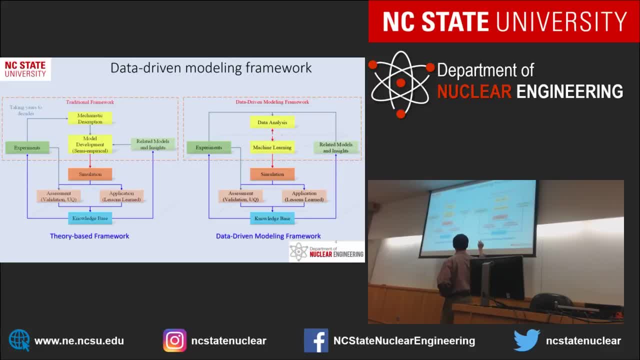 But now the new framework coming in here, the one we are pursuing, the experiment coming out. we have a 3D data high resolution image, a lot of data coming out. You actually not applying data analytics with data. You have data analytics, you have machine learning and machine learning driving data. 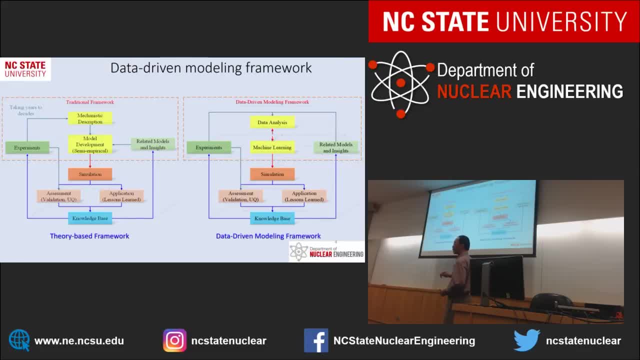 driven modeling framework. In that process You are really processing the data. in a matter of hours and days, instead of years, You have a new experiment. you can be ready to do the processing. So basically the whole process here is trying to eliminate. you eliminate a nuclear engineer. 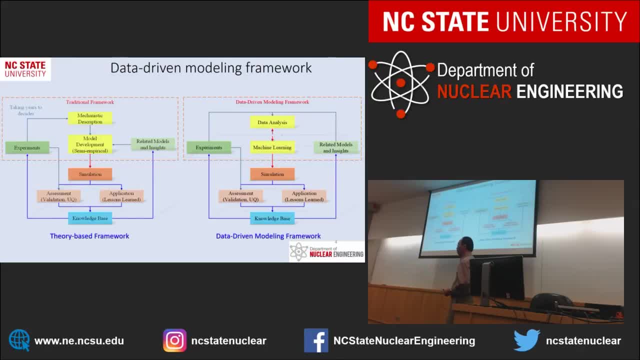 from the process, Because many times our research function has been done by people, but now we analyze the data, But now we are talking about machine learning to bring in, to enhance the way we are doing research, accelerating the research process a lot. 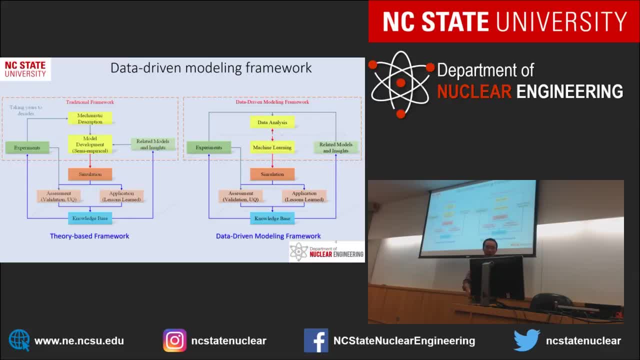 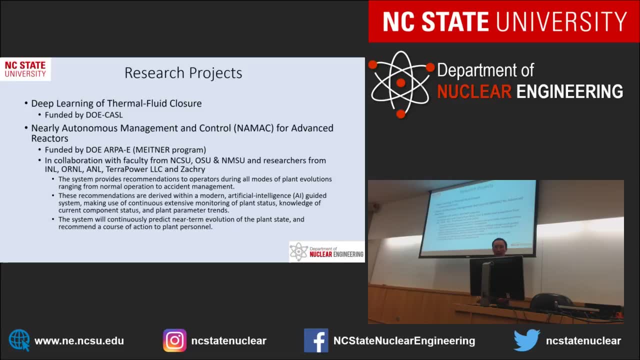 Yeah, That's one part we are working on to do machine learning to. We have a new project funded by APA-E. APA is advanced research project And also it's collaboration with APA and other faculty in the National Lab. So the idea here is that the idea of the project here is that you know that a nuclear 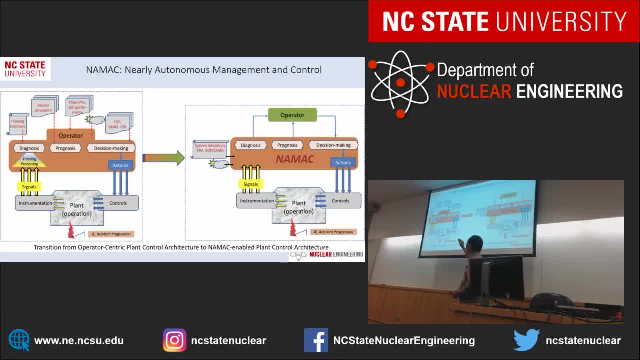 power plant. Of course, The operator plays a very important role. We have to train the operator Based on safety analysis, based on simulator training, and then the emergency response. they have to diagnose the situation, make a prognosis and then make a decision-making. 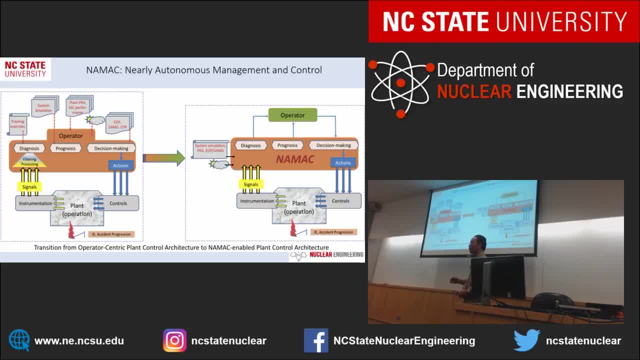 We put a lot of pressure on the operator and that's why 90% of the time they make mistakes And error, error. human error is an immense source of causing an interesting event in a nuclear power plant. So the question here is: how do we help the operator? 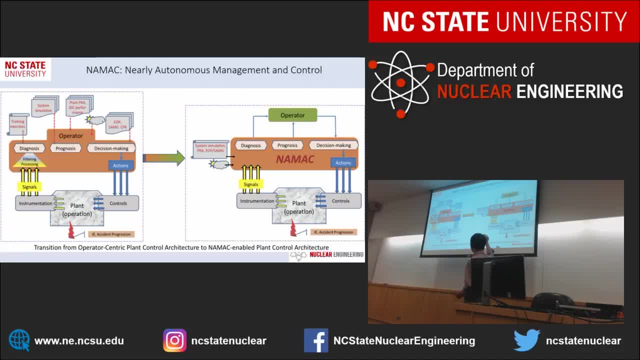 So basically the new system here is that we are putting diagnosis, prognosis and decision-making into artificial intelligence. So artificial intelligence can actually, instead of really looking at four, three or four instruments, a computer can look at 100 signal channels and then do processing. 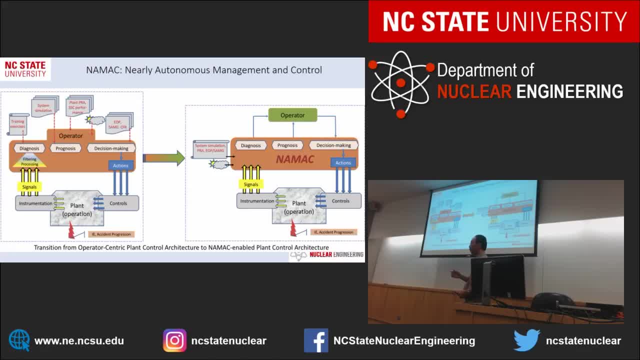 and then give you after training. it can give you operator a way to make run a plan, put a plan in a safe space. So this is something we are working on now: that really putting diagnosis and prognosis and decision-making into a system that allows you to help the operator. 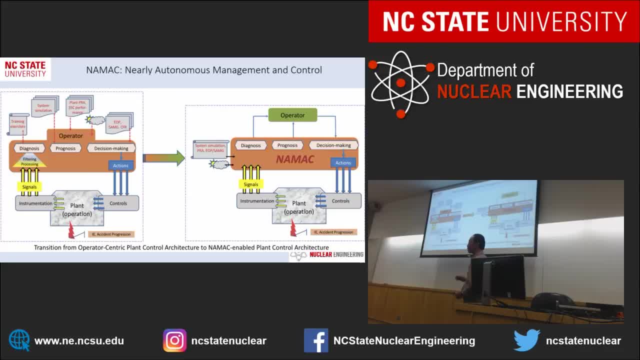 focusing on the way he needs to focus, Put pressure. you understand the operator under accident condition, a very hard time, under high stress condition, under uncertainty, and they are prone to make mistakes, They make the wrong decision. So the question here is that the first part. 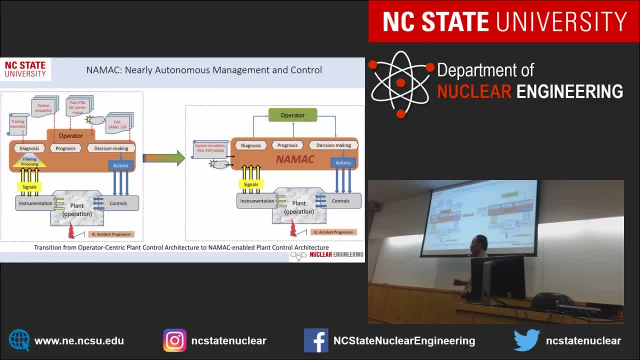 we are trying to help researcher to accelerate the research and in this part we try to use machine learning and artificial intelligence to help operator to run the plan, especially under emergency condition. So very traditional thing, but hopefully bringing a new life based on machine learning and artificial intelligence. 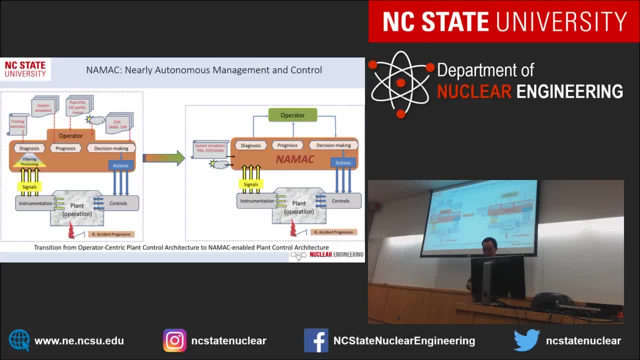 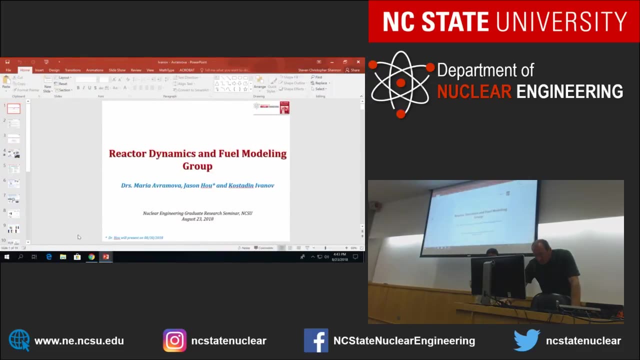 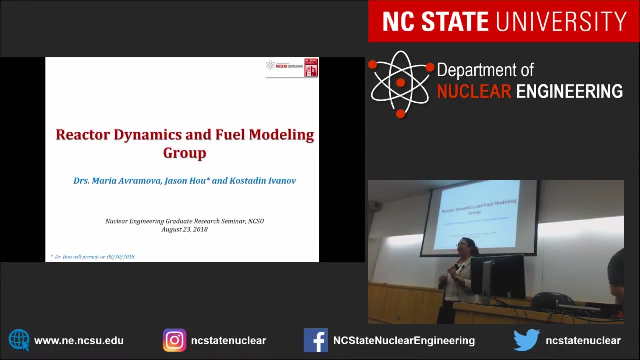 Any questions? I think so. Okay, so I'll try to speak fast and I'll talk about reactor dynamic and fuel modeling group. Okay, We are three faculties: myself, Dr Ivanov and Jason Hu. Jason is in Idaho right now, so he'll present next week. 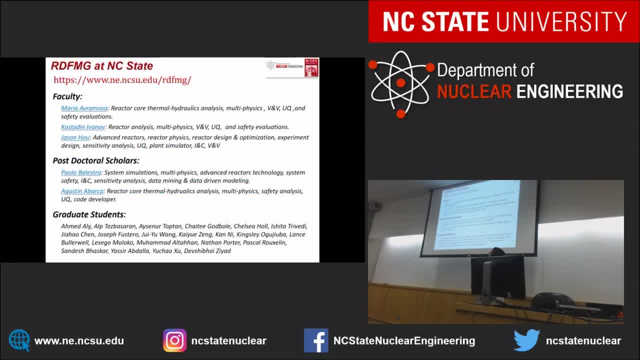 Okay, let me go as quick as possible, So you see our areas. I'm mostly in reactor, thermo-hydraulics, Dr Ivanov is in reactor physics, Jason reactor physics- advanced reactor as well, And we all do multi-physics: uncertainty analysis, sensitivity, validation, verification. 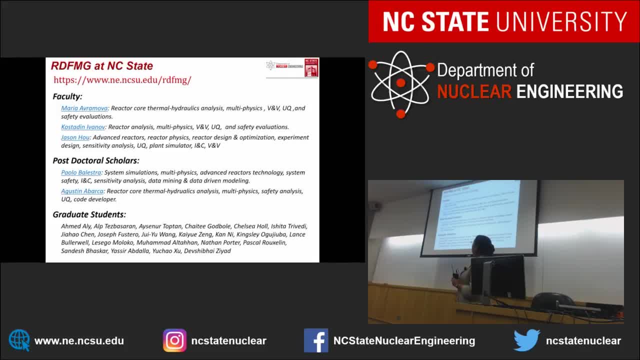 We have two post-doctoral scholars, Paolo and Augustine. You can see their area of expertise And I couldn't put the pictures of our students. There are 22 currently And thank you all of you, So all the figures that you'll see, it's their work. 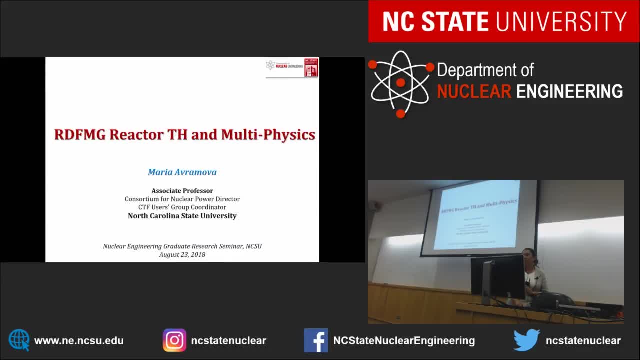 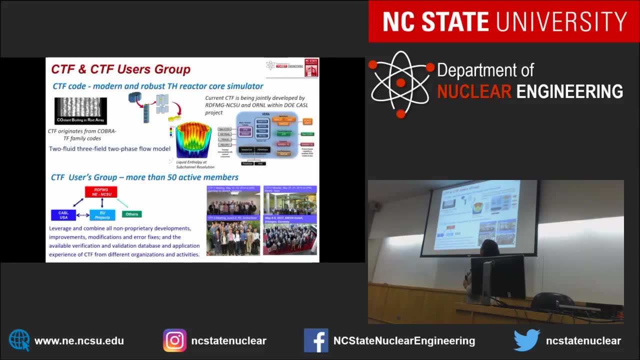 So I'll talk about the TH, thermo-hydraulics and multi-physics in our group And Dr Ivanov. after that we'll cover our international activities. Okay, how many of you have heard about COBRA-TF or CTF? 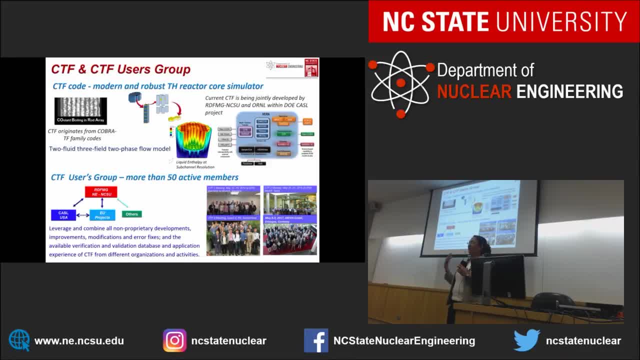 Okay, thank you. So COBRA-TF: it's a very old code And it was developed in Pacific Northwest Library. But CTF it's my baby And I can claim it because this is the code I started working with 17 years ago back in Penn State. 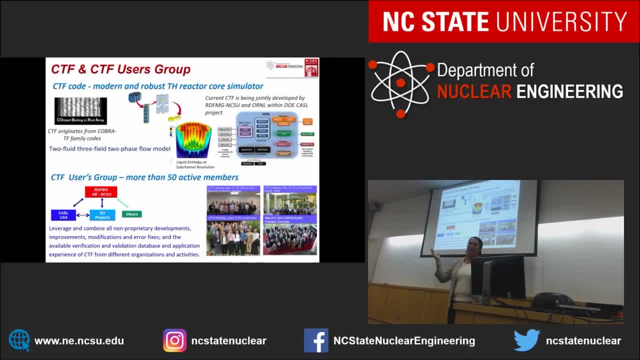 I give it the name, But now it's a grown child And it's out of my control. I even don't know everything which is going on, But I'm very proud of it. So it means coolant boiling in rotary. It's a typical sub-channel code. 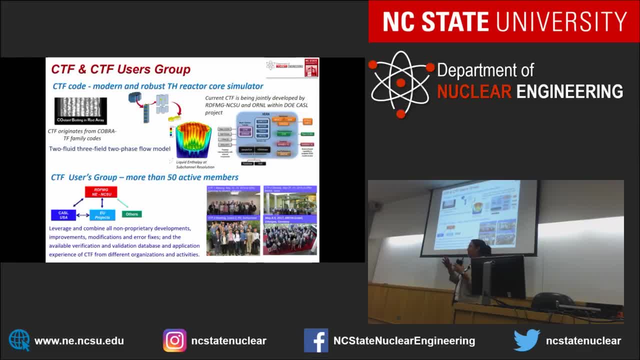 It can give you the temperature and velocity distribution in a sub-channel resolution. Currently we're developing the code jointly with Oak Ridge National Lab within Vera CS, So we have the same code practically. We also have a very large user group, So people around the world- I would say more than 100 organizations- are using it. 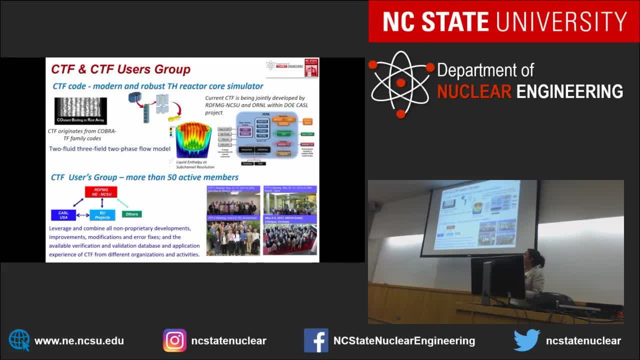 But we have a user group with more than 50 active participants, which means those are people whom we meet every year. We exchange developments and so on, And this is all related to non-proprietary development, something that we easily can share. 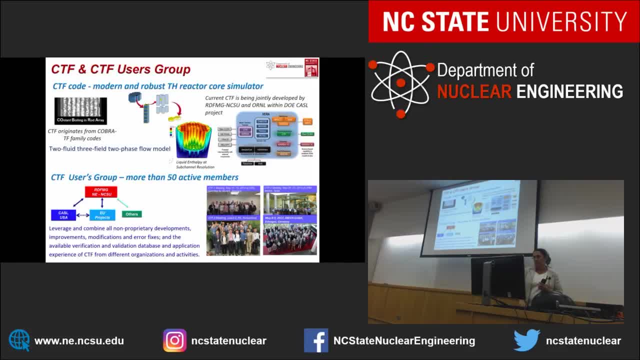 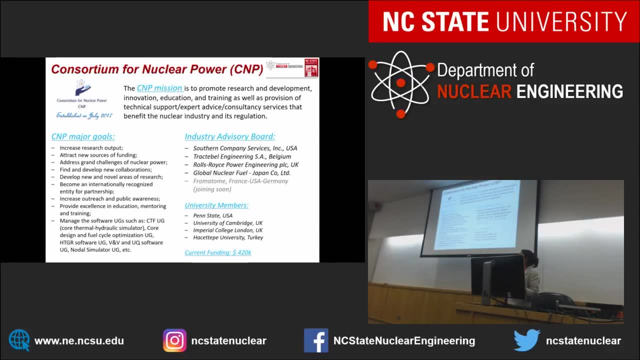 And we started doing that five years ago. We have already four workshops: User group printing. the last one was in Italy this summer. I'll just show some examples of CTF later on, But the other major activities I'm involved in, I'm in our group. 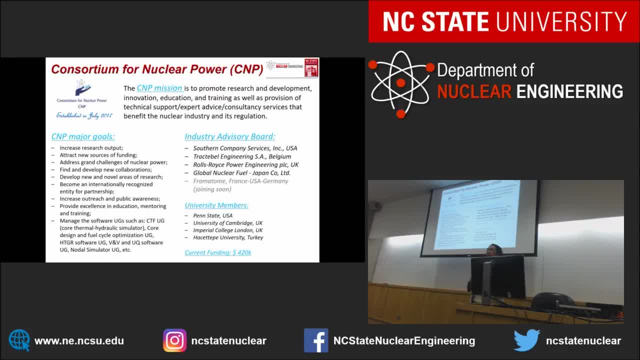 is the Consortium for Nuclear Power which we established last year in June. We hope that we'll go faster, But we're taking baby steps. You see, we have our advisory board. actually It's the industry board. It's Southern Tractebel Belgium, Rolls-Royce Global Nuclear. 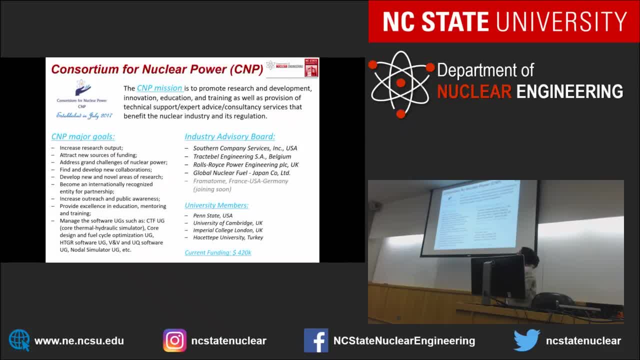 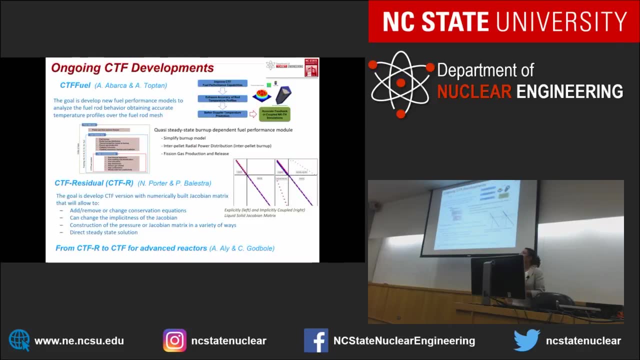 Framatome are just joining And we have a few universities added into. The idea is just to help the industry to progress in advance according to the regulations. So what we are currently doing in CTF- practically I would say we have three major streams- 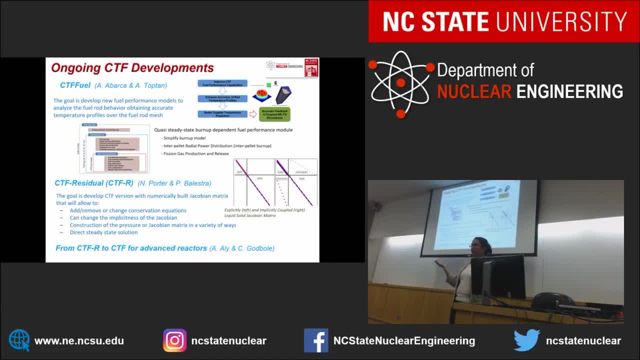 In our groups- I'm not talking about Kassel, because over there there are much more developments- CTF, Fuel- this is something which Agustin Barka, our postdoc, and Aishanur Toptan are doing. They are taking two different paths. 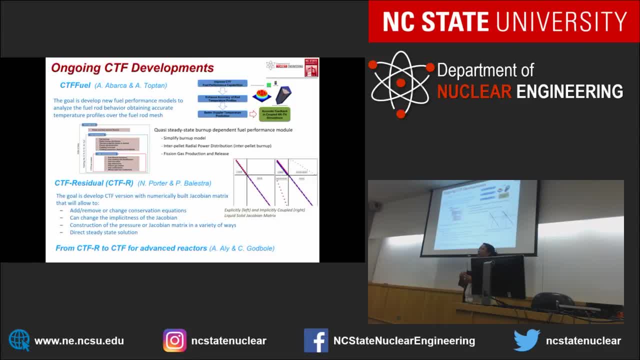 Aishanur is more on the fundamental things. Agustin is working on a near-term project or issues helping with the industry. We really want to have a fuel road model in CTF which will be giving very precise prediction of the Doppler temperature for multi-physics calculations. 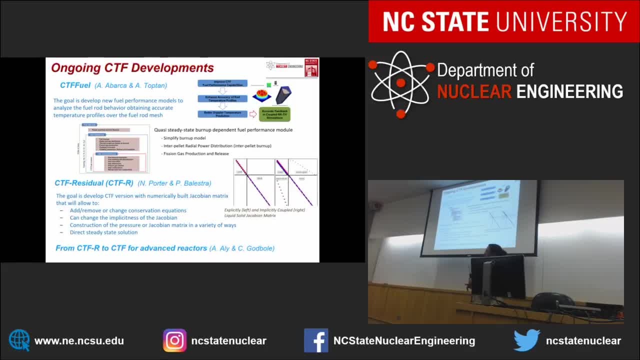 And what the code is missing is a simple burn-up model, interpellet power distribution and better gas-gap conductance model. Now, something which is really new is what Nathan is doing. Paolo is helping him. It's the residual formulation of Cobra-TF. 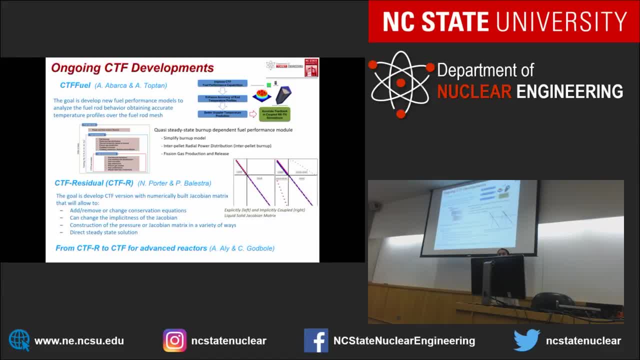 which, once he has it, will be able to switch from different types of equations: number of equations, single-phase, photo-phase, whatever you want, And we may use semi-implicit, implicit, fully-implicit, explicit method of solution. 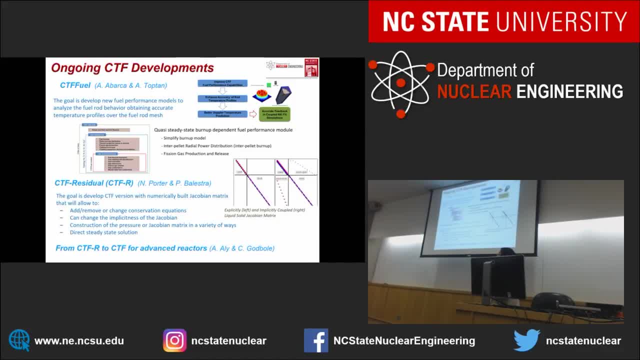 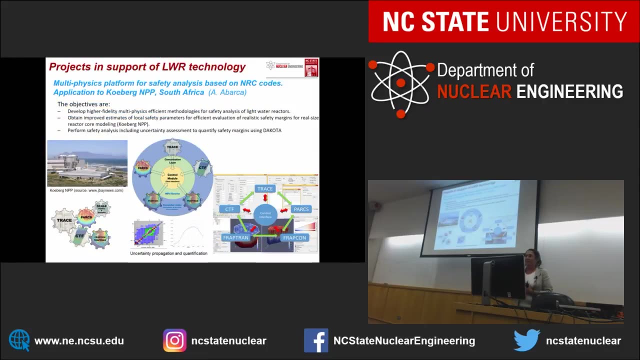 Huge flexibility And that will allow you to go for advanced reactors, and Ahmed and JT are working on that easily. So I'm really going fast, Just want to stay in time Now. but Dr Khawari said that his traditional or his group 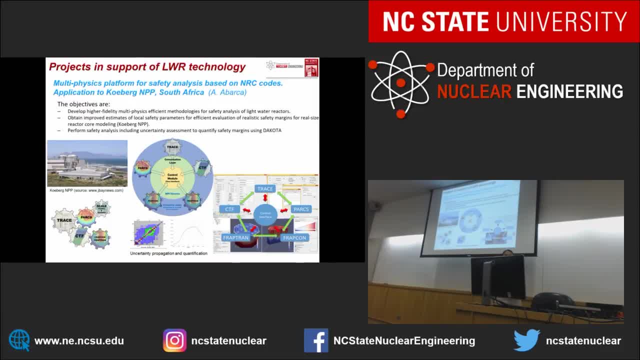 I think we're even ultra-traditional, but we are still trying to support the existing reactor flats light-water reactors. One international project we just started is with Nuclear Regulatory Board of South Africa. They are trying to develop the same approach for regulation as the one in US. 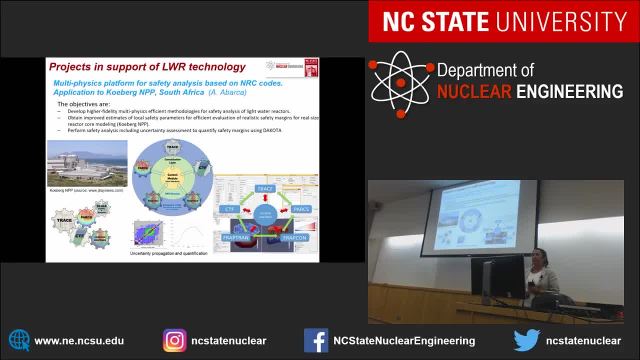 So they are building this system. You see, it's based mostly on NRC codes As trace parts, But we FRAPTRAN, FRAPCON, adding CTF. but we will have also to perform some uncertainty analysis, sensitivity, adding additional codes, even scale into the picture. 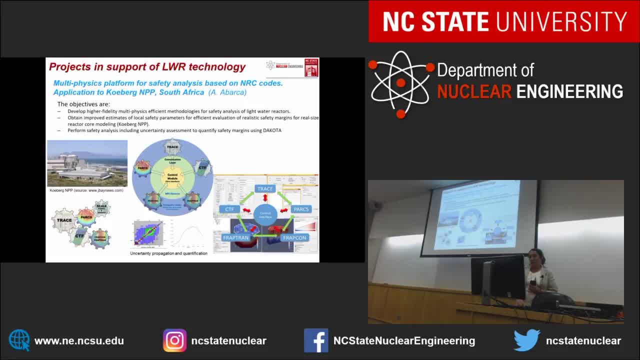 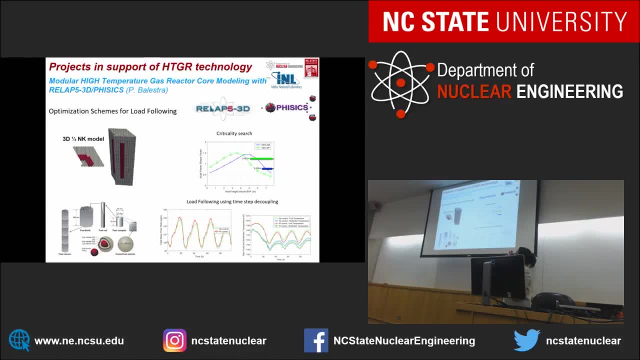 It's something new. we are expecting to graduate students joining us in spring. Now that was related to the light-water reactors. We do some research in high-temperature gas-cooled reactors with Idaho National Lab And that was actually part of one of the senior design course last year. 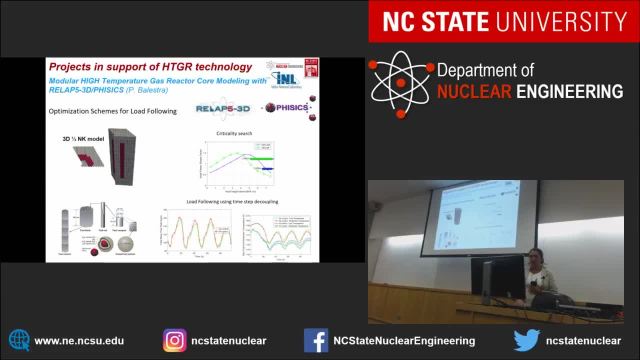 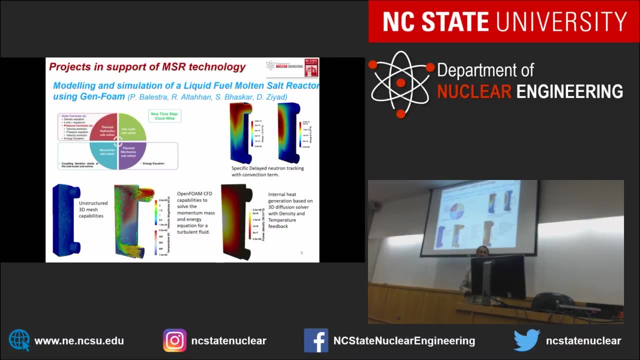 But we are working more on it continuing. We have Paolo De and Pascal, who is right now in Idaho, But he will be back soon. Something exciting. So now, out of the traditional, we are moving toward molten-salt reactors. 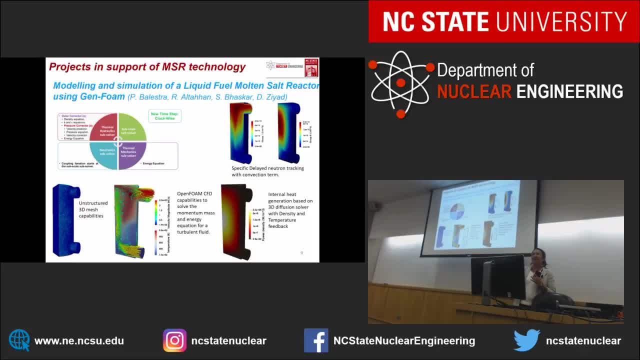 And we have Ramzi, Devshi, Sandesh and Paolo working on that. It's in collaboration with our colleagues in Switzerland and Italy using GENFOAM to model liquid-filled molten-salt reactors. And those are some preliminary results here. 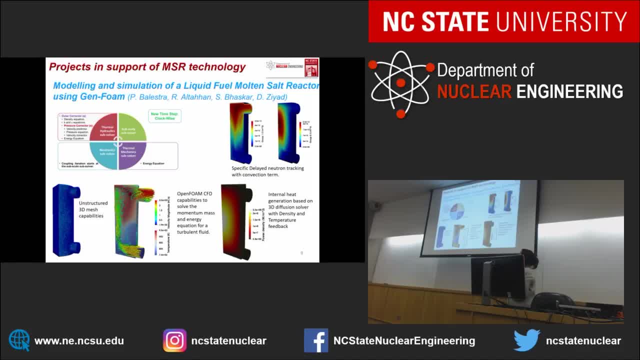 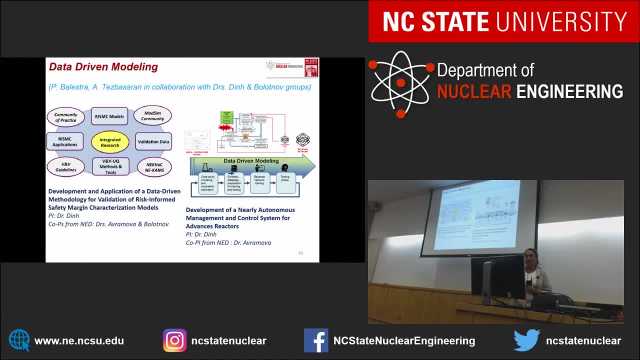 Just imaginary design showing how we can progress with that very interesting design: Data-driven modeling. I'm not going to spend time here. This is which Dr Dean already covered. We I just wanted to give acknowledgment to these students, Alp and Paolo, the postdocs who are involved in these studies. 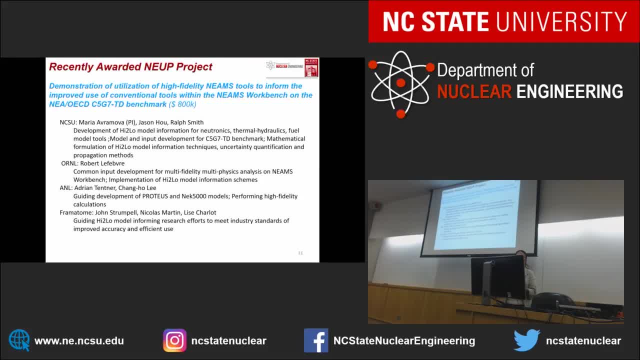 Okay, I have to say that I'm very happy. we just got a new award from NUEP, which is Demonstration of Utilization of High-Fidelity NIMS Tools. to Inform the Improved Use of Conventional Tools within NIMS Workbench. 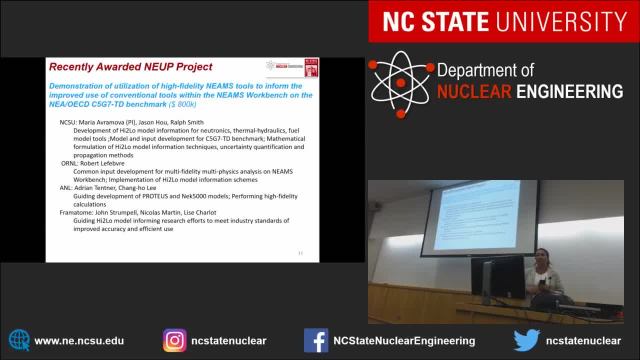 for a benchmark. So it's a long title. I apologize, But you can see the contributors were three professors from NC State: myself, Jason Hu and Ralph Smith for the math department. We have Oak Ridge National Lab and Argonne and Framatome as well in the picture. 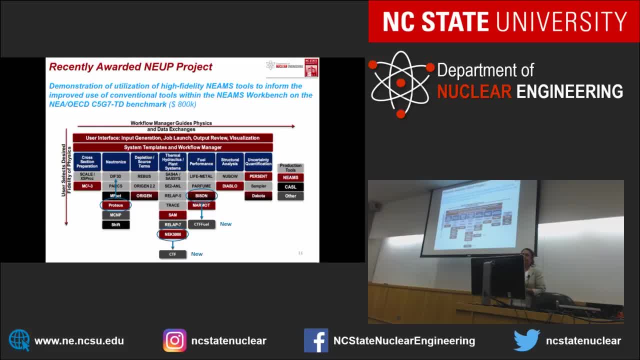 Practically, what we will be trying to do is use high-fidelity codes to inform more fidelity and speed up the calculation. improve the calculation So linking proteols: Proteols with DIV3D, CTF with NEC5000, and CTF fuel with bison. 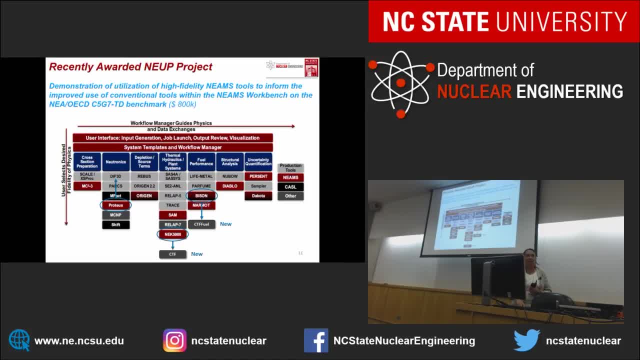 So it's just starting in October- Actually, it hasn't started yet, But this is something new that we will be. We will need some students for, And with that, if you have questions, I am ready to answer. Otherwise we'll pass to Dr Ivanov. 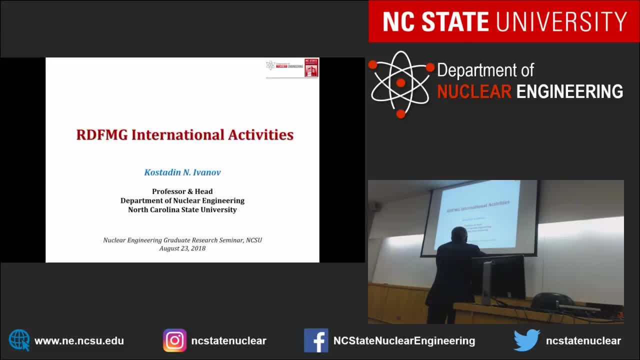 That's not easy, Finally successful. So probably you know me, I am professor in department head in this department And today I am proud of Our professors were almost on time. You know, professors like talking And the most difficult task is to keep them on schedule. 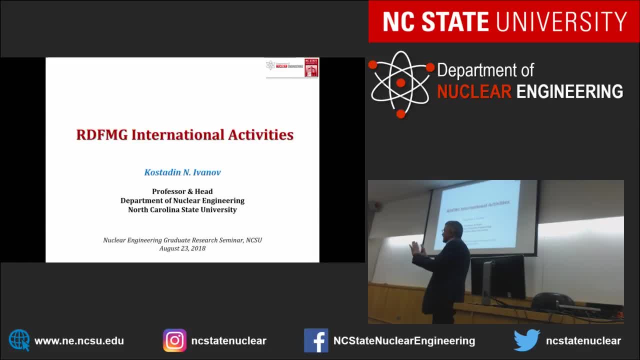 I have to say we have one more after this. Okay, No, no, I'll be quick, So I will talk on my favorite topic. It's international activity, which tells you that I like to travel, But I consider them very important for visibility. 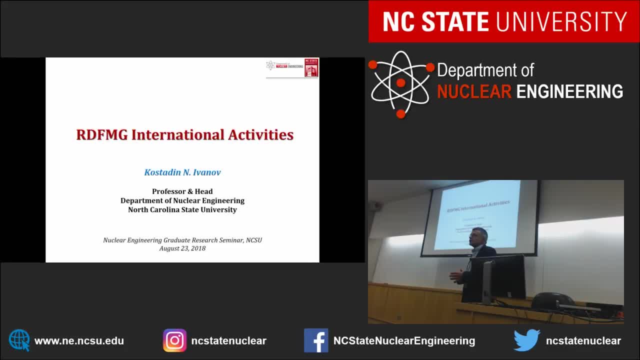 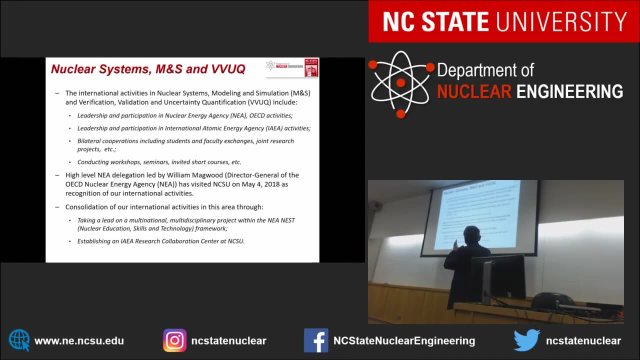 international visibility of the department For recruiting students And also for exposing current students to international environment And working with other groups from other countries. So we I will focus what we do in our group And that's mostly in the area of nuclear system modeling and simulation. 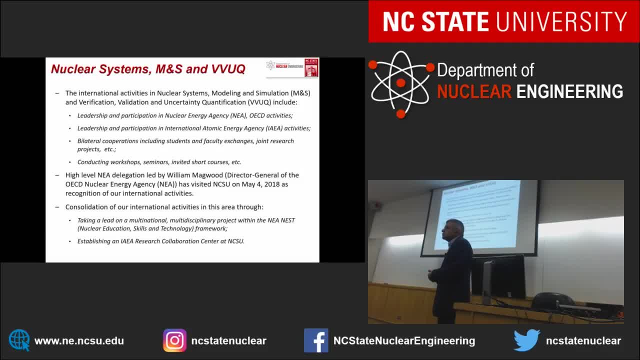 verification, validation and uncertainty quantification, And we do this through leadership and participation in different agencies. Do you know how many agencies in nuclear energy there is in the world? The answer is on the slides. Two are the most important Nuclear energy agency and international atomic energy agency. 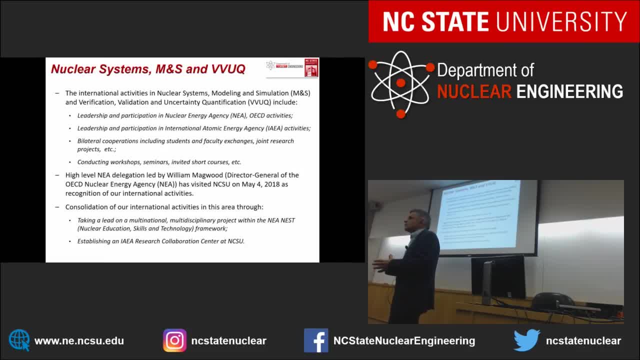 So they support a lot of research activities And many of our faculty are involved- Professor Rudin, Professor Havari and others- And our group actively participate- Not only participate but also lead some of these activities And also we exchange students, faculty. 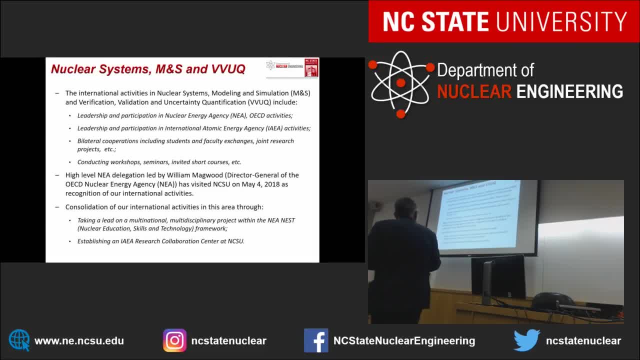 We conduct workshops, seminars And what we're trying to do actually to bring our department even more visible. we're trying to lead a multinational multidisciplinary project within the nuclear energy agency educational and training initiative, which is called Nuclear Education Strategy. 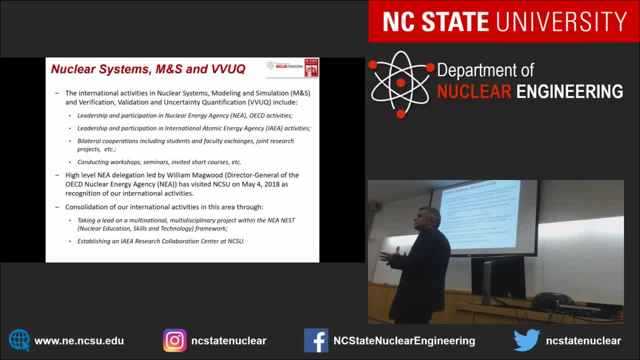 And we're trying to establish a skill and technology framework And we're trying to establish here a project which will be in the area of validation and uncertainty quantification. Similarly, we're trying to establish international atomic energy agency research collaboration center at NC State. on the same topic, 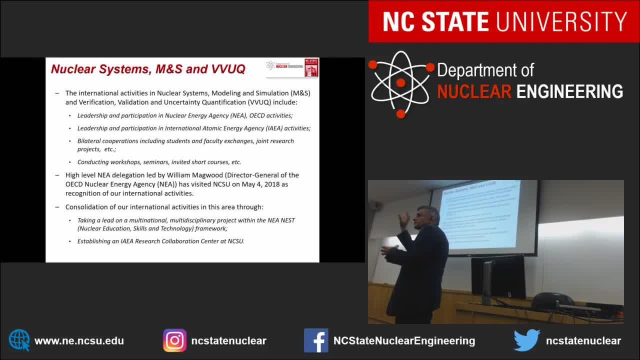 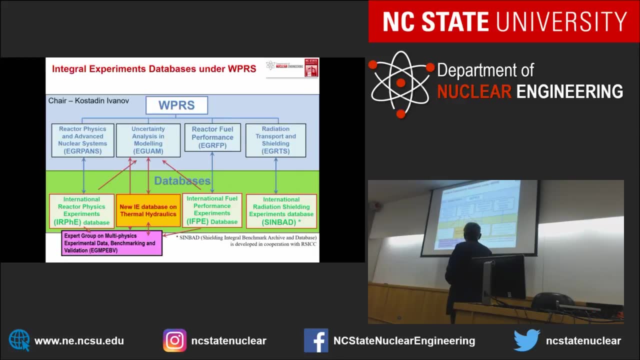 So we're trying to focus, We're trying to put NC State on the international map in the area of competence which we have here, faculty working and recognized. So this is in the nuclear energy agency. I am leading a working party on the reactor systems. 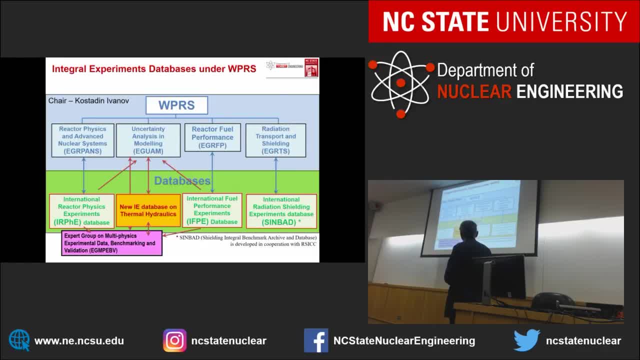 And you can see several expert groups which are involved And mostly their focus: modeling: reactor core including different physics like reactor physics, reactor fuel, radiation, transport, uncertainty analysis and modeling. And next year we're bringing here new expert group which is expert group on core thermohydraulics. 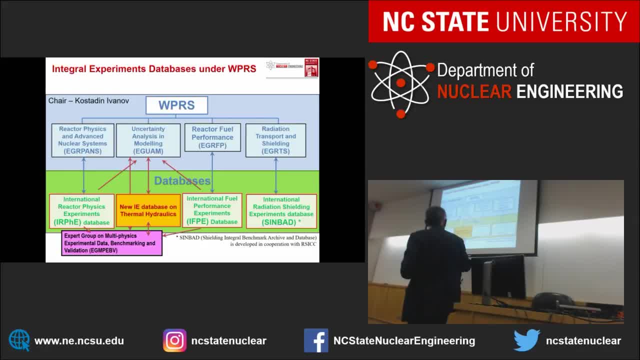 In each of these expert groups is related to experimental databases, And we also participate in expert group which is outside of this working party, but also in nuclear science committee, which is expert group on multi-physics experimental data, benchmarking and validation. 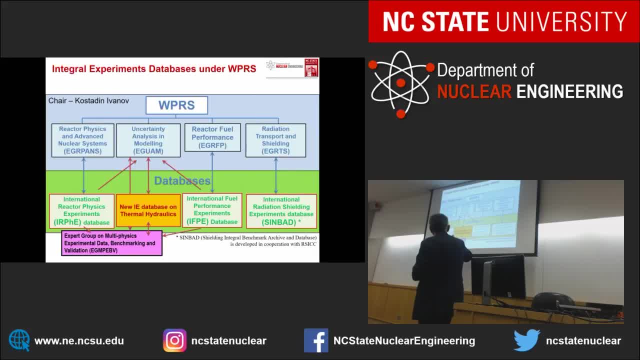 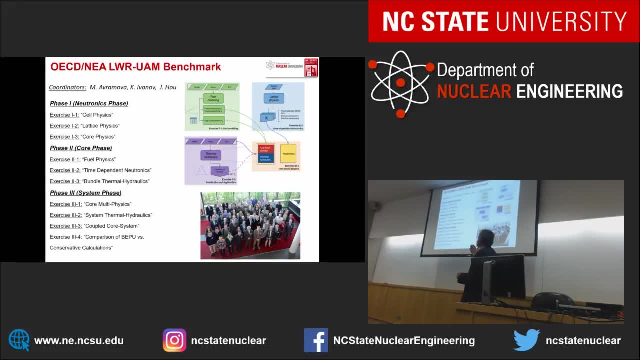 So in leading this activity, we involve our students in different benchmarks and mostly benchmark activities, And one of these is really the light water reactor uncertainty analysis and modeling benchmark. And you know that any simulation involves uncertainties And these are very important when you do your calculations to take into account. 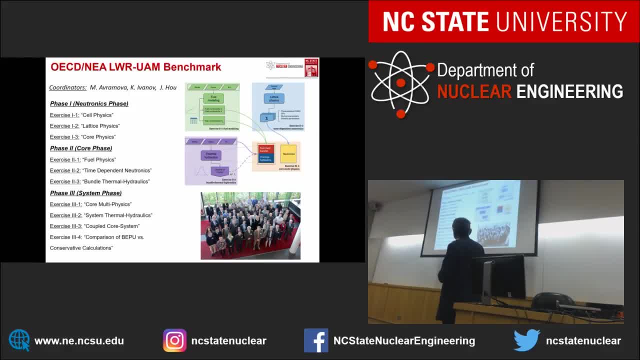 And this is focused really on light water reactors, propagating the uncertainty through different physics and different scale to the final safety margin evaluation. And you can see here in the figure how we combine uncertainty in different physics. And every year we have workshops And next year the workshops will be in Oak Ridge National Lab. 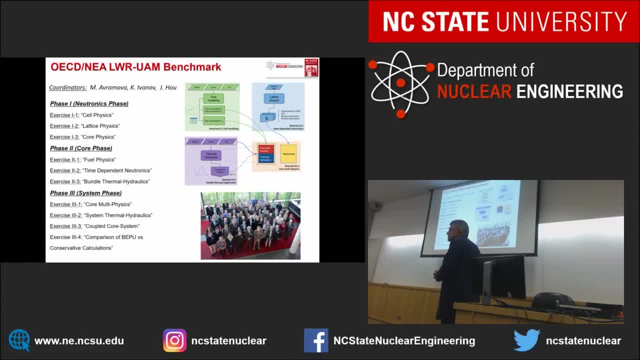 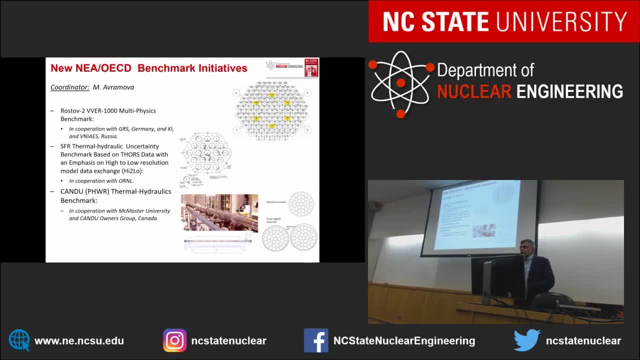 We have more than 70 participants from different countries. It's very important long-term project. We are also coordinating some of the benchmarks in thermohydraulics. Dr Abramov leads several benchmark activities. One is on the VVR-1000.. 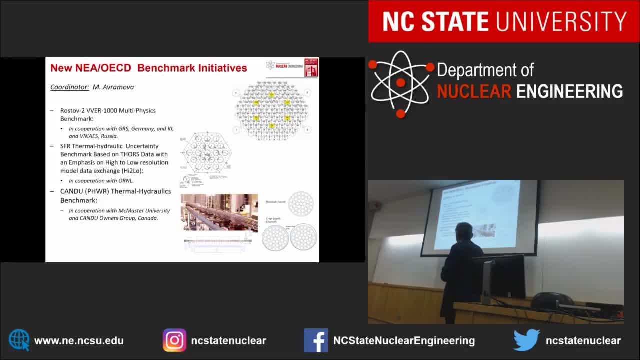 Multi-physics benchmark, which is Rostov-2, is one of the new reactors which start up in Russia with the new fuel, Also sodium-fast reactor thermohydraulic benchmark based on data in Oak Ridge National Lab, And she is involved also in cooperation with McMaster on the CANTU thermohydraulic benchmarks. 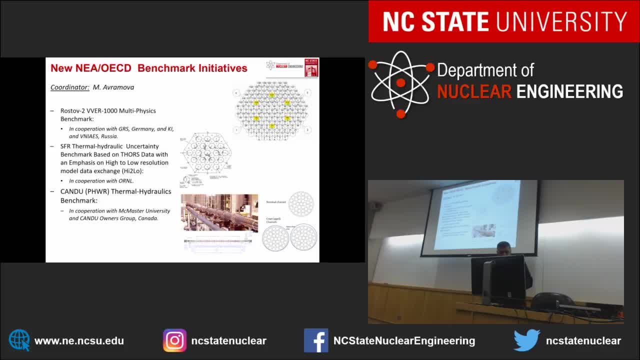 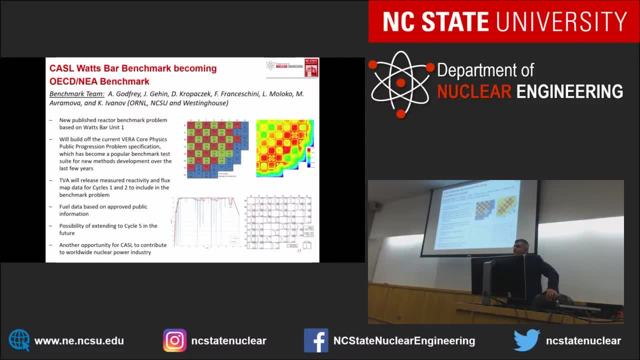 So you can see diversity of activity in different reactors and different benchmarking. We are working with Castle. We are working with Castle not only developing tools but also benchmarking these tools, And we have joined team between Oak Ridge and NC State and Westinghouse. 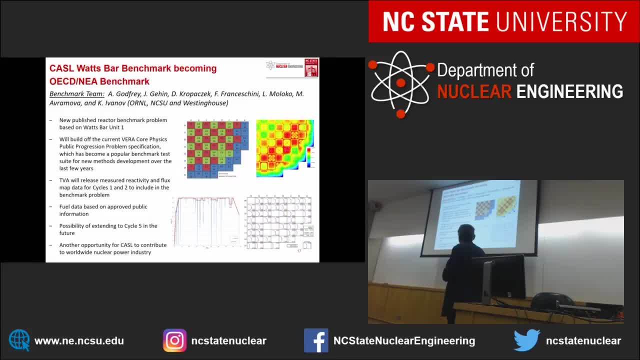 converting the Watts Bar-1 data to OECD Nuclear Energy Agency benchmark. So this is ongoing project And from our side the student working on this is Lesogo Moloko And next again next year in Oak Ridge. we have workshop in May. 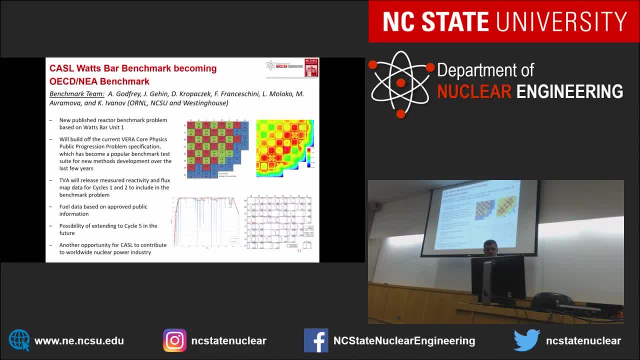 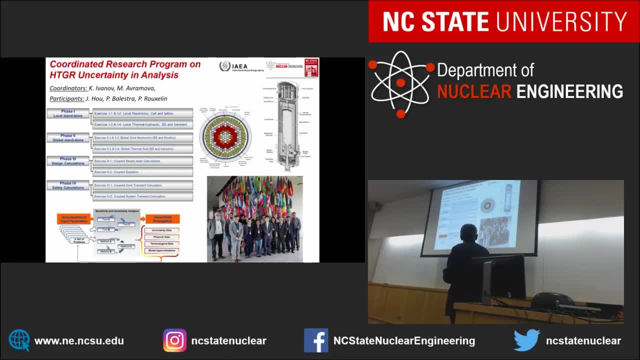 We are starting this benchmark And opening the benchmark to international participation. We have similar program in high-temperature reactor which is in the framework of International Atomic Energy Agency, And we are coordinating this research program And it includes both designs- pebble bed and prismatic. 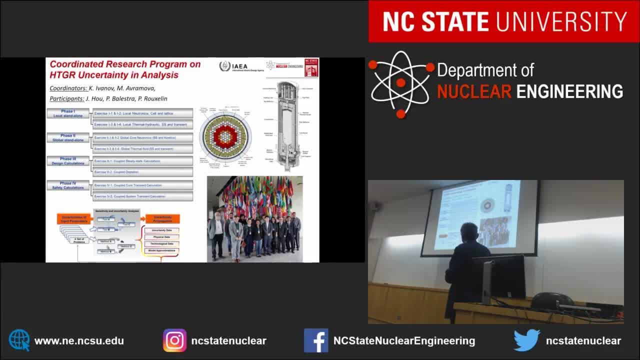 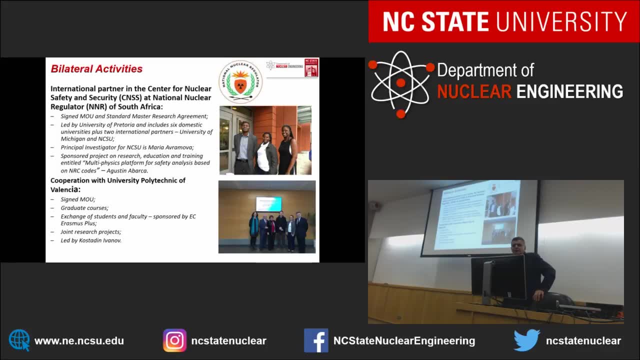 And also similar goals to propagate uncertainty in all the calculations. Finally, some bilateral activities. Maria mentioned about the project with South Africa. It's very important. It's actually it's long-term initiative. They form Center for Excellence And NC State and Michigan are the international partners. 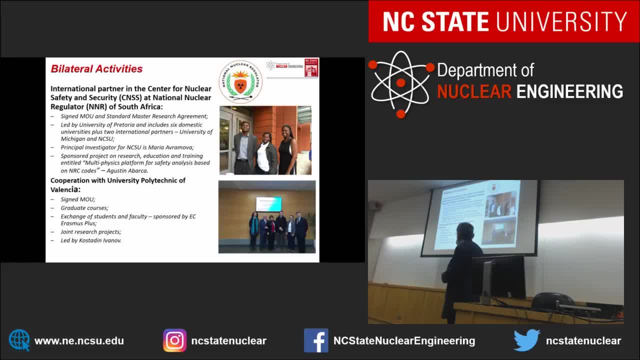 So this is the first project, But then probably will come other projects And we started cooperation with University Polytechnic of Valencia And another project which we are respecting And they are looking for students Is coming PhD project with Fram Atum from Germany. 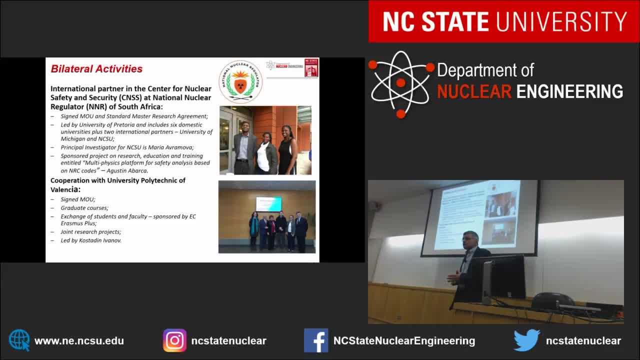 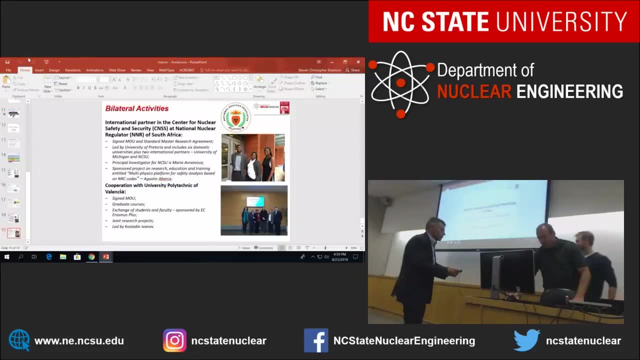 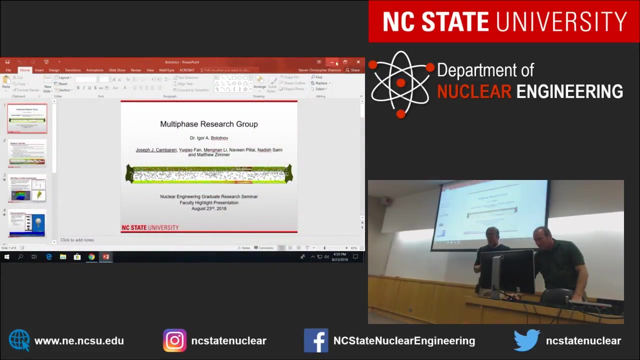 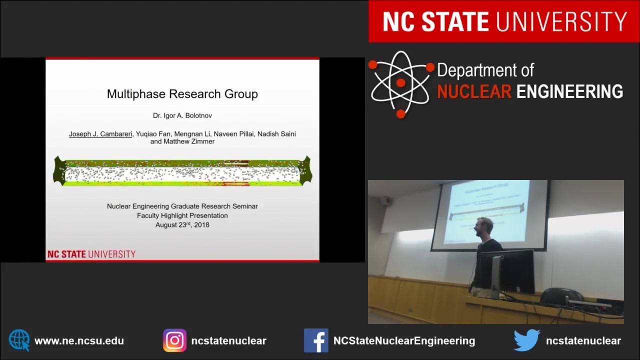 On high-fidelity core simulator with uncertainty propagation. Thank you very much. All right, Hi everyone. I'm not Dr Balanov, But I'm his lucky graduate student that gets to present for him today. My name is Joseph Cambreri. 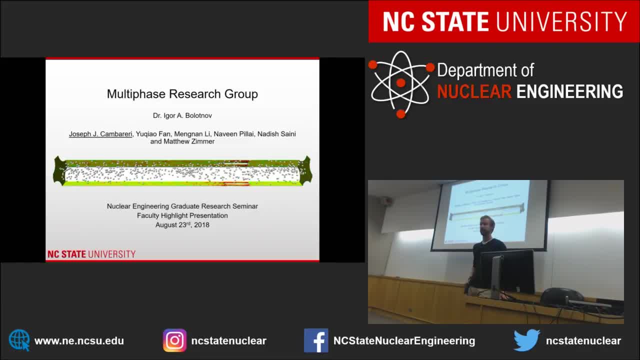 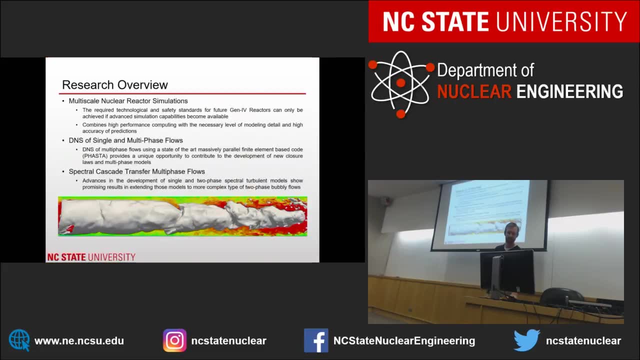 I'm a PhD student in his research group And in our research group we focus on multi-phase research analysis. So bubbly flows, turbulent bubbly flows, two-phase research. So just kind of give a broad overview of our research areas. 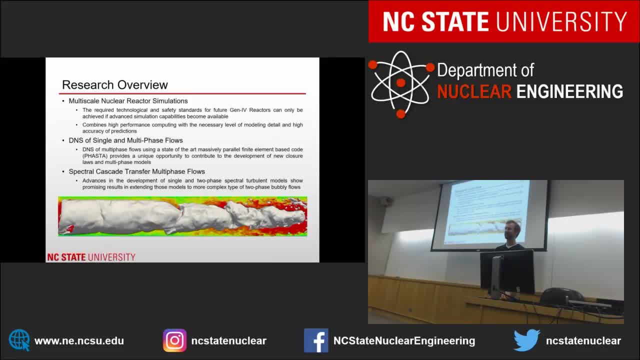 You can break it down into three general sections. I'm going pretty quick Because you know we all want to leave and go home. So first off, we have multi-scale nuclear reactor simulations. So this is looking at basically advancing the development and safety analysis for Gen 4 reactors. 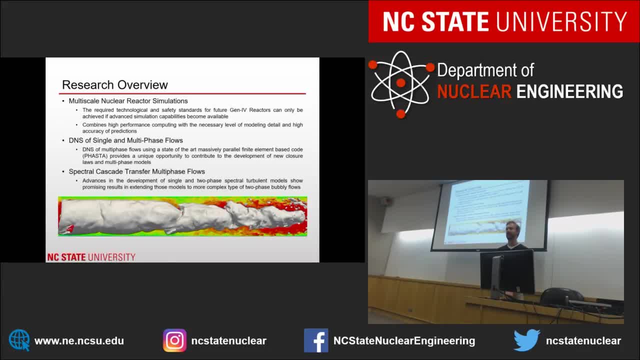 And then combining high-performance computing with the necessary level of modeling detail And high-accuracy of predictions that are needed to develop more advanced closure models for the development of these future reactors. Then there's obviously the data DNS, so direct numerical simulation of single and multi-phase flows. 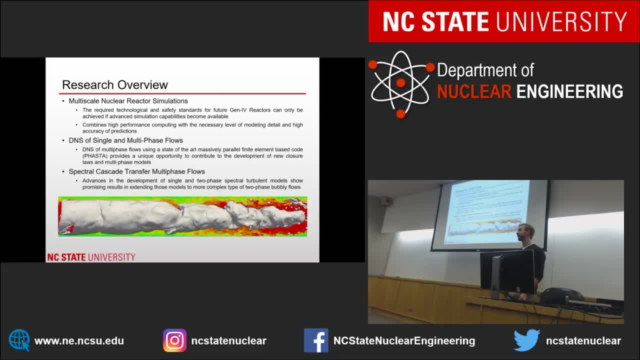 So this is gathering high-quality numerical data for those uses in different development of closure models that may not be, you know, exactly reactor design oriented, But still very relevant in two-phase flows. And then finally, while not a very large aspect anymore, but we're also looking into spectral cascade transfer flows- 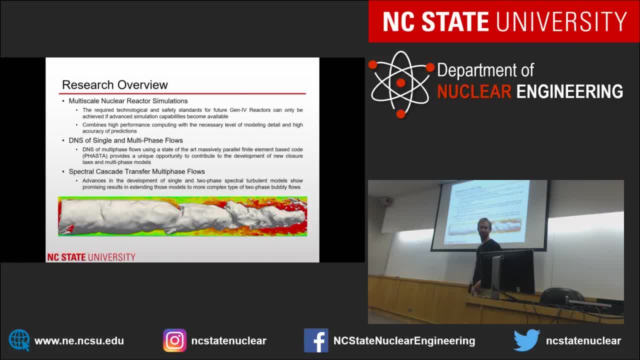 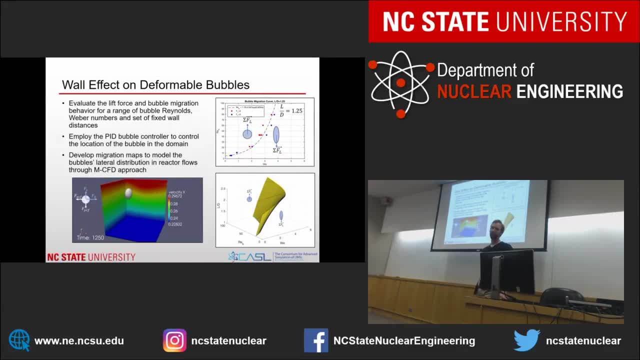 And this is to develop a two-phase spectral turbulent model. So I just have some examples of the work that we're doing. We've looked into the wall effect of deformable bubbles, So this is looking at the specific forces that are acting on bubbles. 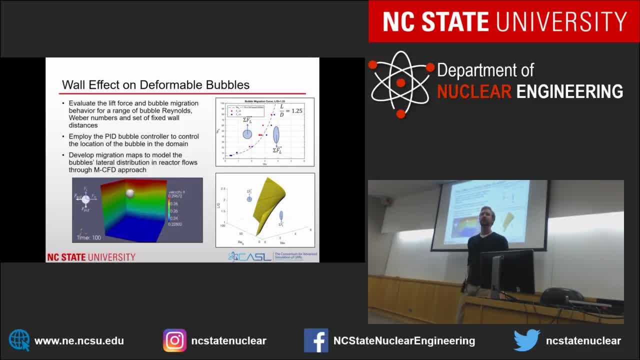 So with our research code FOSTA that we have, we can actually control a bubble's location within the domain And register the forces that are acting upon it, to calculate out some of the you know, drag force, lift force, And by doing this we can create these 2D plots up here. 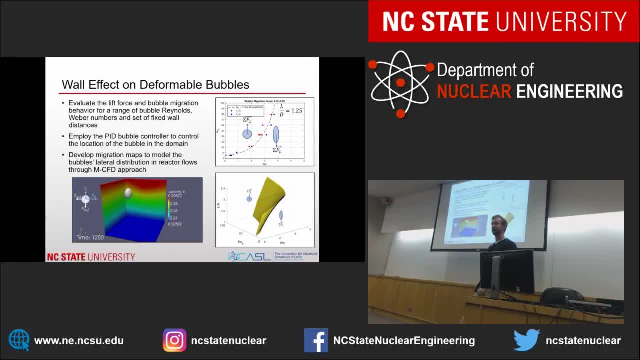 That describe how the lift force develops as you change some of the bubble's parameters And then running these simulations again and again, hundreds of these, We can then create 3D maps that will describe your bubble's behavior Where you are in your domain. 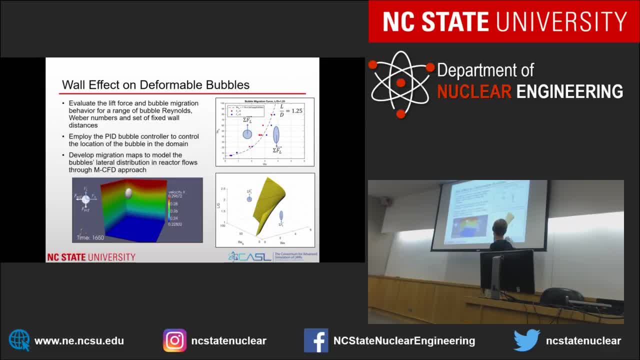 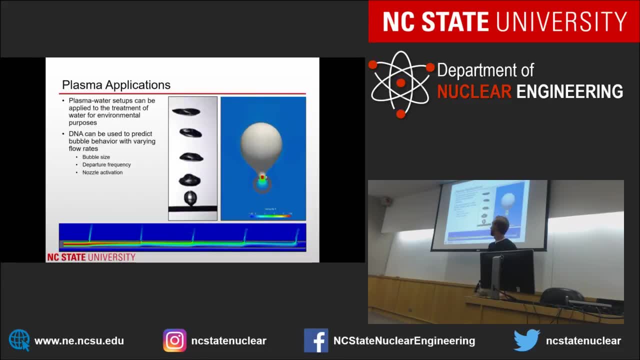 How large your bubble is, Your Reynolds number, Your Weber number Or your dimension list of parameters. So we also have some plasma applications. These have been talked about, So I'll kind of skip through this really quick. Even so, You can see some of the same images that you can see. 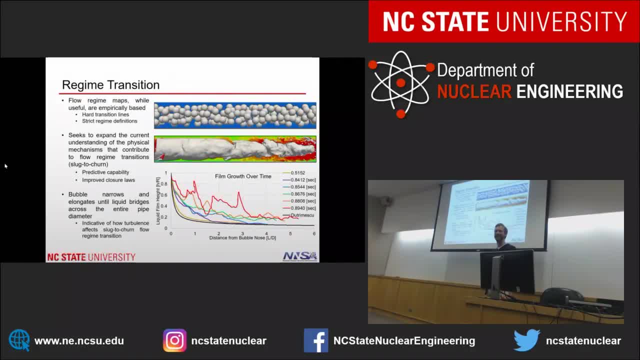 Navin might have doubled up on his emails that he sent out. So some more work that we're looking at is regime transitions. So while these are maps that are empirically based, They're very useful, But they usually have these hard transition lines that are very strict regime definitions. 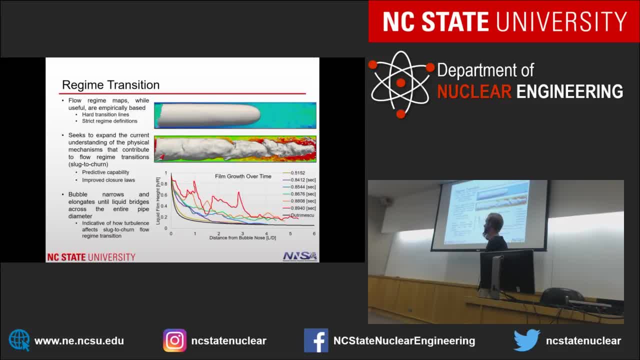 So we're using our codes to actually look into the physics behind some of these regime transitions, So specifically slug flow transitioning into this churn turbulent regime. So we want to improve the predictive capability of our regime maps And then also improve those closure relations. 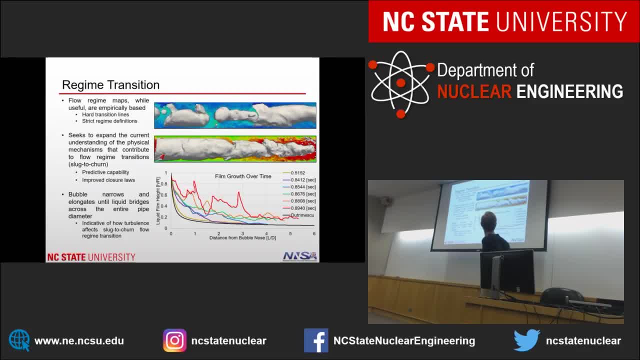 So that we know the physics behind the actual flows we're looking into. So here you can see kind of the development of your Taylor bubbles throughout your domain And then we'll ramp up the pressure gradient that we apply in our simulations And you'll get the development after the slug flow runs through. 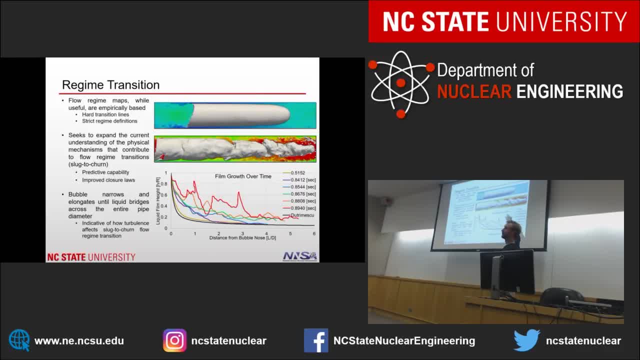 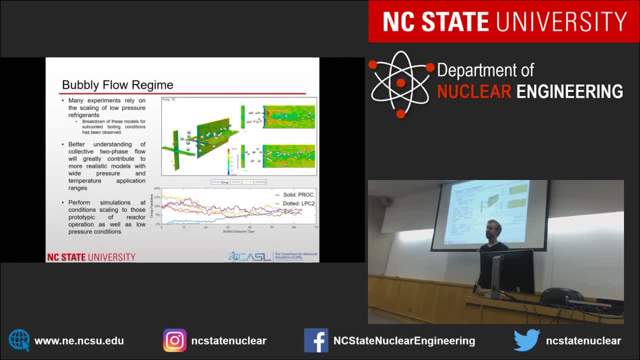 Of this really highly churned, turbulent domain And we can gather statistics from that and analyze them. So we also look into light water reactor or PWR, subchannel simulations. These are all bubbly flows, So we're looking at scaling up to conditions that are typical of reactor operating conditions. 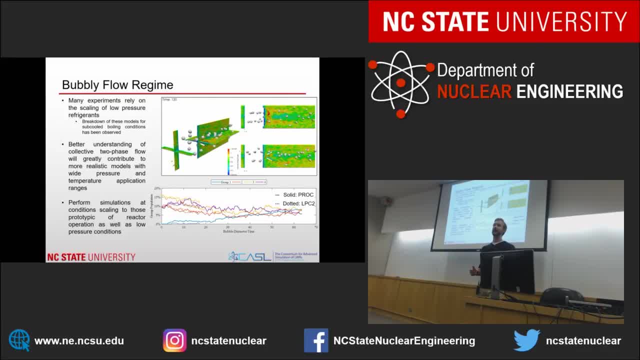 So we're trying to approach those conditions that you would see in a typical reactor, And then we want to get a better understanding of the physics behind them, Of the physics behind the flows, So we can basically improve our closure relations that we have. 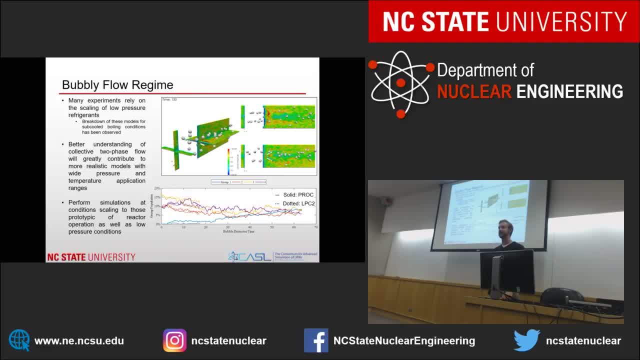 And this is some work that we're doing, Looking into the scaling of low pressure refrigerant experiments Up to these high pressure and temperature conditions. So the breakdown of these models has been observed for subcooled boiling. So we're trying to do some of these numerical investigations. 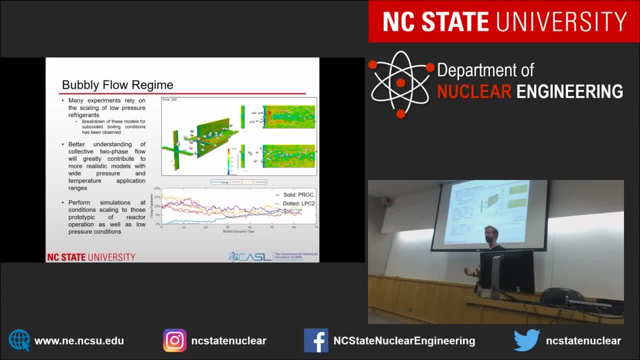 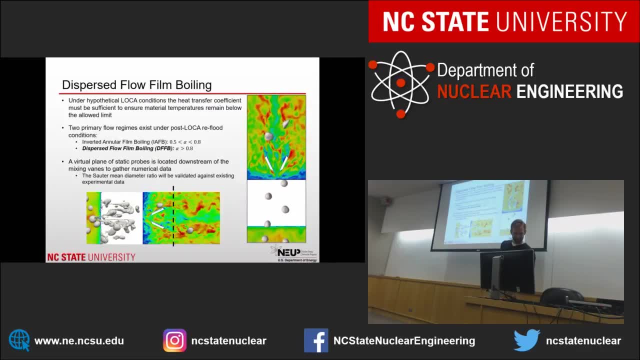 To supplement the experimental data that we do have. For again, I keep reiterating Advanced model development- We also look into more accident scenarios. So when you have a loss of coolant accident Under the reflooding event, You'll typically get two primary flow regimes.